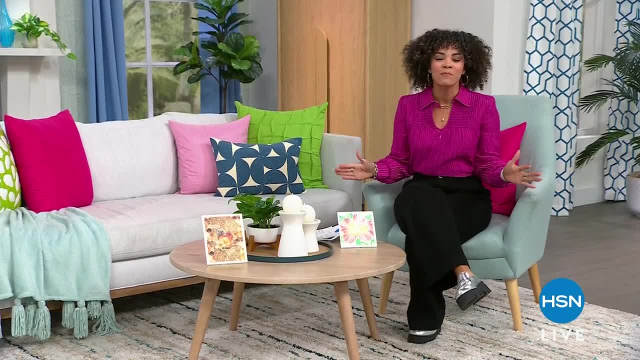 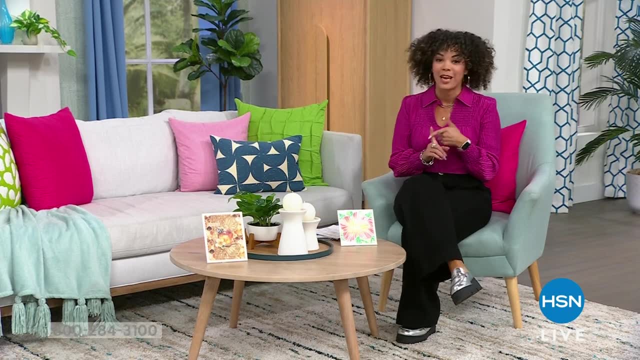 Sale. So everything that you're seeing on air for 24 hours is to help you get those projects done and everything is at a sale price. Okay, coming up a little bit later in the show, I'm really excited about this. Toni will be joining us. She is the one that brings us. 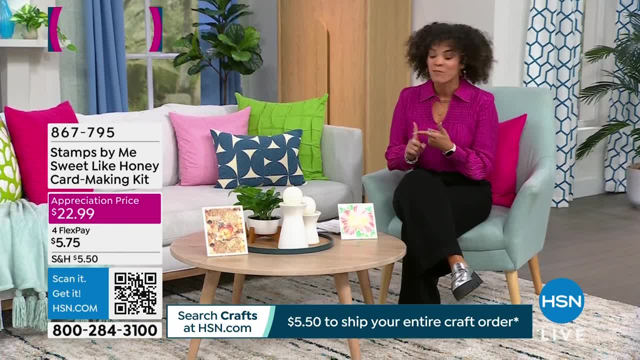 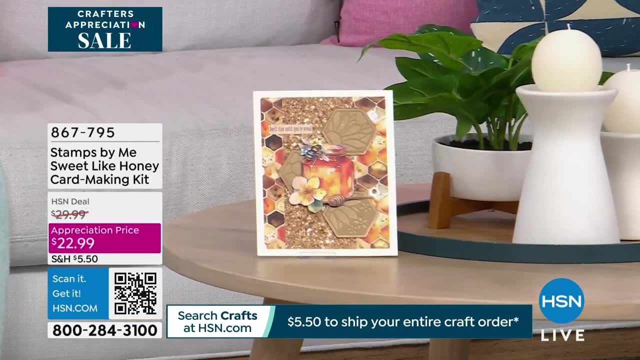 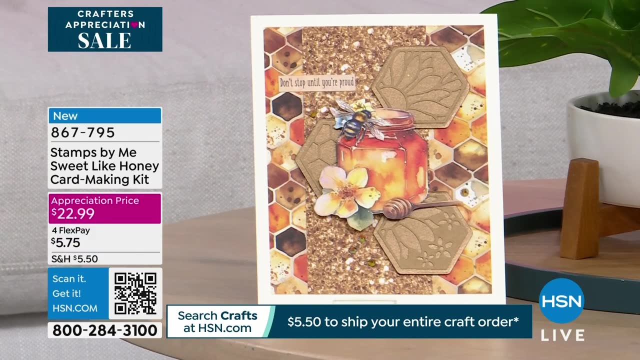 Stamps by Me and this is your Sweet Like Honey card-making kit. So this is an opportunity to really create these visually stunning cards. It's high-quality materials that you're getting, with creative embellishments and with dyes easy to use and even customized. I love the. 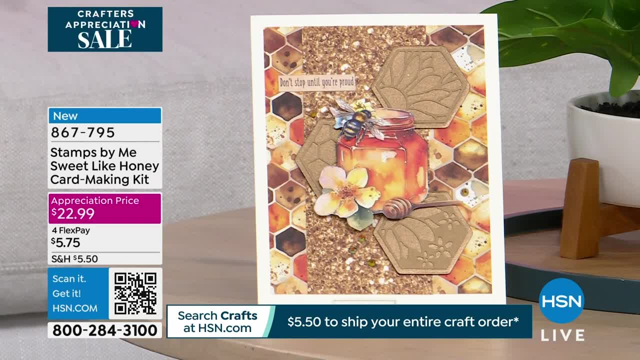 whimsical beauty of the bees that you get with this and the warmth of a flower. So if you're looking for something that's really, really, really, really, really beautiful, this is the card-making kit And, of course, those honeycombs. So that's coming up. 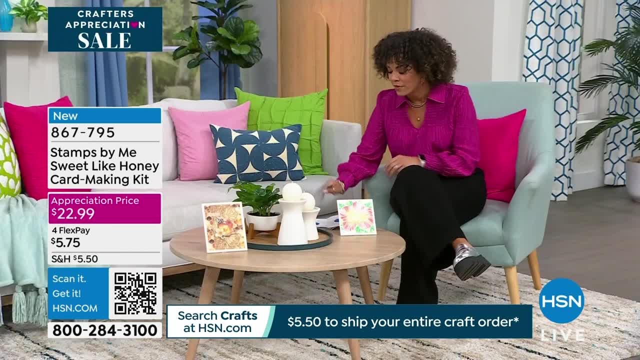 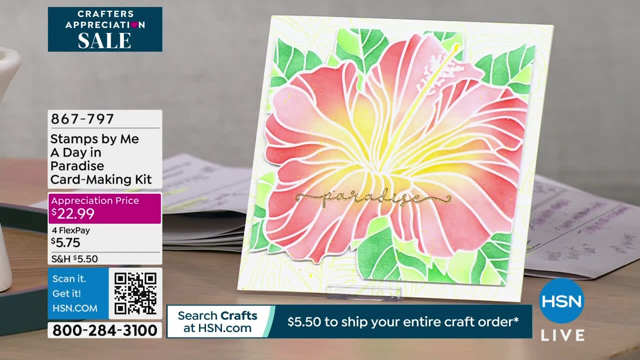 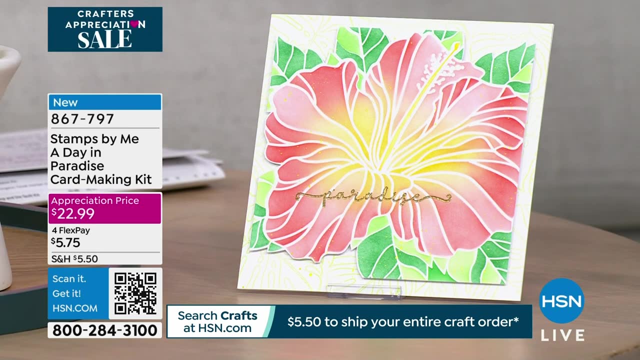 towards the end of the show. 867-795 is the I'm number if you want to shop early, for that, And then also from Stamps by Me is a Day in Paradise. Now talk about beauty that you get with this card-making kit. Beautiful floral designs that you'll be able to make with this. Appreciation price: $22.99.. Here's the thing. Load up your cart today, because your whole cart ships for $5.50.. Now you're probably thinking: well, I don't know, I don't know, I don't know. You're probably like me. You're like, wait a minute, But if I load up my cart and then I check out, am I going to have to pay $5.50 again? No, You can check out already if you already have 10. 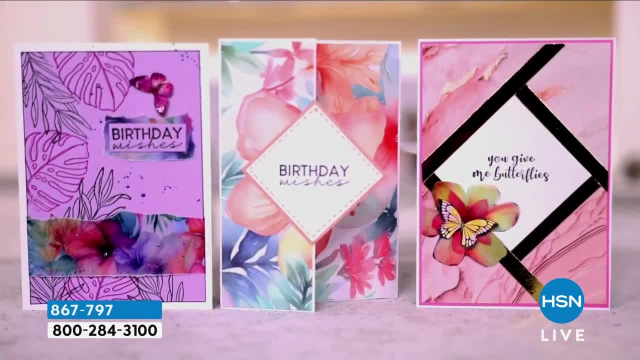 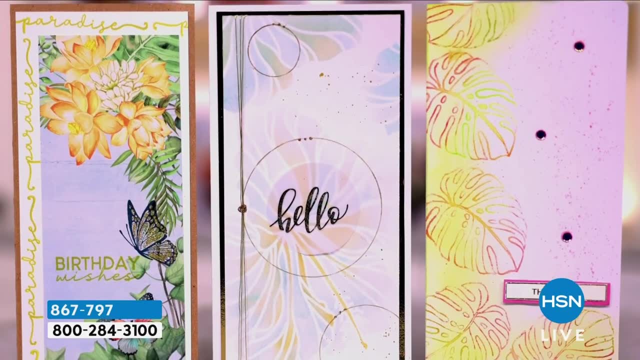 things in your account from Anna Griffin. Check out It's $5.50 shipping Next things that you have. you won't be charged a shipping, So I absolutely love that. You're welcome to dive into that card-making kit that will come at the end of the show from Tony by Stamps by Me. 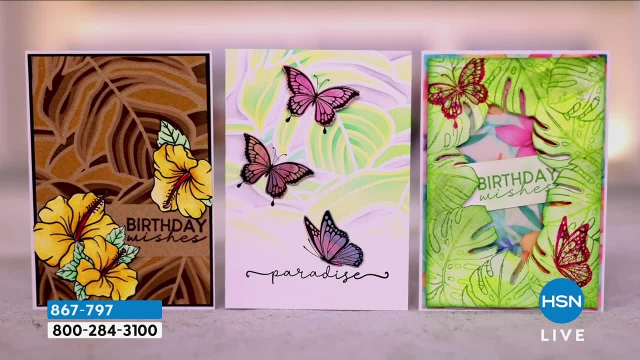 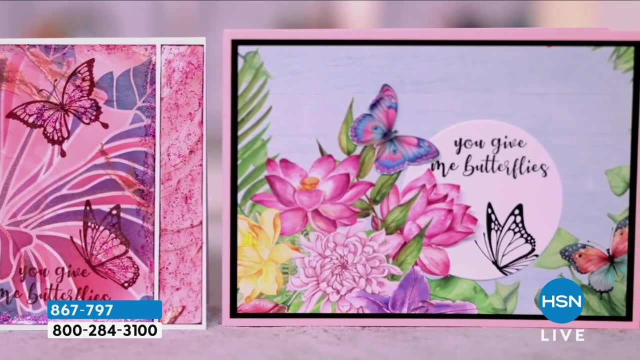 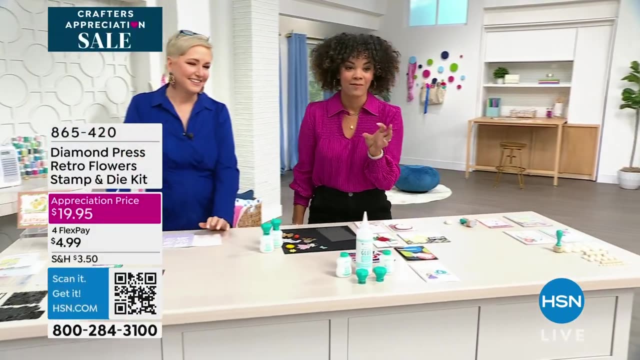 It's 867-797.. Okay, Let's get started. And let's start with something that is so, so fun. It is from Diamond Press, And what you're getting are these Retro Flowers, Stamps and Dyes Kit. Now here's the thing that's really exciting. First off, Beth King- I thought you were. 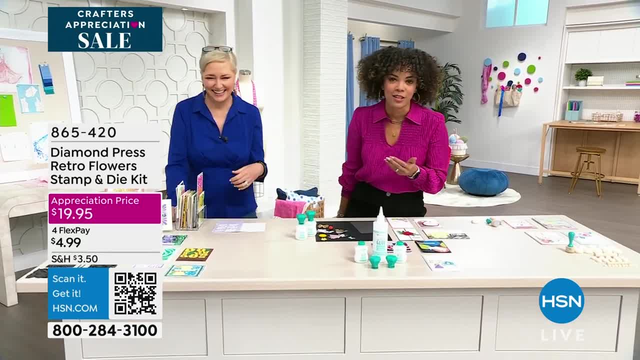 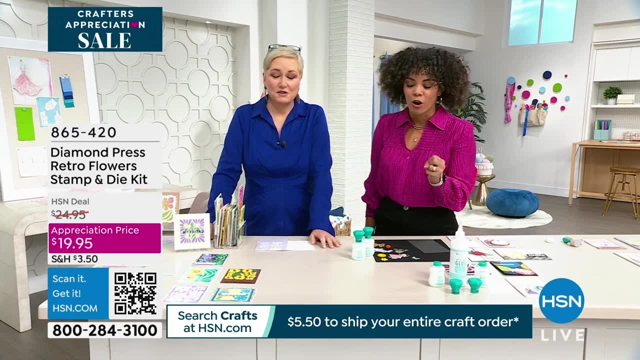 going to say I was doing something that was so fun. Beth Kingston is here with us. She's been in the crafting world for many, many years. has so many tutorials online, been teaching classes across the entire world? You can't escape me. That's what she's saying. No, she makes crafting. 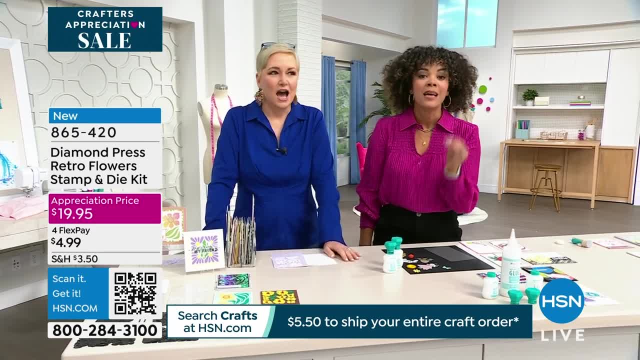 so much fun. But what's great about this is we have so many brand new pieces from Diamond Press that we're featuring, So this one is your Flower Stamp and Dye Kit, So you're going to get the stamps that you need. 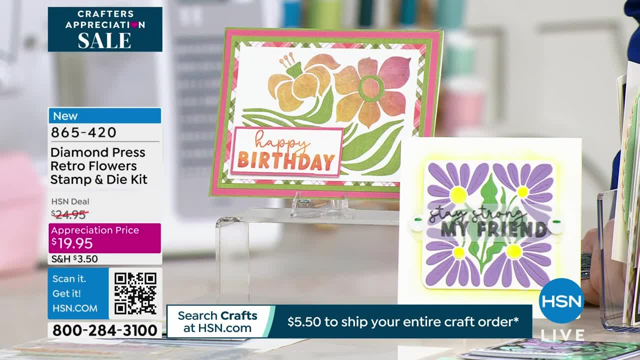 the dyes that you need, the adhesive, all the things to make the cars, the tags, the embellishments, I mean. and then look at the price: $19.95.. I know, but here's the thing. Here's the thing. 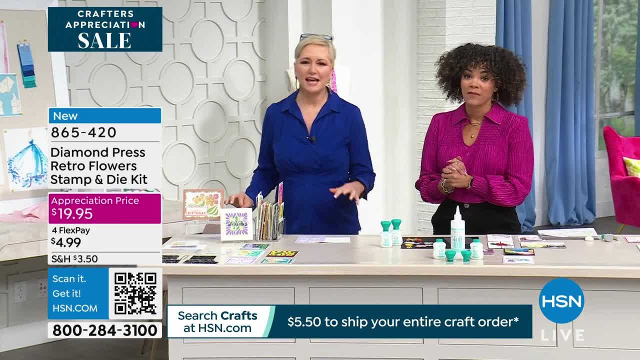 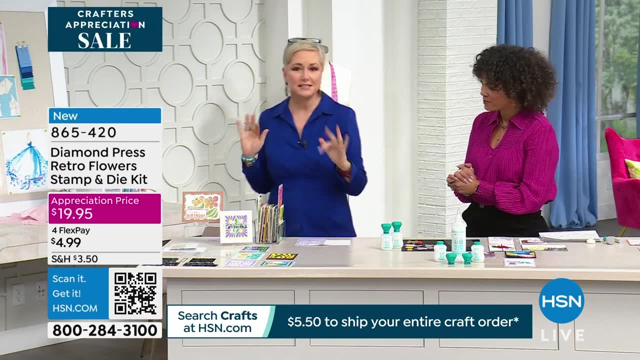 Beth, Only about a thousand. That's it: A thousand of these to go around. This has been very popular. I showed it on Friday during a live, I think, and people just want crazy. So I want to show you initially what you're getting, because this is something that Diamond. 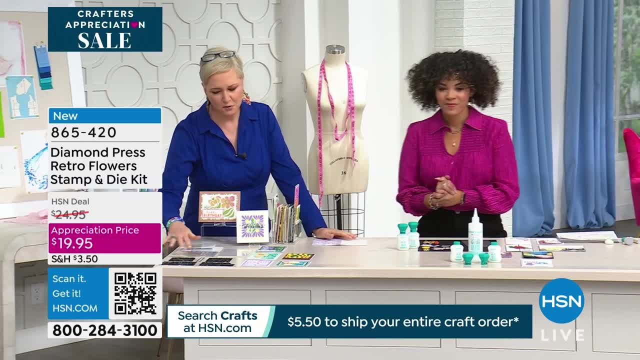 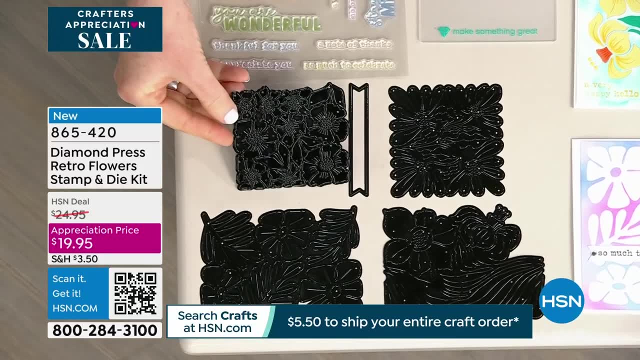 Press has never done before. You might look at these dyes and think: okay, I don't understand what's happening here, Because normally our dyes are like super intricate and they've got little cutouts everywhere. This you can- oh, you guys are so good, Look at it. This you can actually see the entire pattern, and it's one. 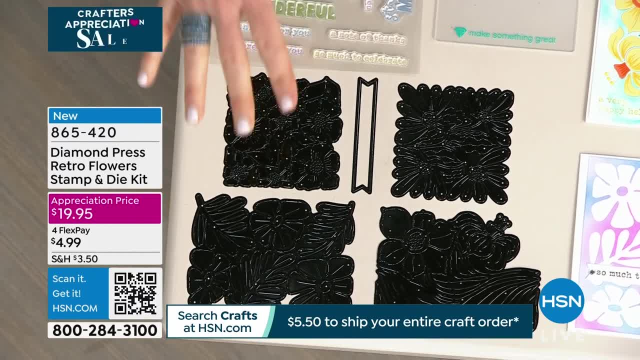 piece And you might be thinking: okay, what does this mean? How does this happen? So what it means is: I'm going to, we're going to come back around here. I've cut it out on one piece of cardstock. 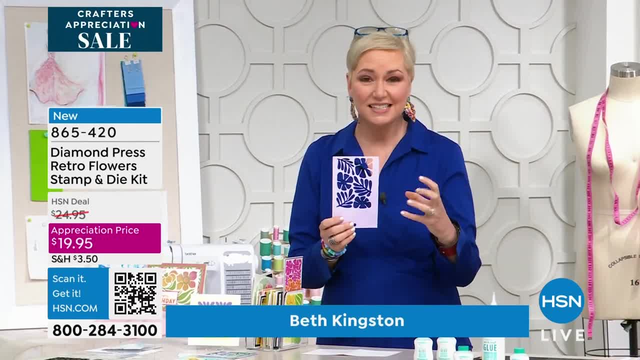 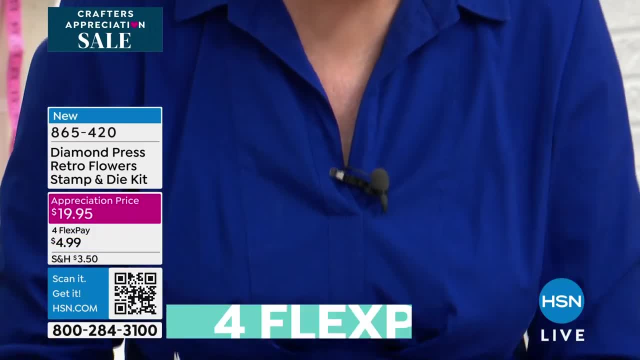 All the little pieces come out individually. Why is that so important? Because it lets you create. So this is. I'm going to show you what comes on the inside in a second. So this is what cuts out for you. You can lay it then on a piece of cardstock on top of your cardstock, And then you 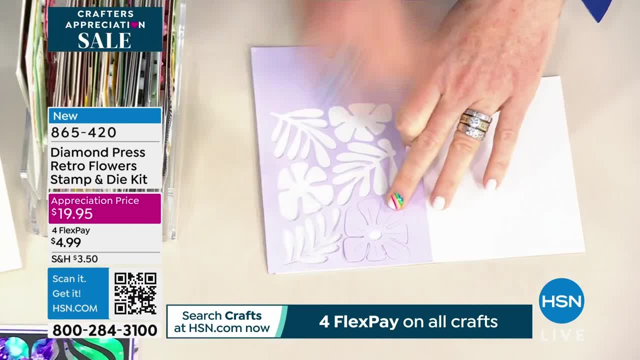 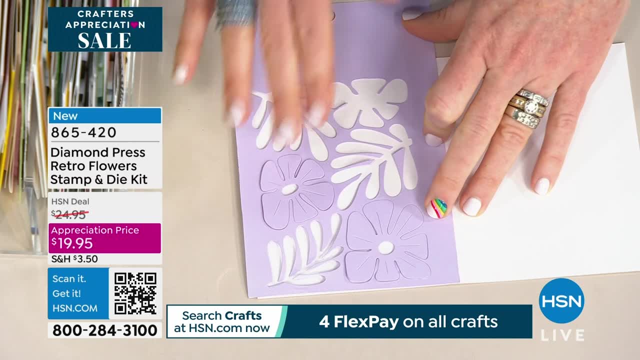 can start layering these intricate pieces in and it's going to let you create these puzzles. And you may be thinking, okay, I sort of get it, but I don't get it. Let me show you the finished projects. Look, so you're going to take whatever pieces of cardstock you've got at home- blah. 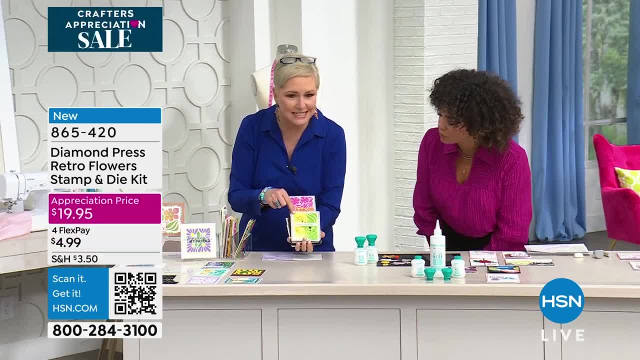 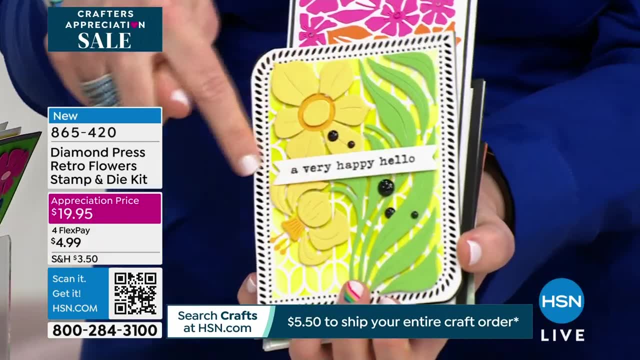 blah blah And you're going to turn them into. look at, look at the detail of this card. So these are all dimensional cards. So you know I love to talk about value. You also get the sentiments of very happy Hello. I'll show you some of the others as well. This card would cost. 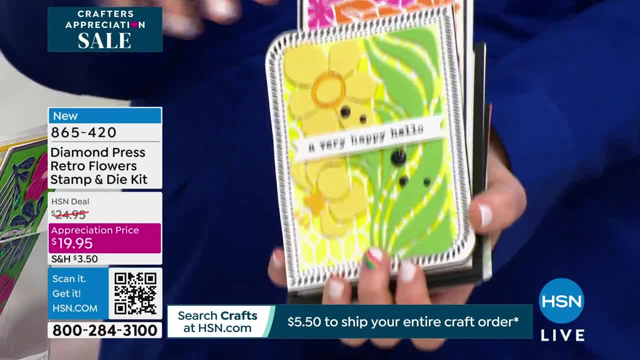 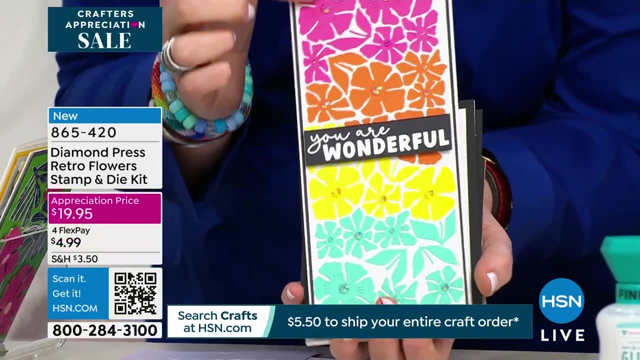 $6 or $7 or $8 at a very bougie card store. easily all day, every day, You're using scraps of paper you've got at home, So very happy. Hello, Look at this one. These are all individual flowers that you wouldn't put on yourself because you're like, okay, that's way too complicated. 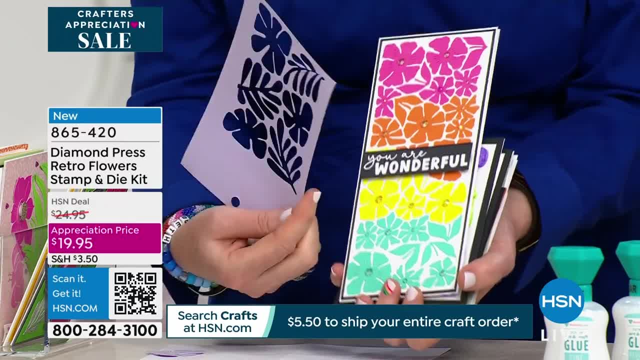 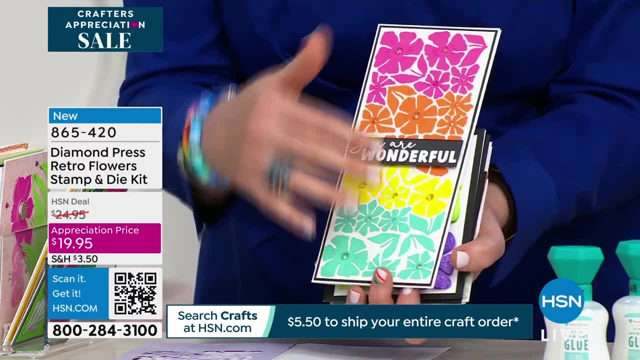 When you're cutting out the pattern of each one that you can just lay over. it's like a puzzle, but it comes together so beautifully and easily. So if you were an advanced crafter, you may put something together like this, but it would take you about 700 hours. 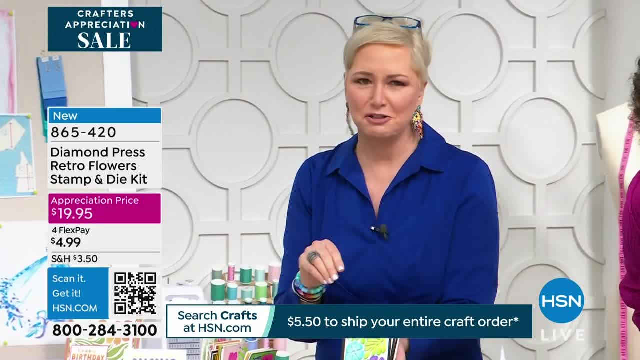 This is for beginning crafters. I can just do it right out of the gate. Nicole was looking over my shoulder and she's like, how do you do this? And I was like, look, it's a puzzle. And she's like: 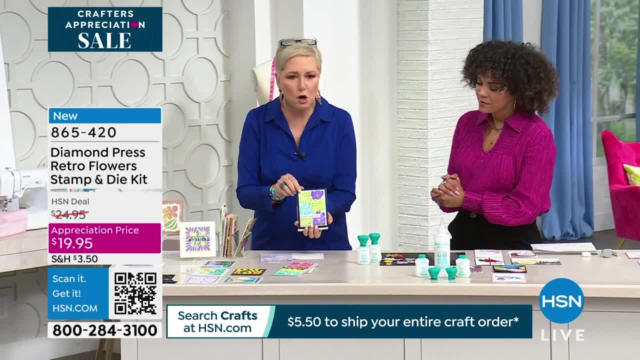 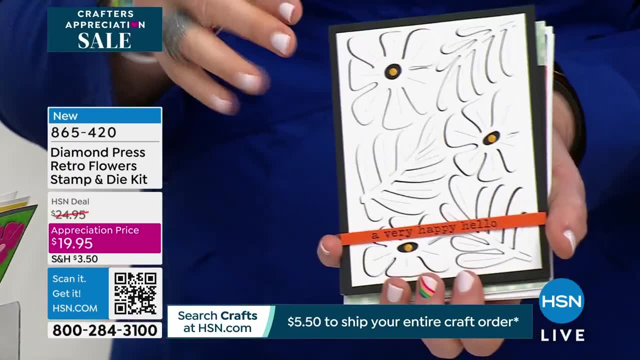 oh, this makes total sense. but it just makes the most beautiful intricate cards. And because you're cutting out all the different shapes, you can mix and match patterns. I mean it's just absolutely here, Tone on tone, white again, six, seven, $8 all day, every day at a card store. 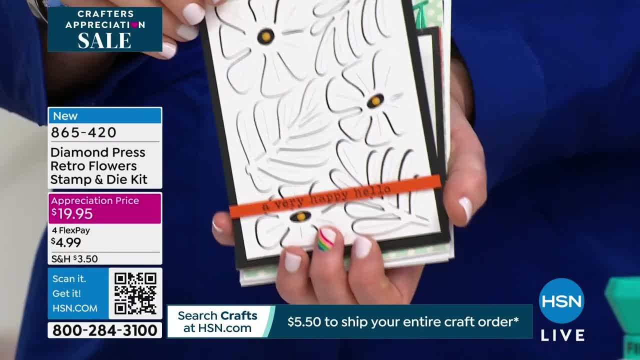 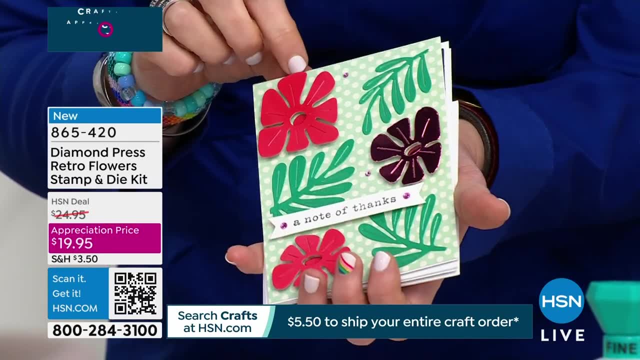 You're doing this with a piece of black scrap paper and a black piece of white paper, But look at this. This brings it to life, right? That's what I love. And because they're individual pieces, you can pop them up with foam, You can pop them up with all that I mean, but it just is absolutely. 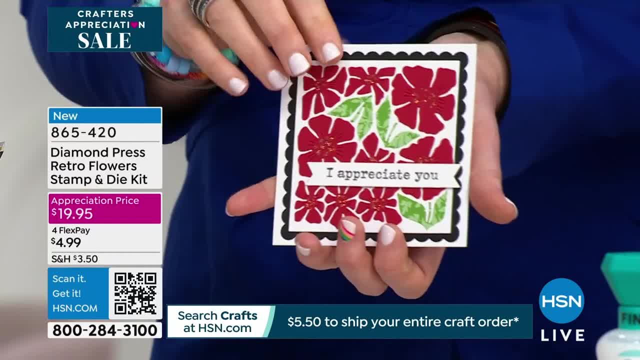 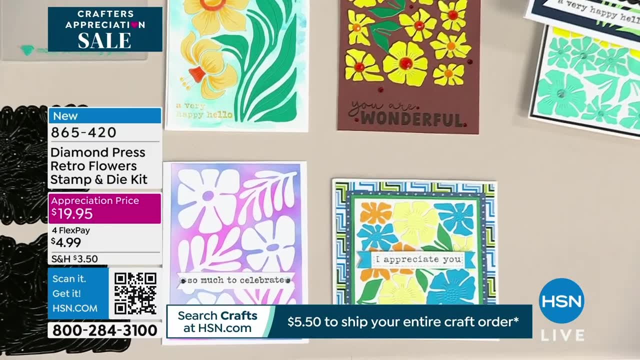 incredible. So I want to show you a couple of like look, can you believe these are from the same card set. So here's what I got: a whole pile of things I want to show you. So this card and this card, it's the same set, but because if you're a beginning crafter, you can just cut it. 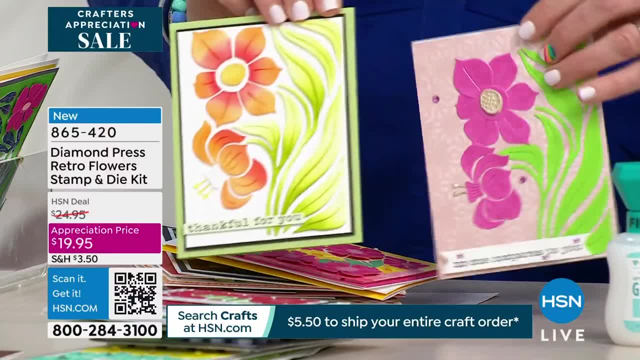 out of regular card stock. If you're a more advanced crafter, you can go ahead and do the chalking, but they both have the same set. So if you're a beginner crafter, you can just cut it out. both make beautiful cards and it's for whatever skill level you have and whatever you want to. 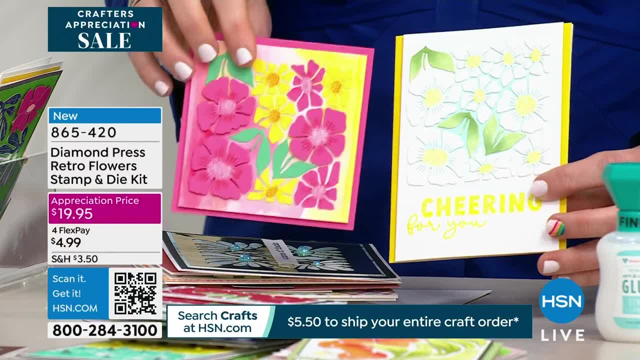 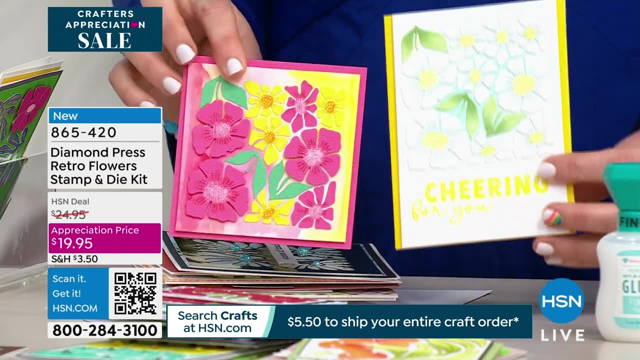 create. Okay, These look like two completely different cards. They are from the exact same die set. You can see how it lines up, but they look like two completely different. So, whatever your theme is, this would be great for a luau. This would be great, you know, for something. 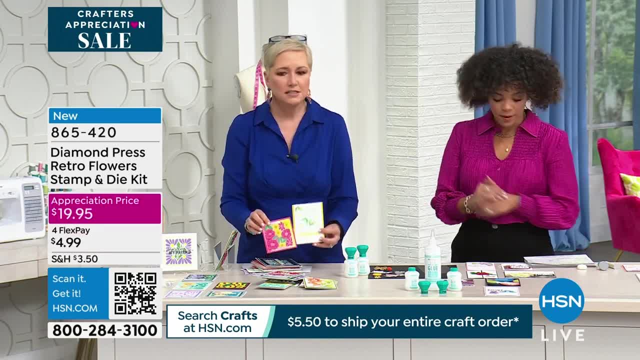 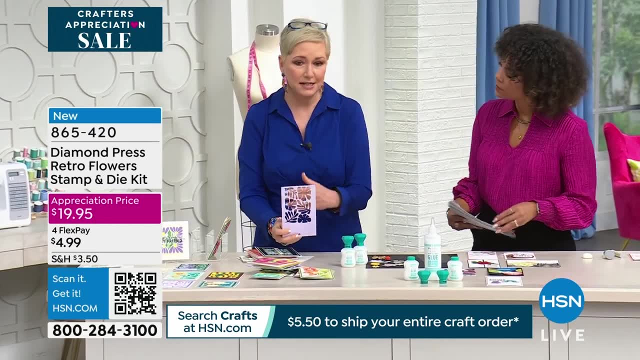 festive, but then you could also do these for baby showers, wedding showers, something really classic and beautiful. That's what I think. And and oh, by the way, because you're cutting out your essentially stencil, for lack of a better word. 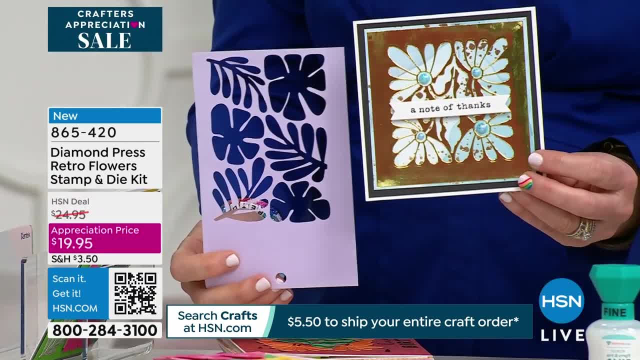 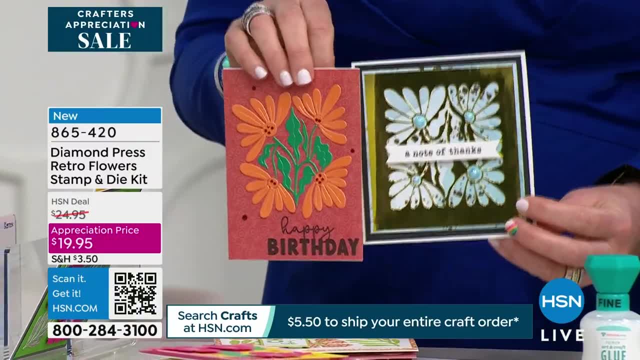 one piece. you can also use the negatives to create gorge. So that's the negative of this pattern. So there is no waste- Yes, exactly No waste with this set. You know we love to use all our stuff. This is a way you can use If you've got those pieces of paper that you're like you. 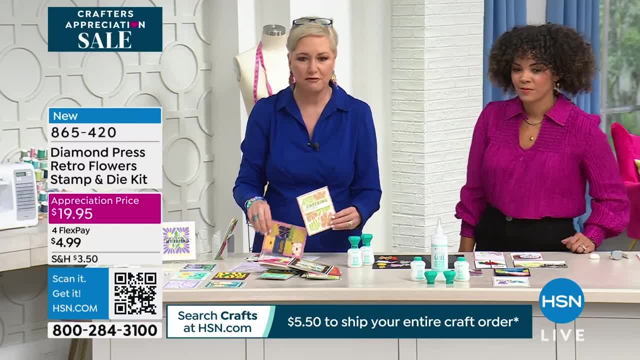 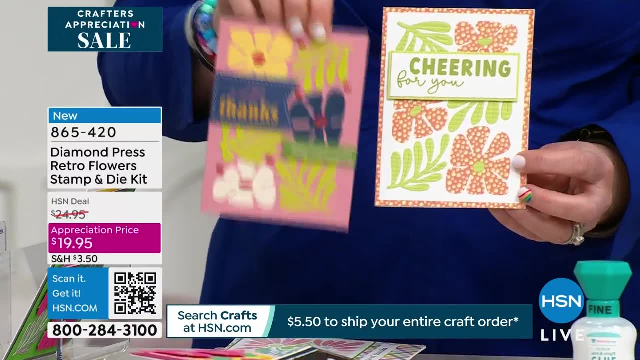 know what. this is really gorgeous, but I don't want to use it on something where I'm going to have to throw half of it away. This is the set for you. Again, same exact die. You can choose the colors you're using. You can choose the way you put it on the card. All of these great projects. 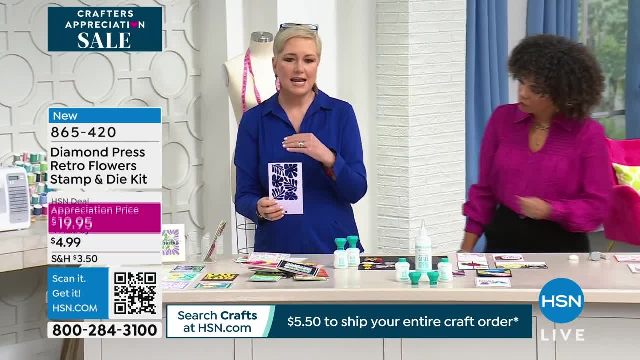 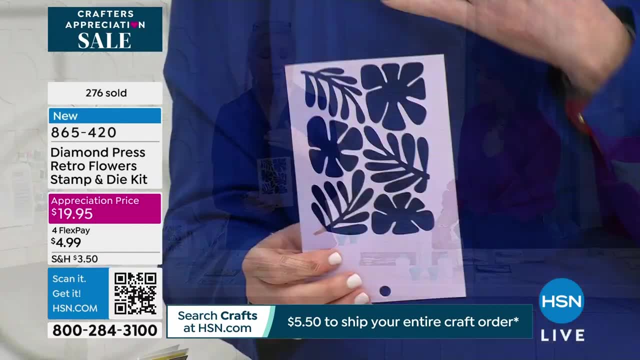 that you are doing. But to do something like this and hand, put them together and be like, okay, well, I need a two inch circle, two inch flower over here and a half an inch leaf over here, You'd never do it, And so. 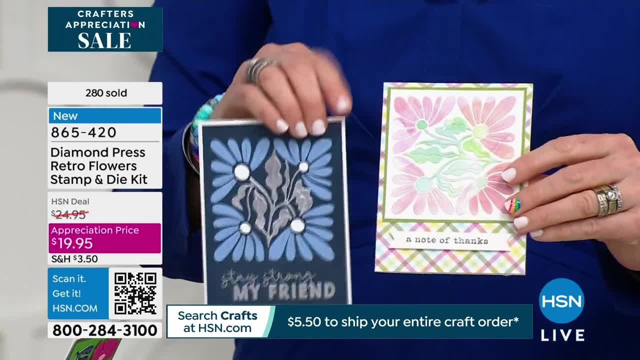 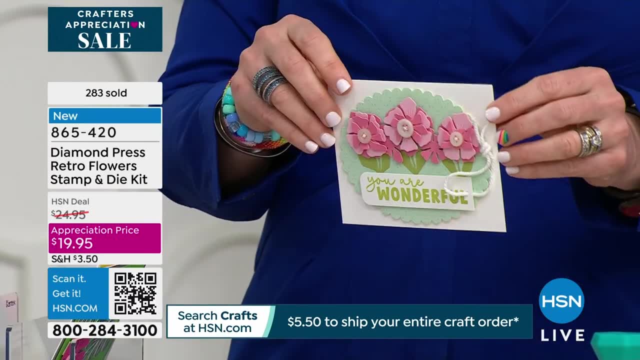 you're not creating these really gorgeous projects. This is what it's going to do for you, And this is a perfect time of the year to do this too. We're in spring, we're in summer. Think about making a baby shower card that you could put together right, Adding those different belts. 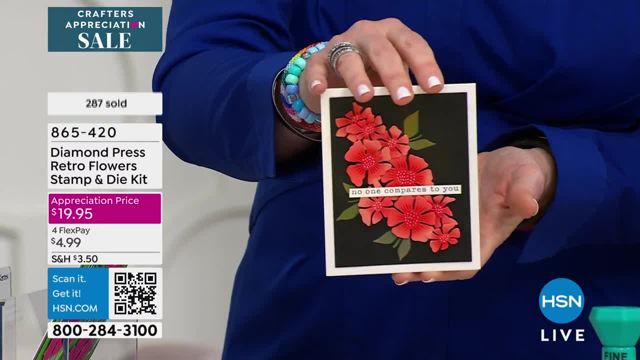 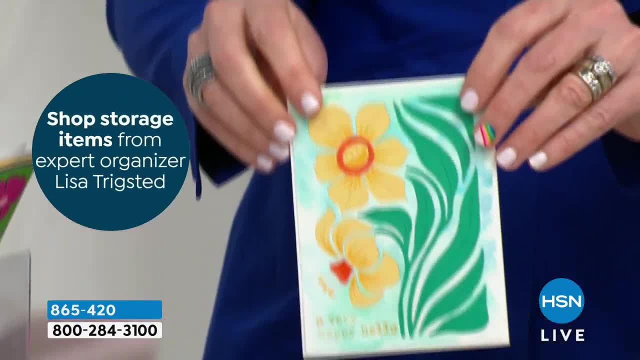 Maybe it's a wedding card that you want to put something together too. What I love about the kit that you're getting: it's very small. It's very portable. This is brand new. Remember, in a customer appreciation price, everything that you're seeing on air is on sale right now. So instead of paying about 25 bucks or under a $20- 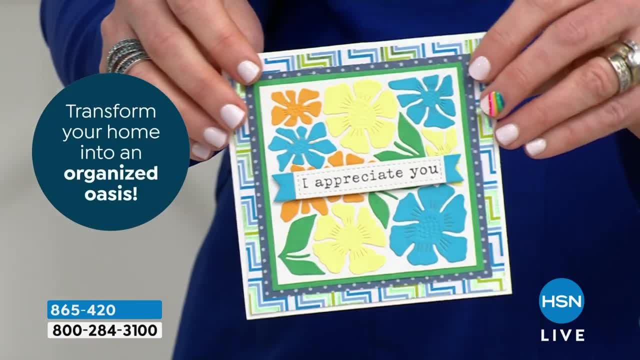 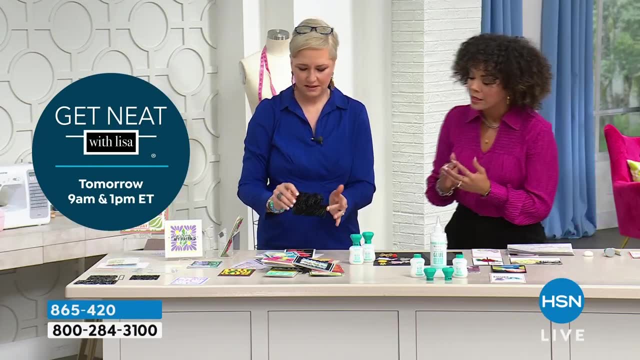 bill to get this home. you'll get the four by six blank folder. You'll get the card scraper. You get two adhesive sheets, the instruction sheets that you need, five dyes on one card, 10 stamps on one of those clear sheets. So you're getting everything that you need, whether it's scrapbooking or the. 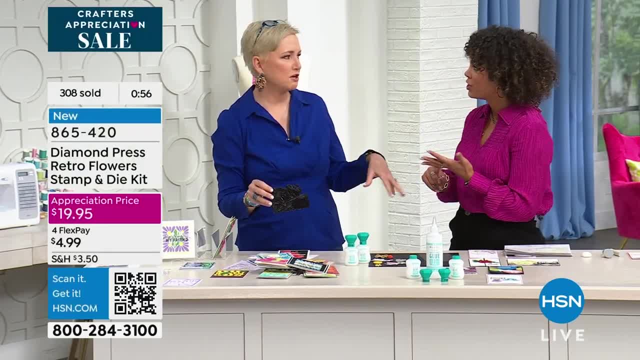 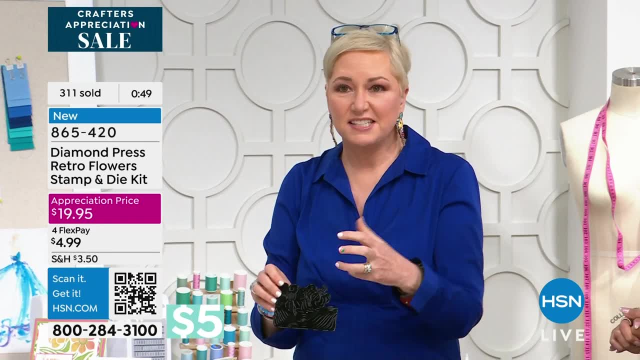 cards or maybe you're making gift tags or anything that you really want to embellish. Oh, this would be so cute for tags- If you're going to be doing this, and just portable again, if you wanted to make an elaborate floral card and you had to have seven different flower dyes to make it, that would be. 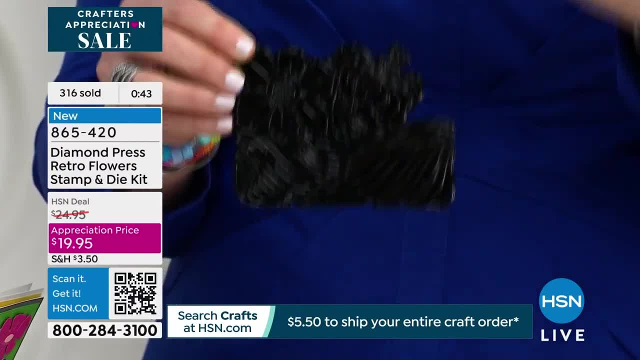 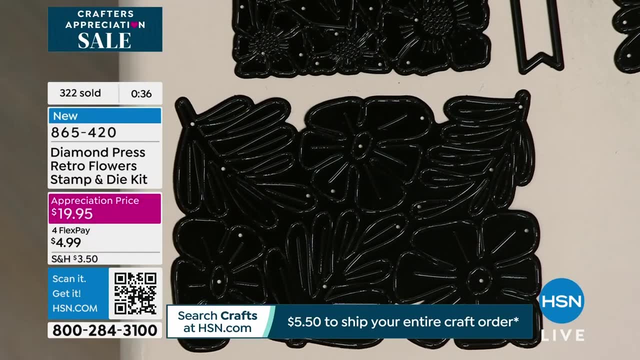 a problem. This is one dye. So you've got all these great configurations, You've got all these great florals, You've got all these great leaves, but they're in these larger shapes and you're cutting them out at one time, which saves you time. Then you can use the use them mix and 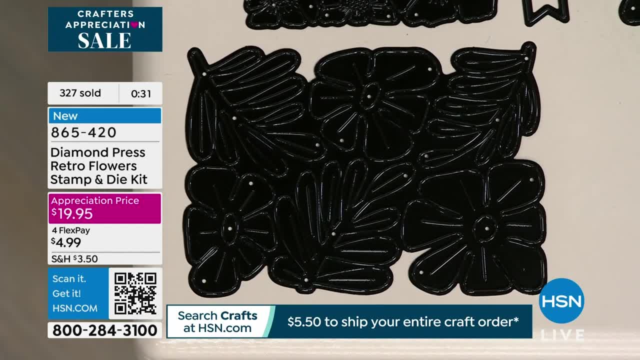 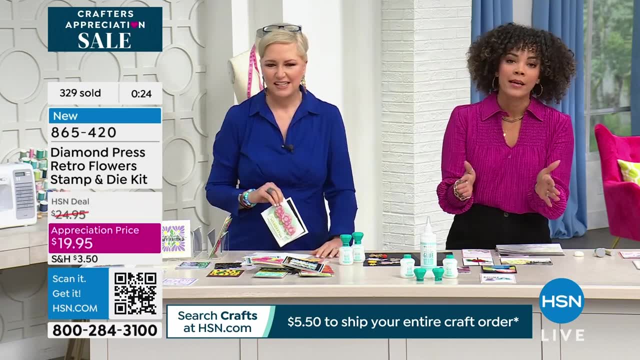 match as you go. By the way, just before you share that, we're seeing the sold counter. Now this is brand new. We only brought in a thousand, So, with many of you jumping into the pouring room, we're going to be halfway through our quantity. So remember, load up your card. 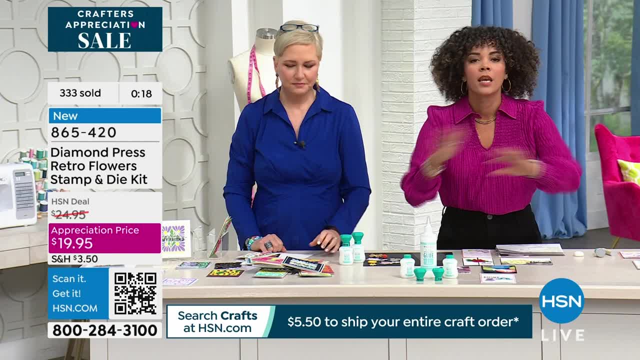 $5.50, we ship it to you. Well, Nicole, I already checked out. Are you going to charge me $5.50?? No, it's only $5.50 for the day. So here's the time to jump in 865-420.. What did you want to? 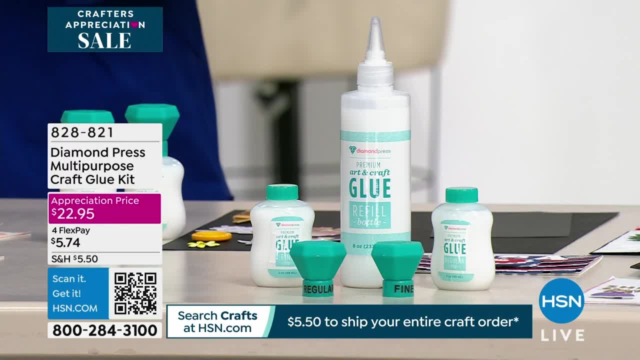 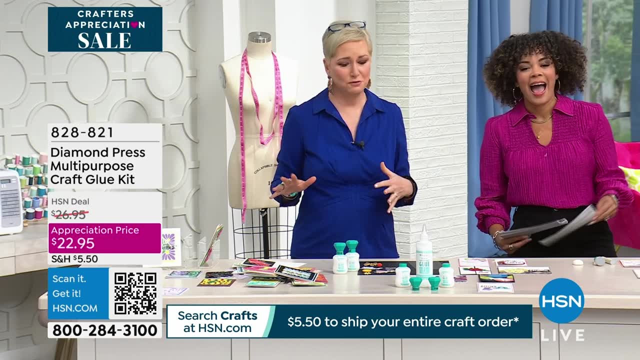 say. I just wanted to say that, like you can mix and match all the shapes and all the sizes, And so you've always got embellishments ready to go, whether you use them for your cards or your scrapbook pages or whatever you're working on This is. it's such a really cool set and $19.95,. 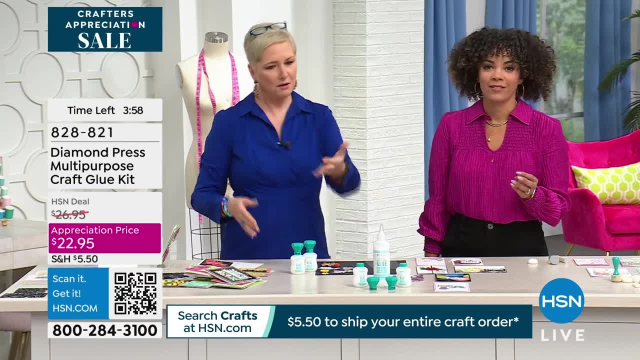 which I don't really get. I don't know how you guys do this all the time, but okay, I don't know either. Oh, here we go And here we go. So this is really perfect. So, thinking of layering embellishments. 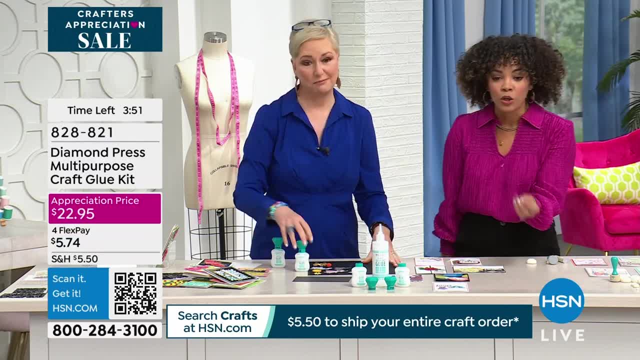 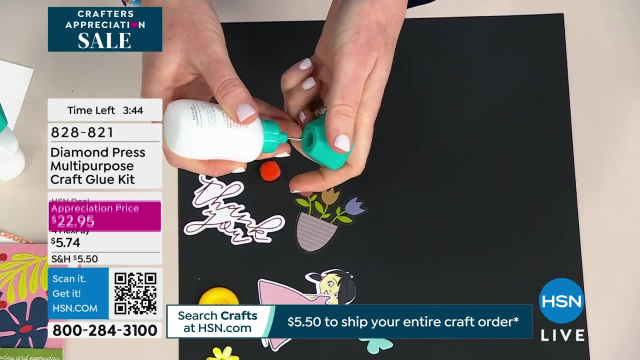 a lot of time. you need something to stick with it and adhesive. This is a glue kit that you're getting. Yeah, really, All the time you need glue, All the time. You can't just press it and hope that it stays there. What's great about this glue kit is actually the fact that it comes with 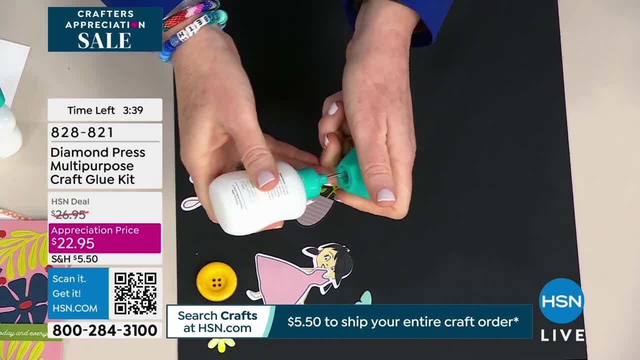 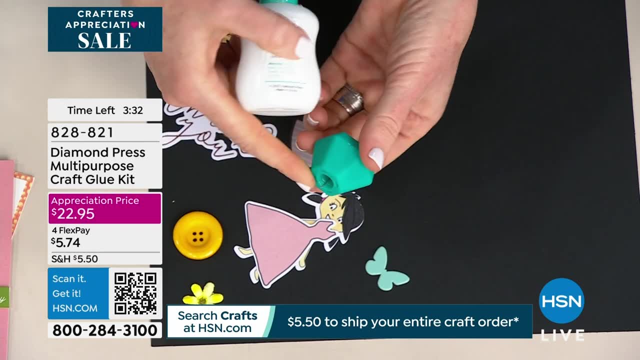 two different tips. It comes with a regular and a fine tip. So you really need that precise, just that little dollop of adhesive, then it sticks and it dries clear. That's what's really fun, And oh sorry. What else is amazing is the tip which I'll talk to you about. 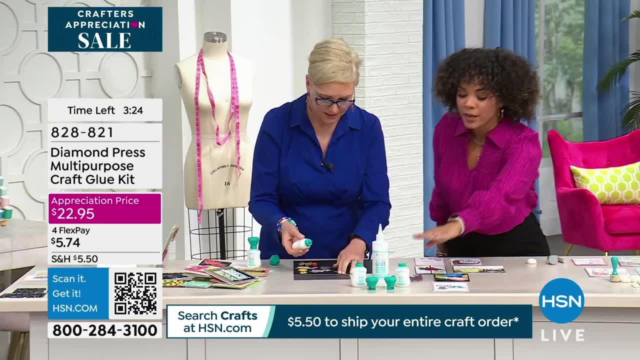 how to use it. Yeah, So it keeps it from gumping up. So sorry, I just interrupted what you were doing. Oh, I love that. Okay, So you'll get two bottles of the two ounces, and then you'll also get a. 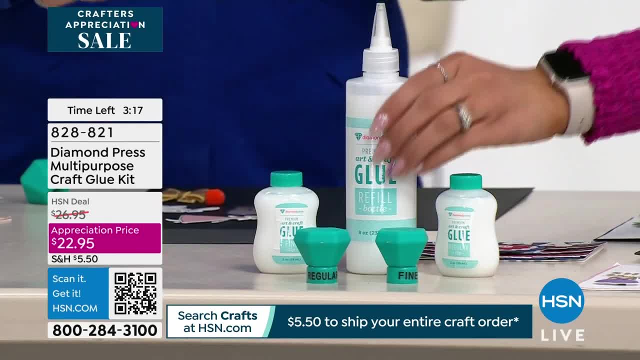 refill glue bottle that is eight ounces. Look at the size of this thing, Look at the size of that thing. Refill bottle, meaning it's not empty. You will refill the other two ounces, and then there's the tips that you get. All right, All you, Beth. 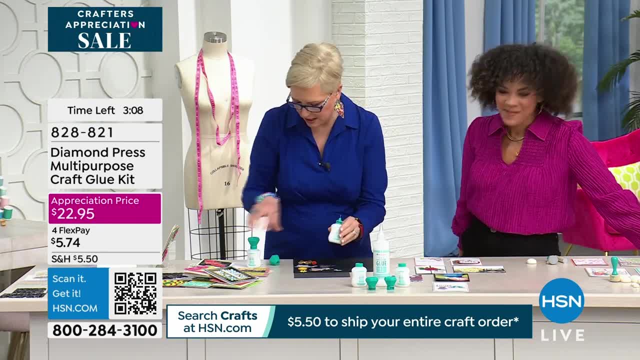 So here's, and I'm just like so excited, I'm like: let me tell you all the things. So you're getting a fine tip and you're getting a regular tip. It tells you exactly what it is on the bottle, So you're never having to guess. but here's what makes it special. 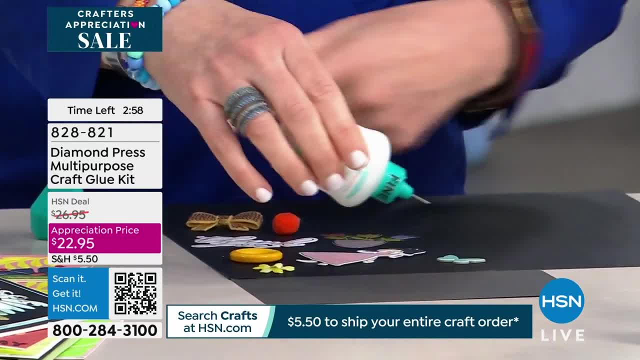 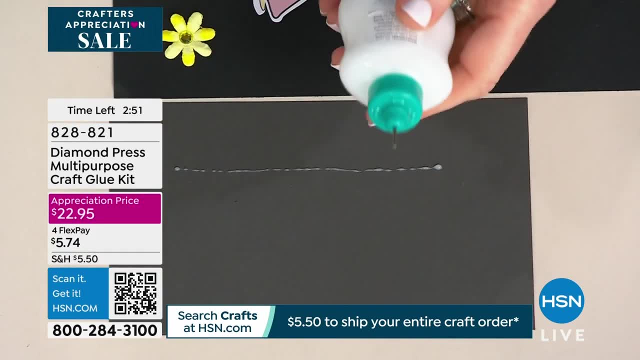 So I'm going to squeeze this out. It's got a metal tip And then it's got a metal, so you squeeze it out, So you get a nice solid line of adhesive. Yeah, Then when you're done using it, 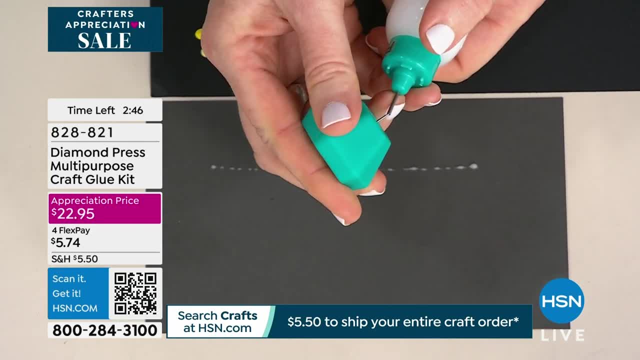 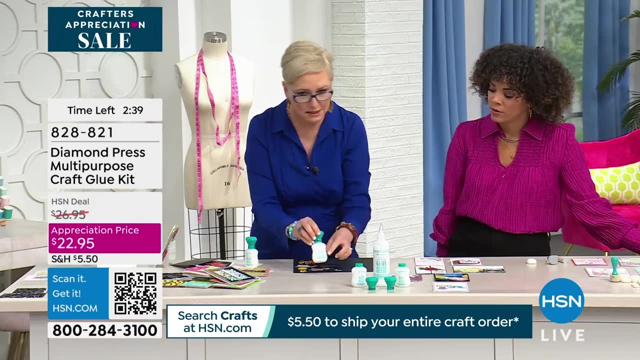 you see this little needle right here. This is going to go right inside the tip. So it is never hear me, never going to goop, never going to get stuck, never going to. you know how sometimes you like, especially with craft glue, it comes with a plastic tip and you'll cut it off or you'll open. 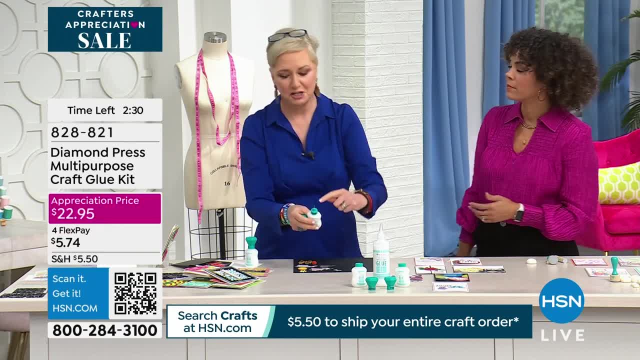 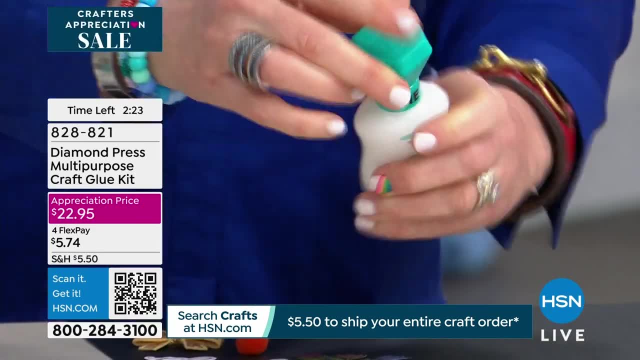 it up And then the next time you use it you have to cut a little bit more of the plastic tip off because they're stuck, And then you have to cut a little bit more of the plastic tip off. This will go right back inside, So it is never going to dry out. And here's the other thing. 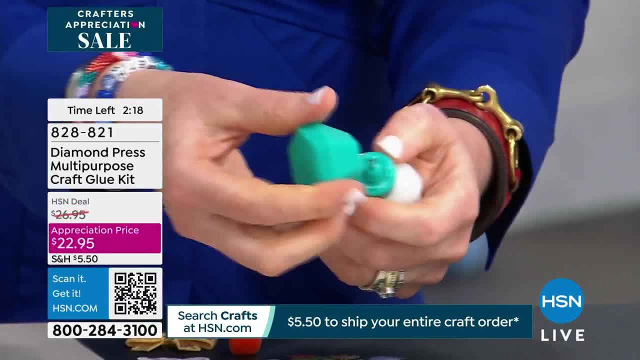 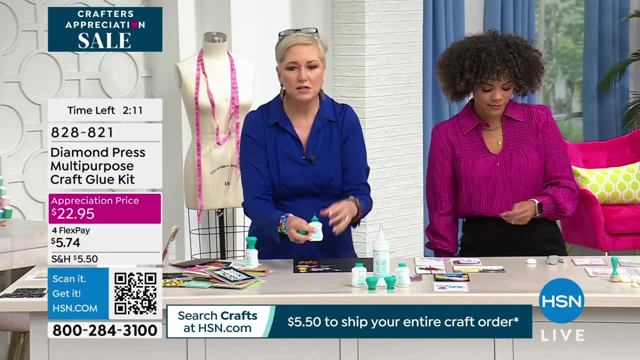 It doesn't. you don't have to twist and turn it, It just pulls right off, So you're not having to worry about. you know, sometimes if you have things that have the ridges, if you twist, it doesn't turn tight enough, So then it dries out. You're never going to have that issue, So 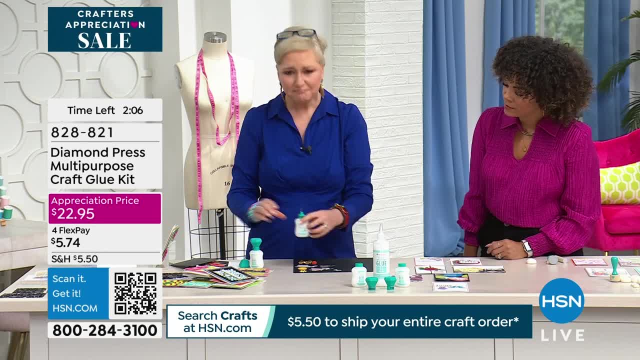 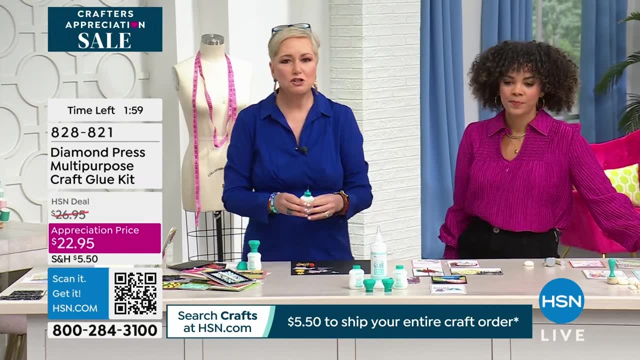 you get both the regular and fine. Here's the thing We like to make crafts. That's why we're all here, right? Yeah, Every single craft, you need to use adhesive of some kind, And so you want to use adhesive. You want to use adhesive of some kind. You want to use adhesive of some kind. 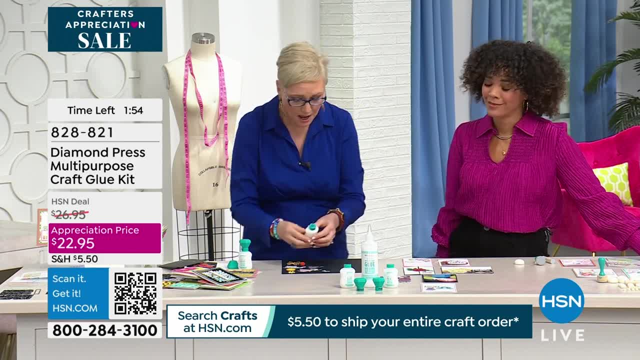 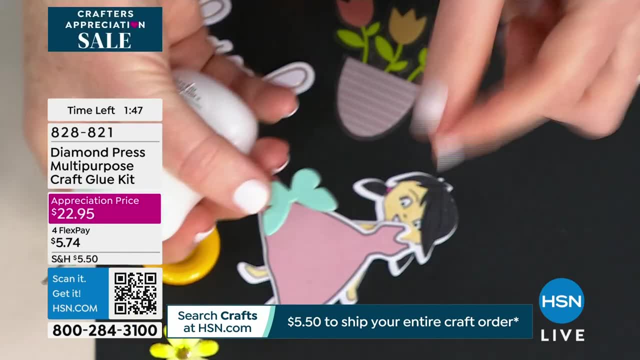 For $22.95, you're getting all this incredible adhesive, but it's just so great because of the tips You can use it for all these intricate So like. you may use a tape runner and you may think you know that's all I need, But when you're wanting to use these really intricate embellishments, 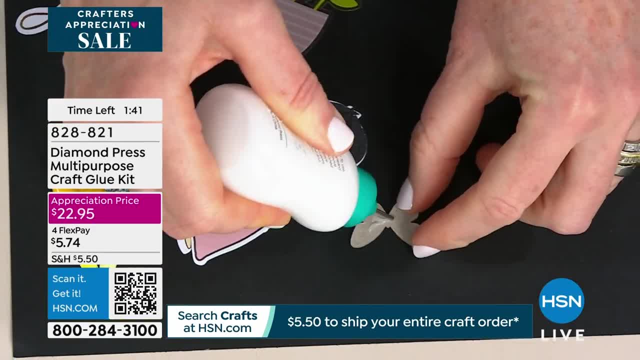 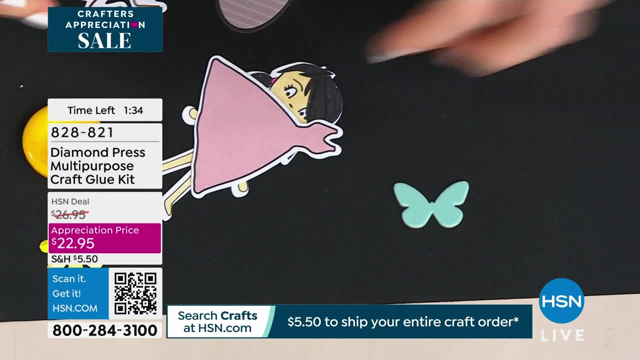 you just take a little bit of the adhesive and you sing while you're doing it And then you flip it upside down And because you can control how much glue is coming out, that's going to stay. It works on chipboards. It used on this is some of the Kingston Crafts paper dolls. 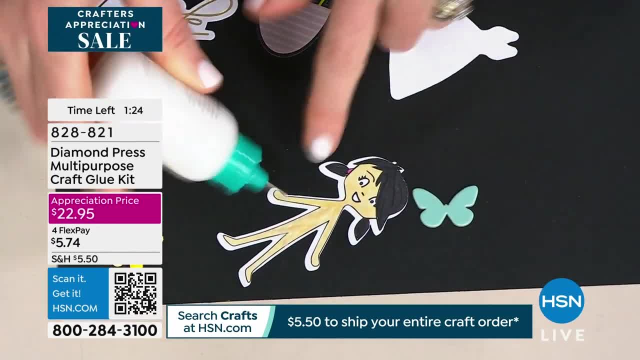 if I want to put this little dress on, I just but look at how beautifully I can control it. This is a. I know this sounds weird. This is a thin, a thin die, a little thin body, but I can take it. 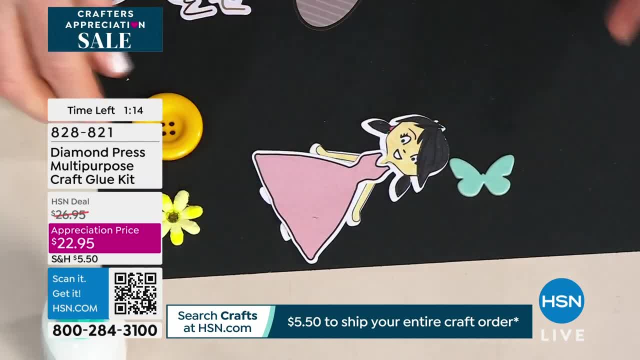 add the adhesive. Now she's ready for the party. Now she's ready for the party. But all of these embellishments you got, oh, okay, You want to use it on plastic? Sure, Let's do that, Like all of. 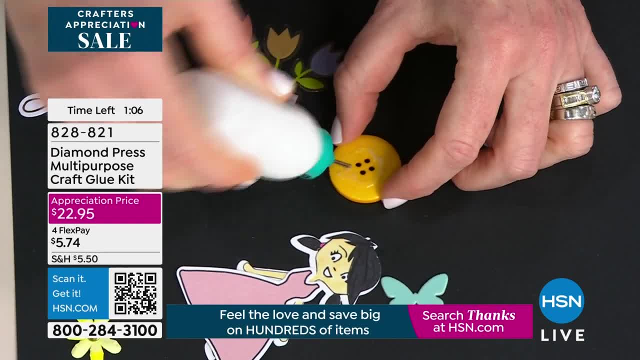 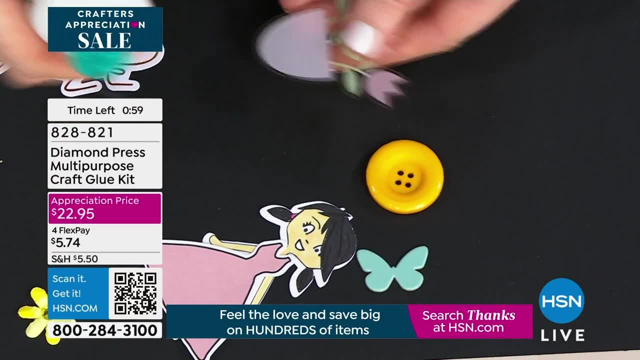 those embellishments. you've got that you've thought: okay, I don't know what kind of adhesive to use, because a tape runner won't work And I don't necessarily want to use a glue dot for everything. How about acetate? right? So acetate is something that we 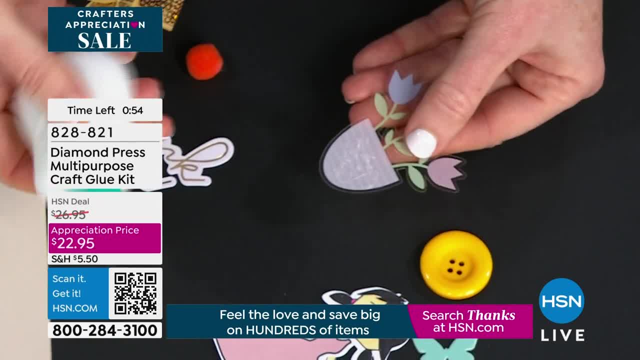 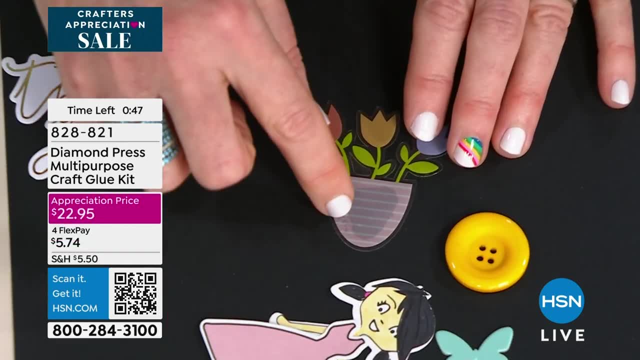 all that we've all started to love and use again. but you think, okay, how am I going to get it on there So it doesn't show through? Look what happens. So you do that and then it's going to dry clear. but it shows you that it's sticking and it's not squishing out the sides. That's. 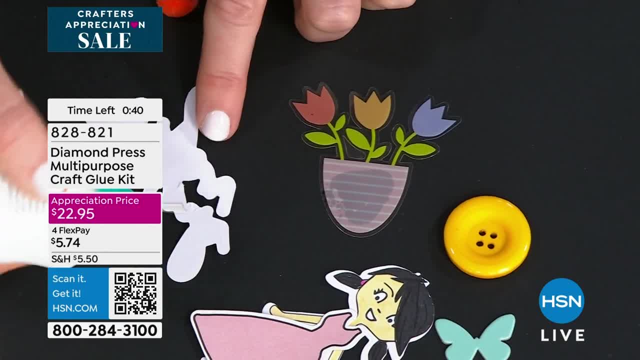 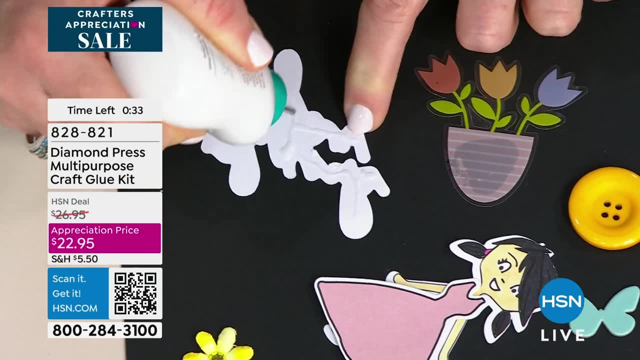 going to dry clear for you. You have so much control too, as I'm watching that, And that's what's great about having the two different tips. You'll have kind of a finer tip and then your your regular tip, which is really nice And you can have great precision with it. A lot of you. 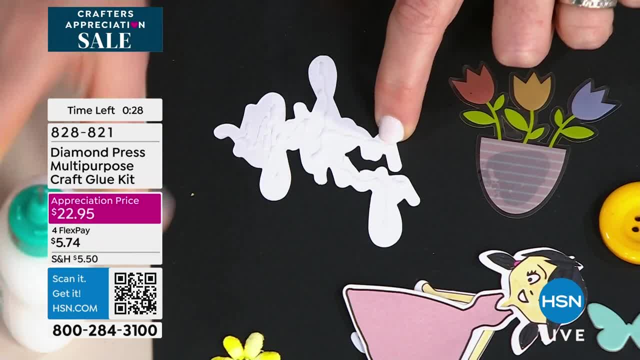 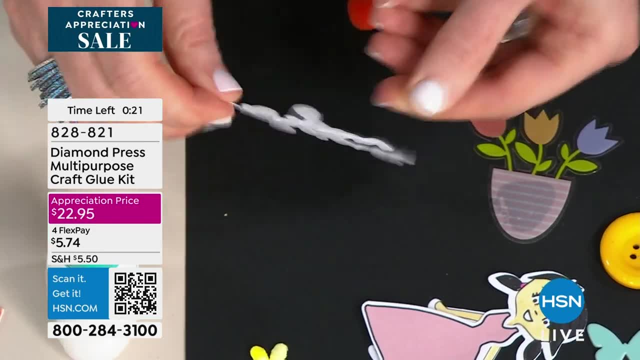 are jumping into the ordering process. Remember, this is another um great reorder. we just got it back in stock for you. Now to customer appreciation price at $22 and some change. Remember, load up your cart. $5.50 shipping just once today on all your crafting. And then. 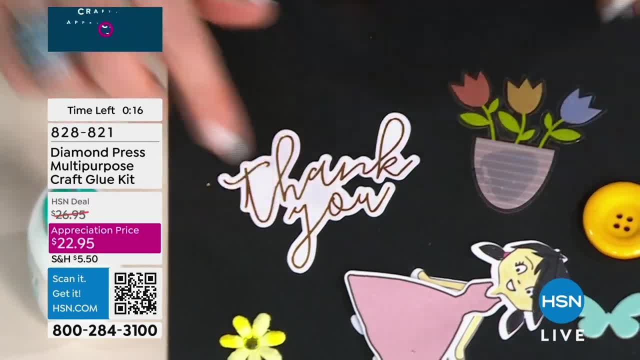 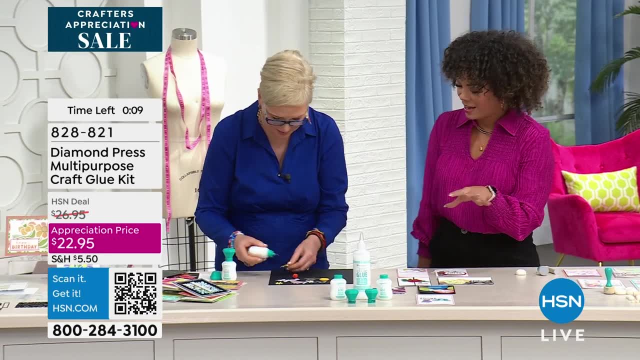 everything else that you keep adding for the day throughout crafting. you are able. we cover the shipping. It's just $5.50 once. 828-821 is the item number. Look how fast that is going. I love it. And to your point like this, is a super intricate dye If you were using a regular glue. 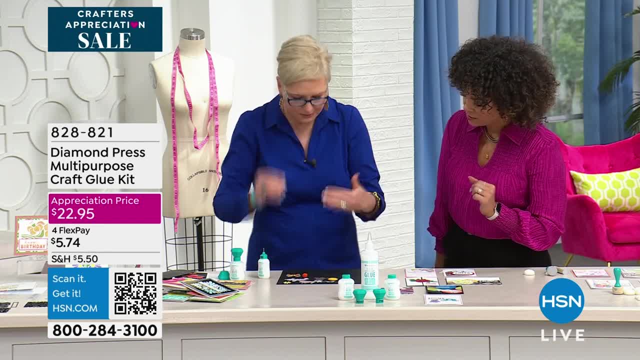 tip. you'd have like glue squishing out everywhere, but look at all the different types of materials I've been able to glue down. That's what I think is important when you're looking for adhesive. You don't want to be like 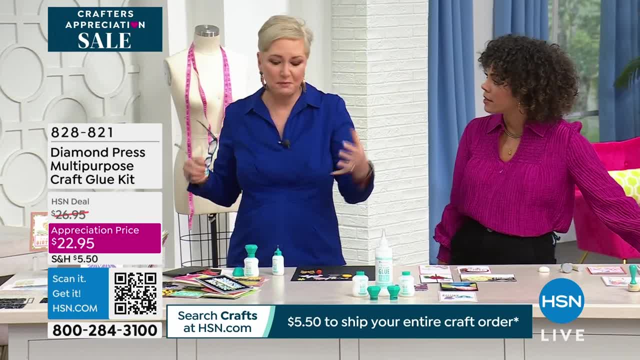 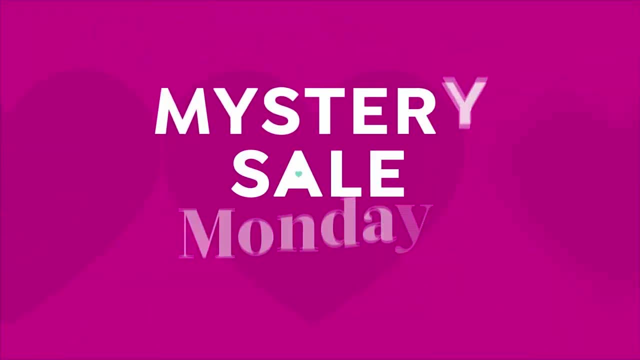 well, I need this adhesive for a pom pom and this adhesive for a button and this adhesive for paper. Use the same adhesive for everything. It's so so, so, so good Love that, All right, Stay in the ordering process. 828-821 is the item number. Well, 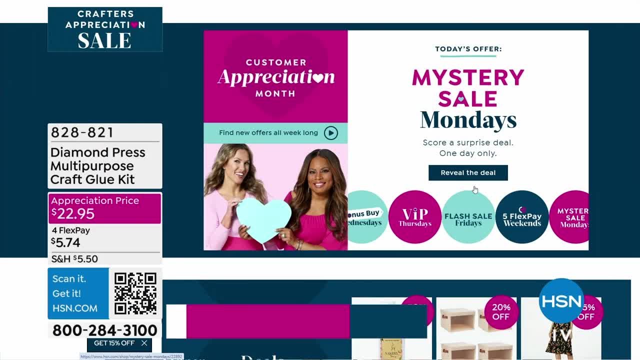 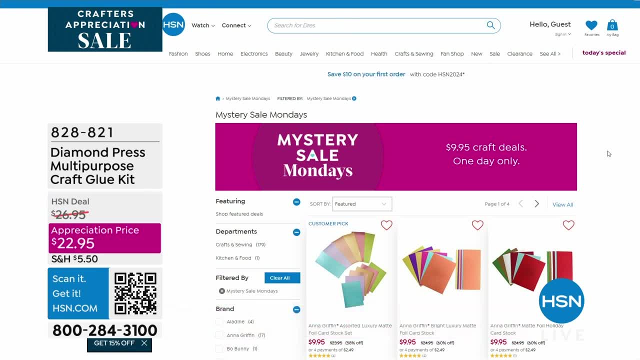 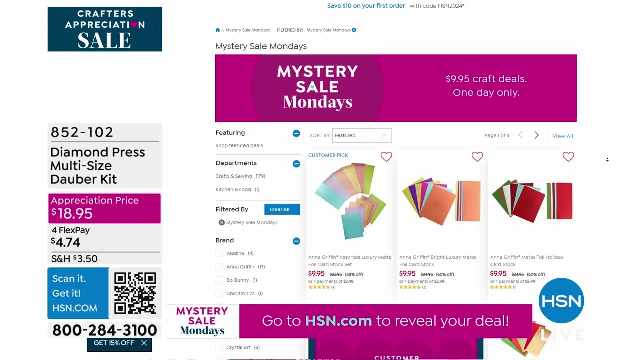 since it is customer appreciation month here at HSN, something that we're doing throughout the month of April for a thank you is mystery sale Mondays. So that is your key three words that you'll search is mystery sale Mondays. We have crafting 95 deals. Nothing is over $10.. I love that There's so much good stuff in there, So much. 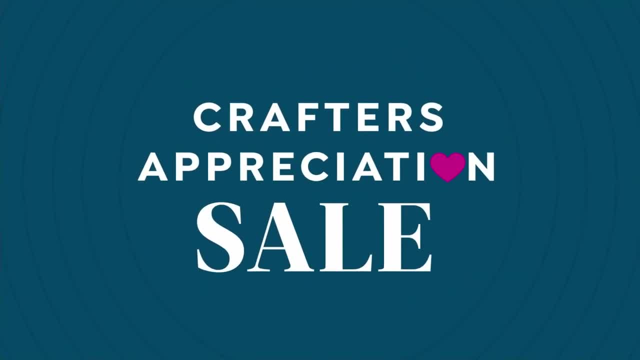 and load up your cart. It's five, 50 shipping just one time- Cause that was the question I asked. I was like wait a minute, but what if I have 10 things? Okay, It's five, 50, and then I check out. 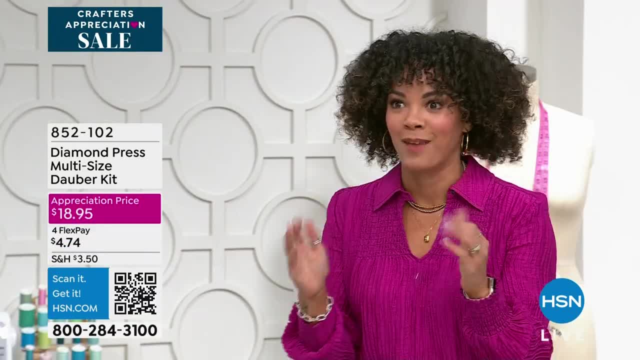 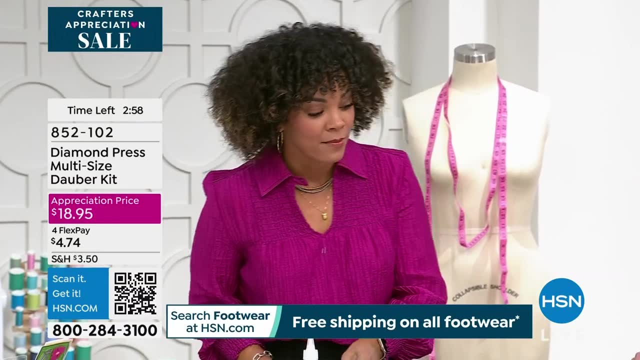 and then I want to add another two or three things still covered. It's five, 51 times. So that's what I love about this. Okay, Another thing from diamond press that is always very popular is the dauber kit and has sold out a bajillion. I know, I think this is my first time, actually. 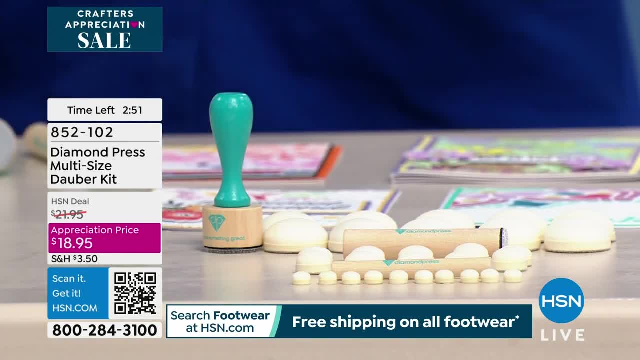 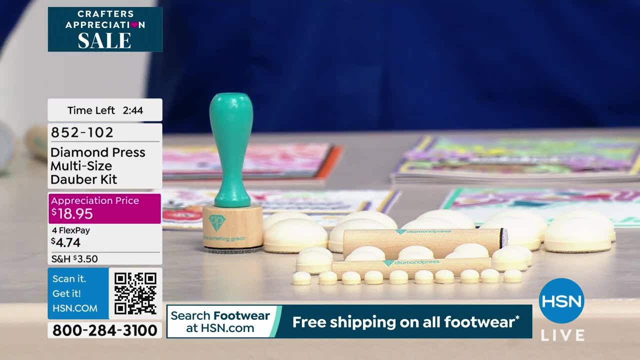 having the opportunity to show it. So it is a great reorder opportunity. appreciation price at 1895.. So you'll get the main dauber, Then you'll get extended handles. You also get the foam dauber heads. There's 30 of them included, all different sizes. This is what I love, because 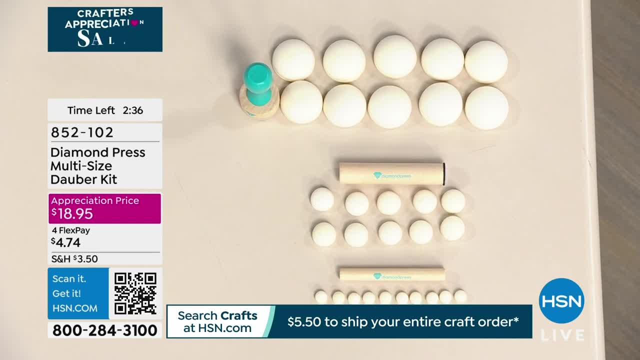 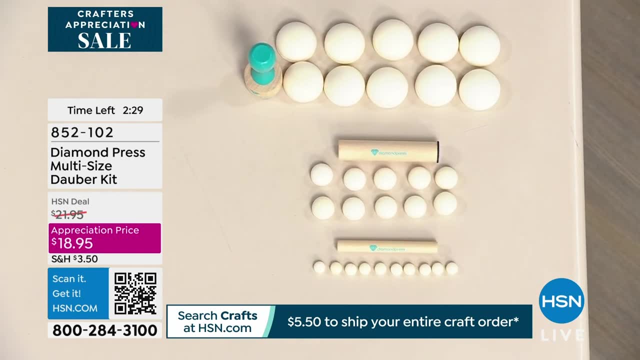 this is adding like a really beautiful kind of like final touch to something. Oh my gosh, Yes, That's the perfect way to put it. So we have always sold the larger daubers and handles with all of our diamond press inks. but what our customers have said- and it's a great thing- 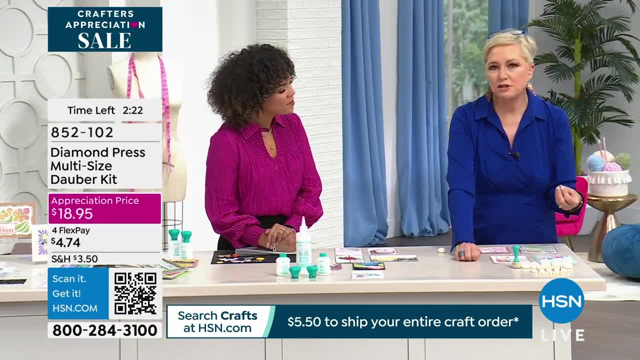 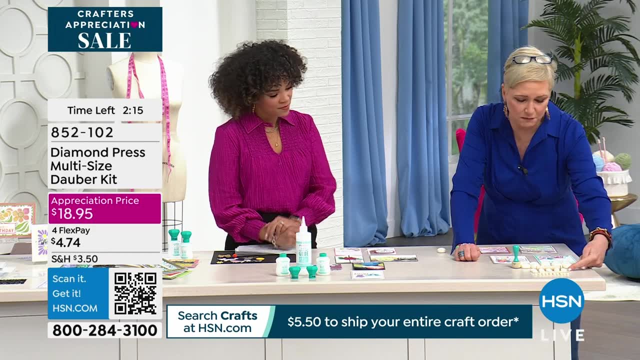 about HSN and diamond presses. We listen And customers have said: okay, you've taught me how to use all these great tools. I need something a little bit smaller so I can create these more intricate projects. So we've done two smaller sizes, We've done the smaller and then we've done the mini, which I absolutely 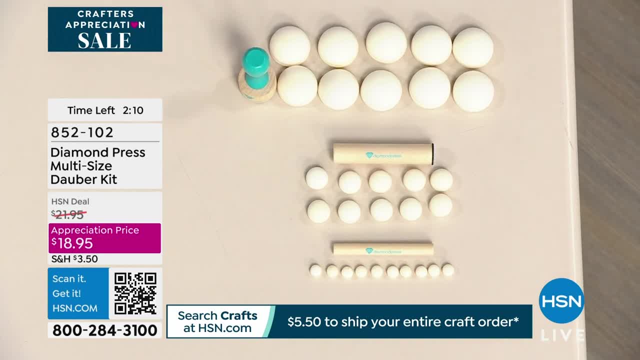 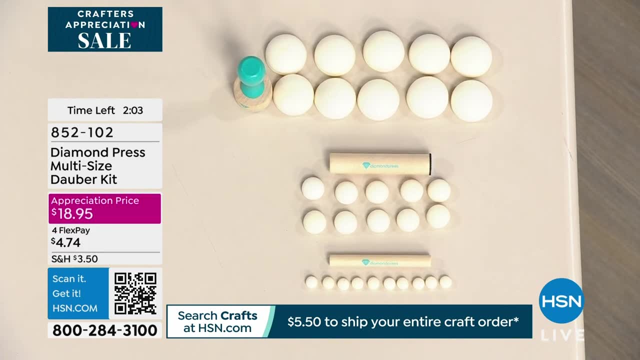 love this little guy down here. but what's so great about these? And I just- I know we don't have a lot of time- I want to show you some finished projects. So if you're working with ink, if you're working with chalks, when you're doing projects like this, and there we've got the. 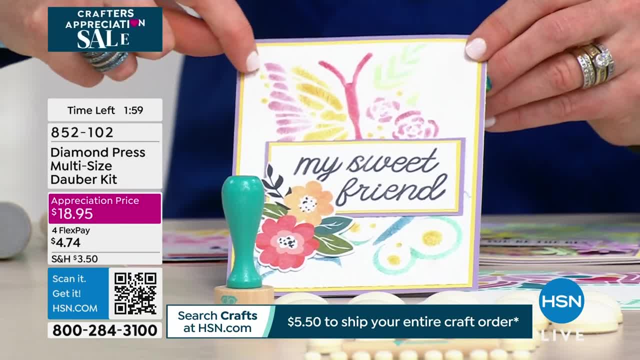 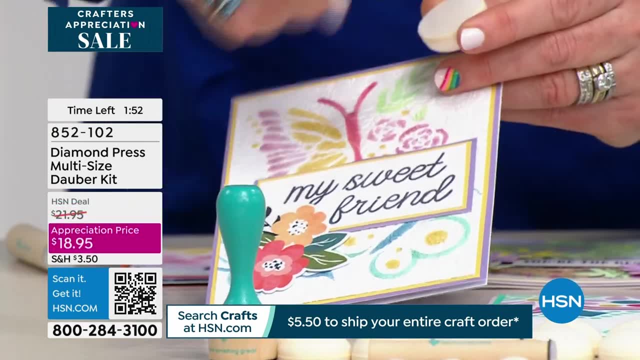 beautiful. there we go. Um, you can see how the color is different here than there's a little tiny bit of color out here and a little tiny bit of color out here, If you were using, and I'm, and here's how the daubers work. by the way, there's a little uh, Velcro on one side and 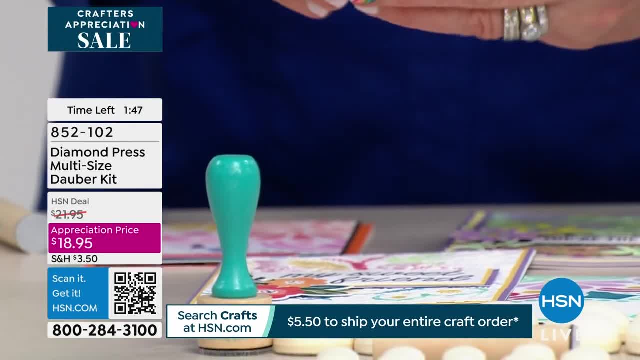 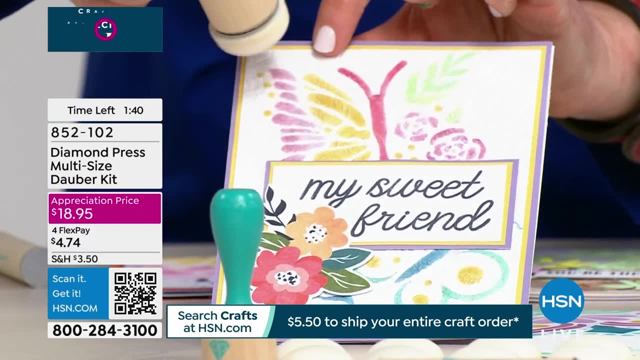 you just boopy it on and then it's good to go. You could center it if you were not on live television, But so if you were using something this big, there's no way, there's absolutely no way you'd be able to get this detail because, look, it covers everything. So you couldn't use chalk. 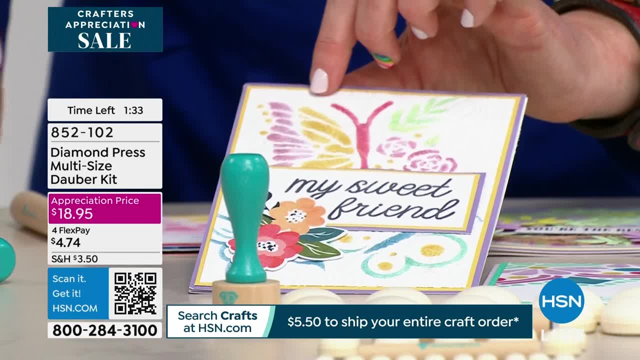 you know you'd have to be like: well, let me tape this off and let me tape. It. just takes too long. when you have the smaller sizes- And again, this one also uses the Velcro- You can go in and do. 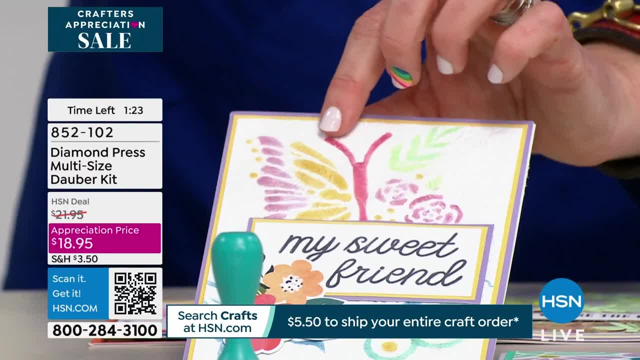 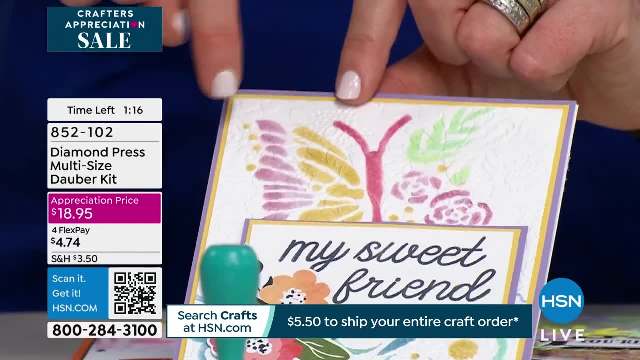 that little, tiny detail, and that's how you're going to get the really so. it's the same techniques that we've been showing you for years, but you never had the tools before to get into those little nooks and crannies, And that's what this is going to do for you. So, whether you're using 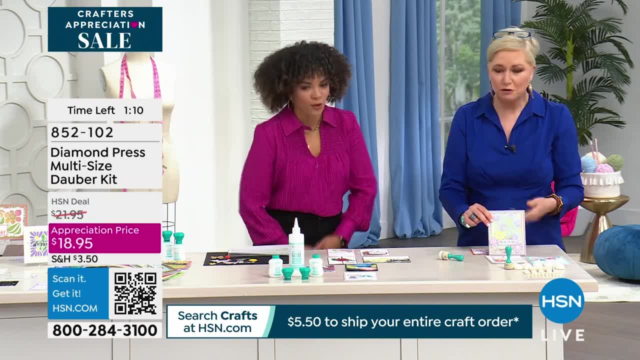 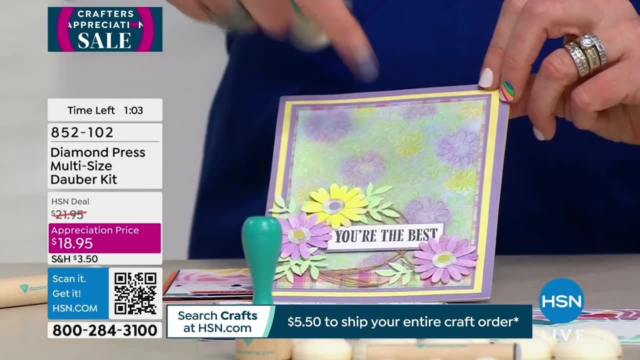 inks, whether you're using chalks. here's another perfect example. This is a full right. It's beautiful, But again, this size is too big for these flowers. So if you wanted to do this like little intricate yellow, you can't because this dauber is too big. You just go and decide which. 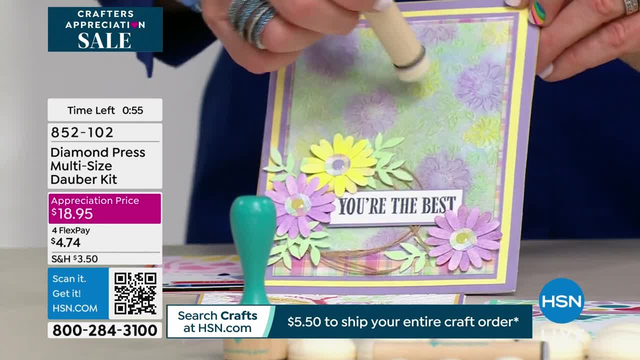 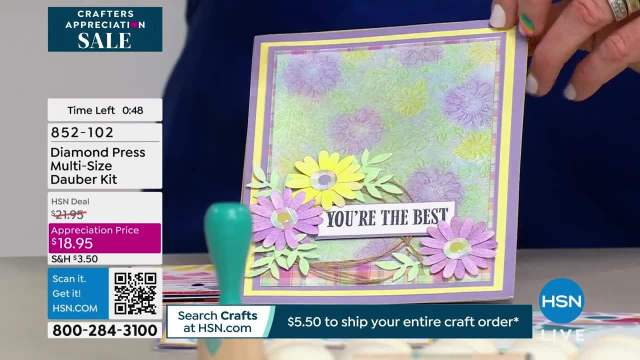 size you want to use. This one happens to be a little bit bigger, So if you wanted to do this, perfect my daubers just going everywhere. But because you have that kind of control now, you can do the smaller bits, You can do the insides of your flowers, You can get the detail. 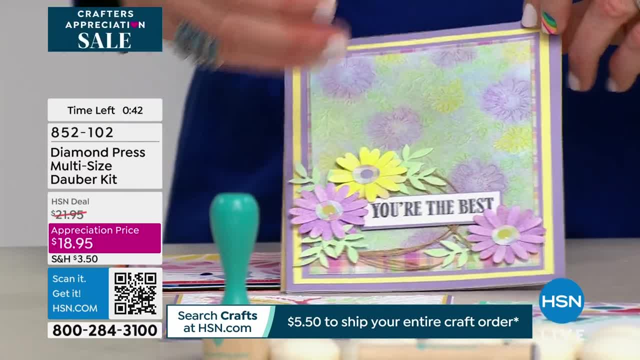 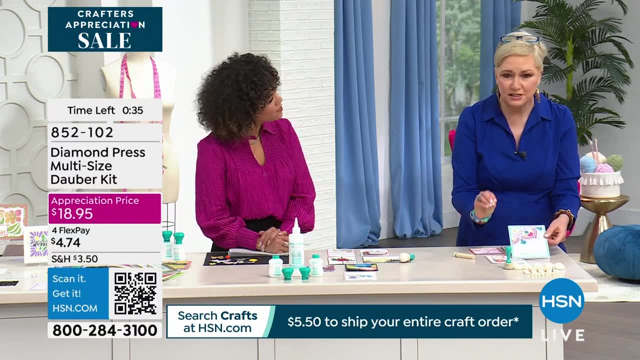 you want, because you're getting all three sizes and you're getting 10 of each. So that's what I think is so cool. And again, with the, I think we glued down the little tiny one. So I'll just take a little dauber. When you're using daubers this size, or you get a little tiny. that's how. 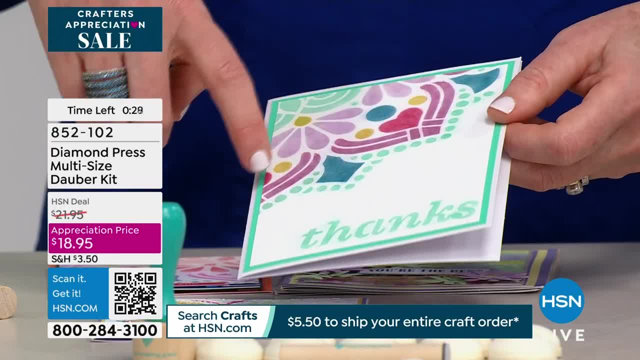 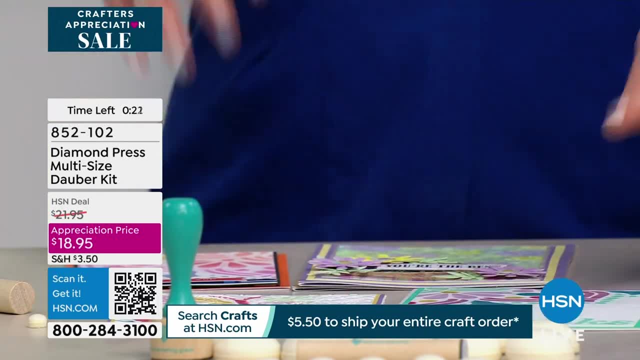 you can get, actually get these dots. So this, this design right here didn't have the dots. You can take them and add them in because you're doing this. So every possible kind of detail, from adding extra color to adding an extra layer, you can do that with this. that it's techniques. you. 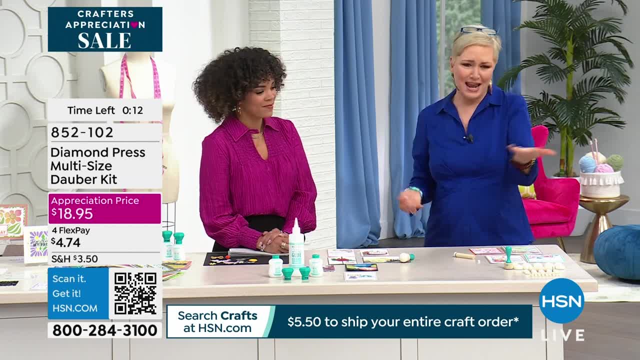 already know how to do. You just didn't have the tools to do it Right. And this now for 1895.. I mean, that's all right, That's math. So that's like what is that? Five, five, 50 of size? I mean. 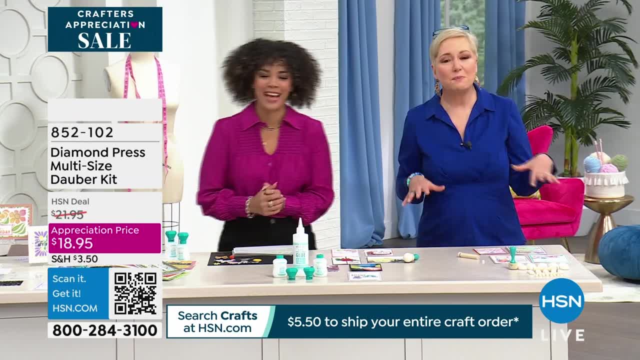 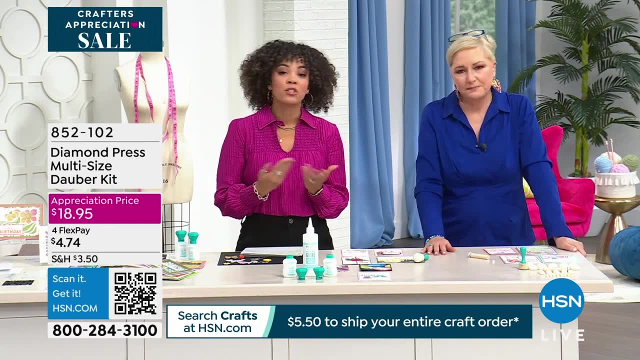 that's. that's incredible. That's pretty close. Yeah, that's pretty close. They don't pay us to do math here, They pay us to do crafts, but it's such a great deal because you'd pay $10. It's just for the large set. Well, especially now that it's back in stock, and now it's at that. 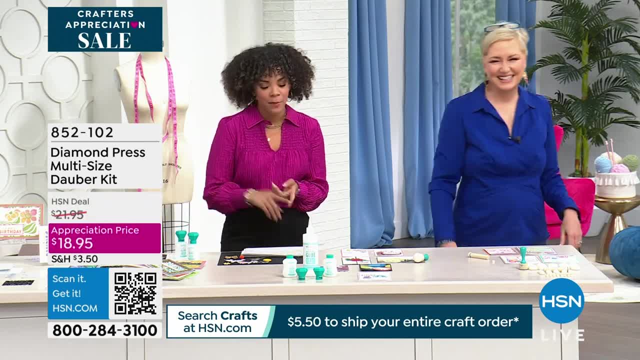 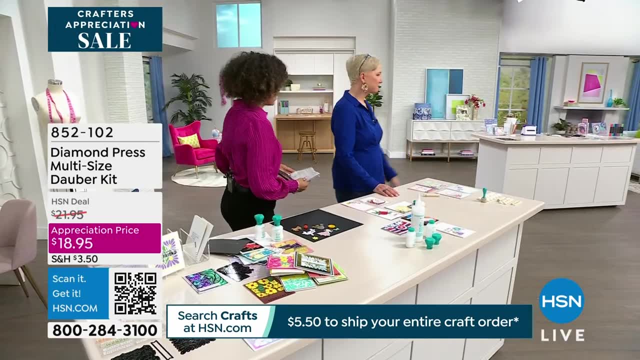 price. So if you want to grab it, eight, five, two, one zero two. So I've never keyed into hsncom or your HSN app. Okay, Really quickly. Oh, we're going, we're going to the left, We are moving. 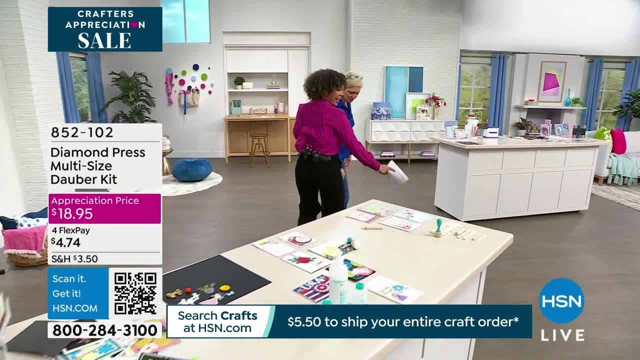 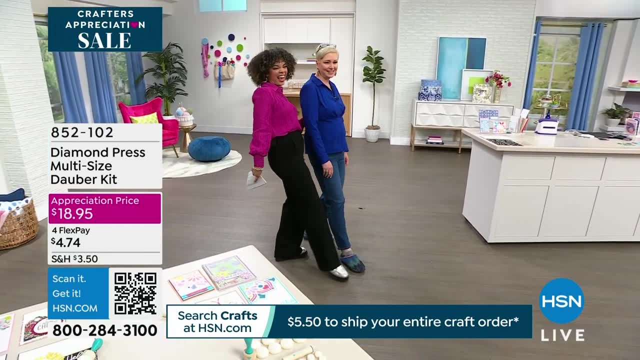 in the hallway, Nicole, she's wearing these like amazing shiny shoes and I'm wearing these slippers. And she was like, are you changing out of those? And I was like, no, I honestly, I would love to be in slippers right now. 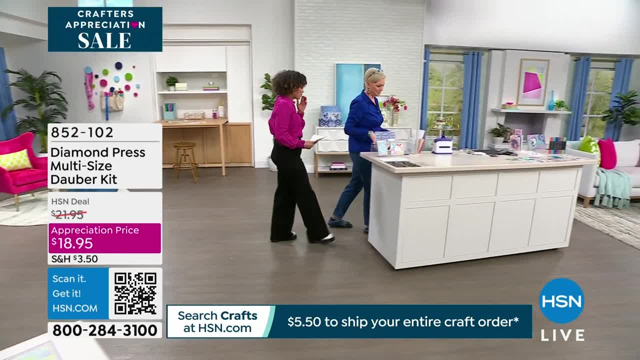 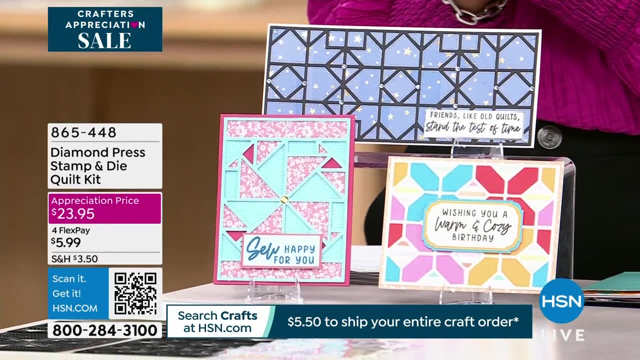 I just can't. I would love that, I just can't I. when you have to stand up for 14 hours, I was like I love you but no, I will not be changing out of that. That is okay. You come as. 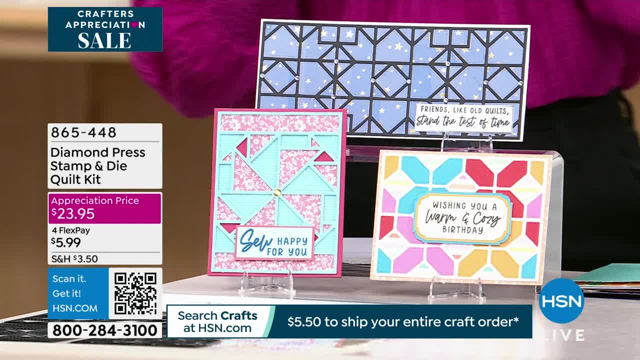 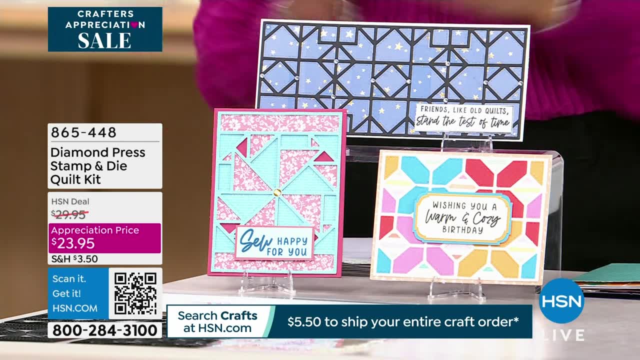 you are. That's how we want it to be here, Especially whenever you're crafting. this is something that's supposed to be, you know, therapeutic for you, relaxing for you, And you get the shot for the comfort of your home. That's what's great about HSN. Okay, What are 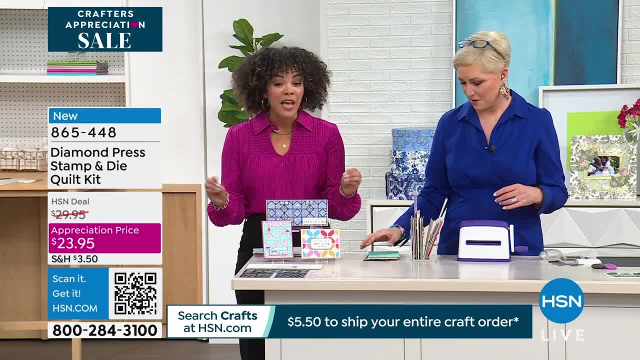 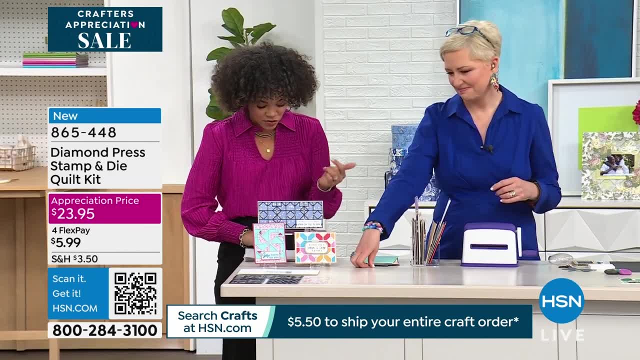 we talking about from diamond press brand new again stamp and dye quilt kit. Yes, Beth has been so excited to show this to you, So get your stamps. You're done. You'll get some blank folders, the adhesive sheets that you need, everything that you. 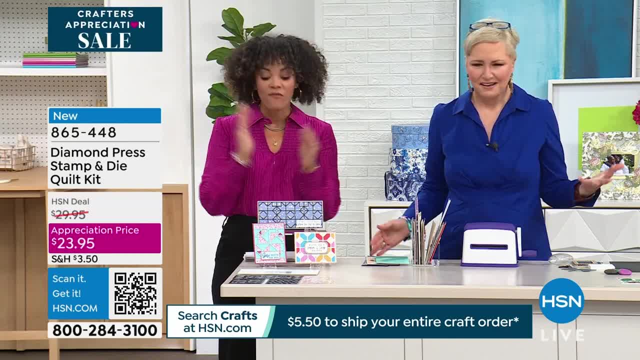 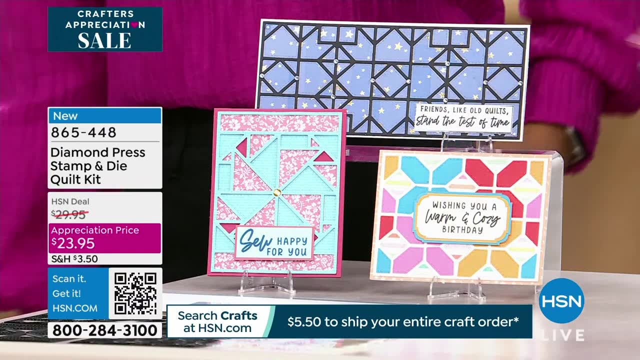 need, at appreciation price at 2395.. So run, don't walk to this deal. And this is brand new today, Like this, is a launch event right now, So I'm going to show you what you're getting and then I'm going to completely disassemble it, Cause I need to use it to. 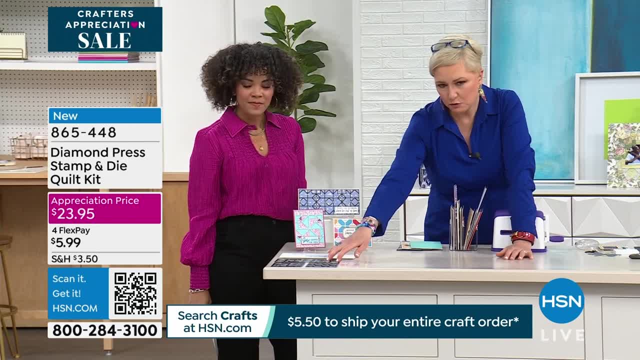 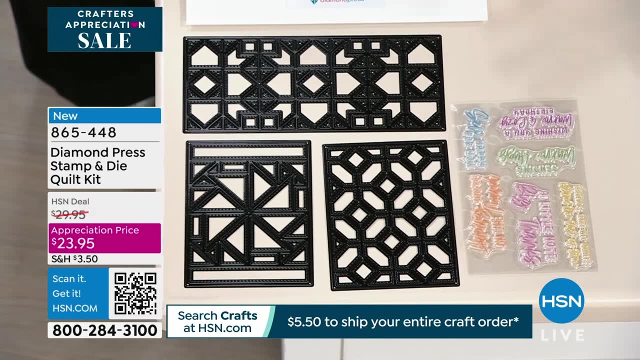 demo juice you Okay. So you're getting these three. you're getting a slimline quilt dye and you're getting to what we call a two size quilt dyes. You're getting a full sheet of stamps that have these really fun sentiments I'm going to talk to you about. you're getting 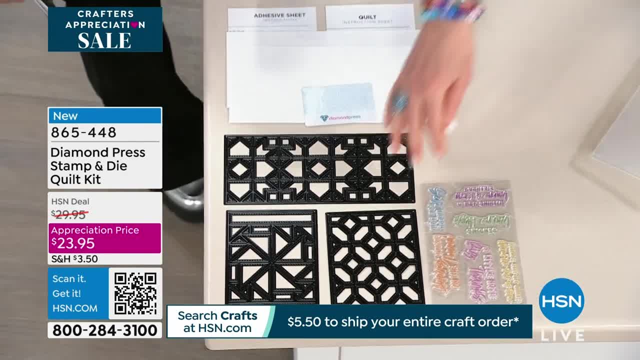 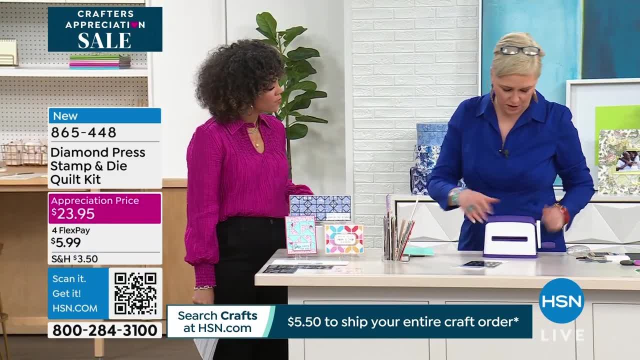 two adhesive sheets. You're getting this folder Which I am going to use momentarily. So what does this mean? Everybody, I think we all- know what a quilt is, So, but you might not know how to create a quilted card. So I'm 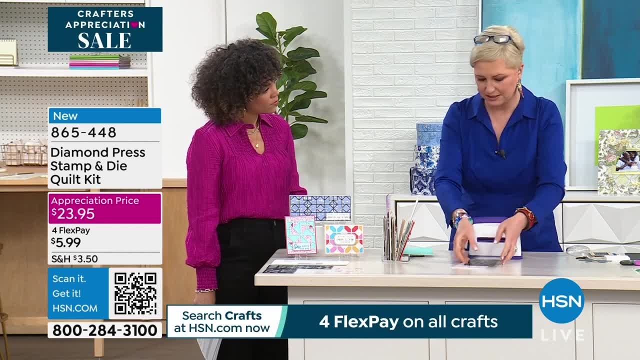 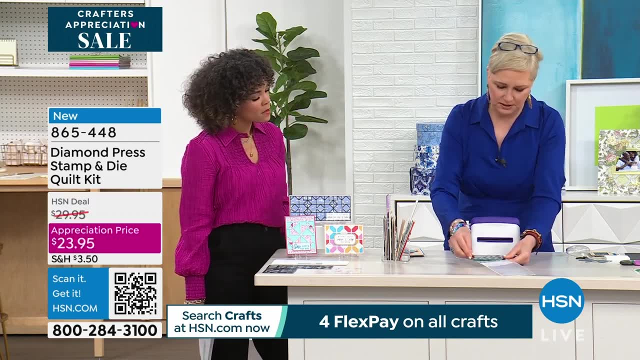 going to take. this is my diamond press machine And I think we have some marquees back in stock, maybe for the first time in like a bajillion years, So that might be that's a nice little tip. So I'm just going to take a piece of card stock. I'm going to lay it in my diamond. 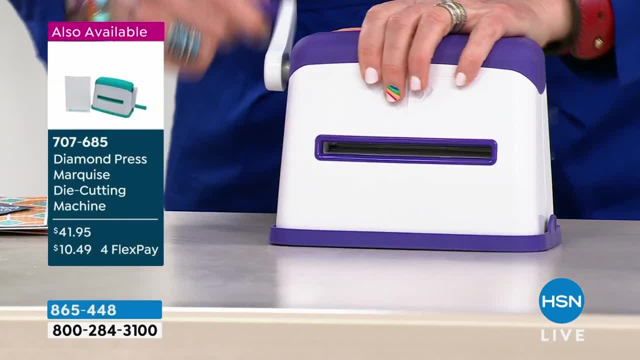 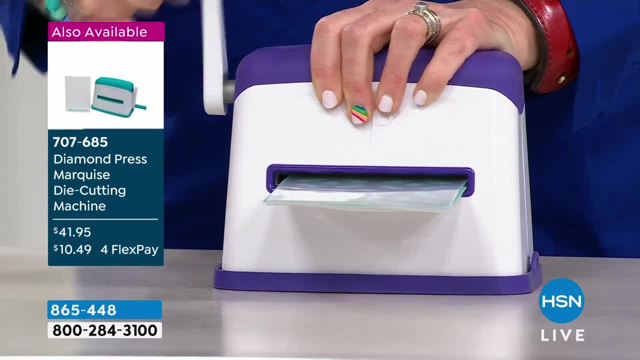 press folder and I'm going to run it through here. Um, so it comes with, here we go, We're turning or turning. We've got a machine right there from diamond press: 7 0, 7, 6, 8, 5.. 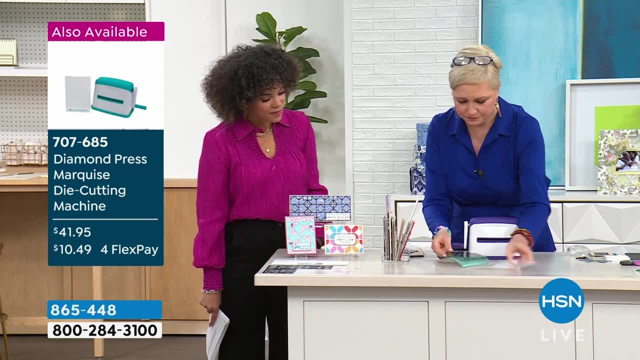 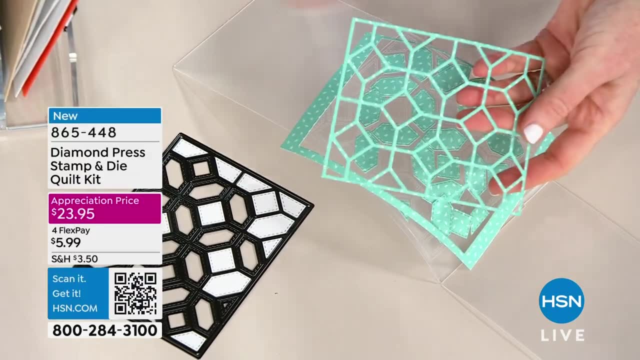 Also a lower price than we normally have, because of course it is Okay. So here's what's important. So this piece is going to come out and and what I love about diamond press is it just pops right out. You're not having to get a needle and like pick and poking, but then 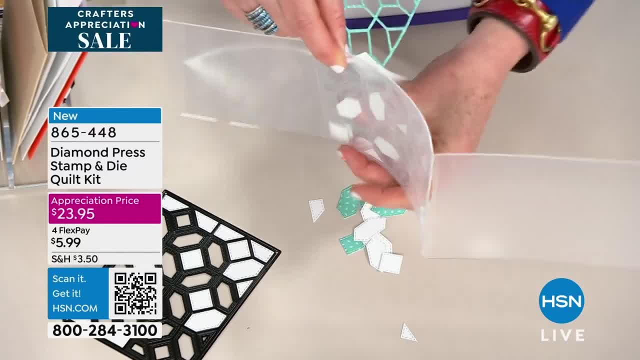 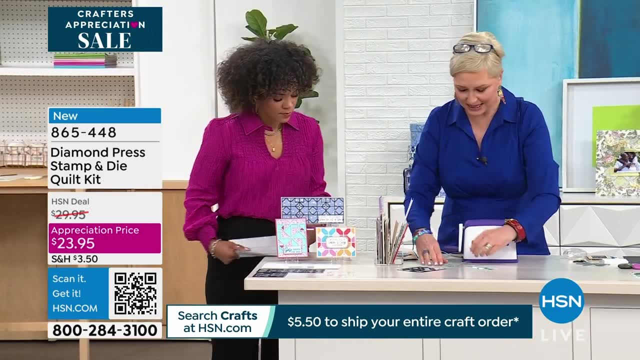 all of these other pieces and I'm not going to grab them all. All of these other pieces are coming out and you'd be able to be like, okay, but why do I care about that? Because you are going to use these pieces and these pieces to make these quilted cards. 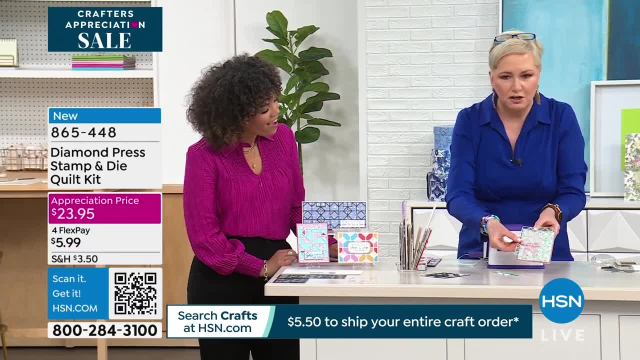 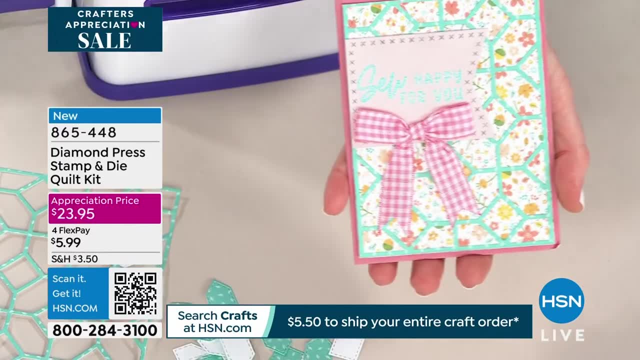 So you take the outside piece and you can make a card that looks like this, where you just lay it over and it still makes an absolutely beautiful color. Or you can take the inside pieces and you lay it over and you're making an actual quilted card. So I don't know how. 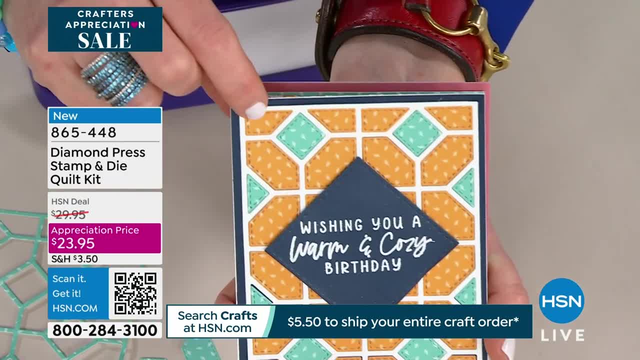 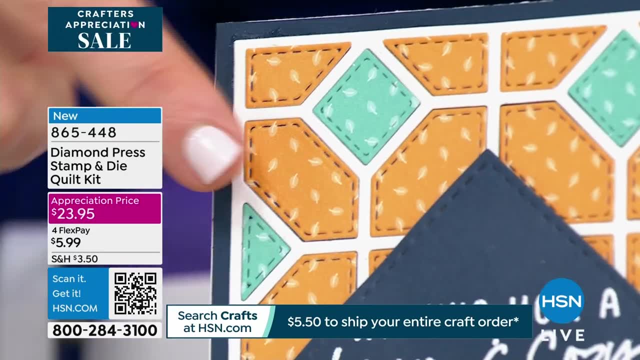 close. you guys can get in and see there are little quilts. Oh my gosh, you're so good. I know the team's amazing. Look at those on each individual piece. That's the quality of diamond press and that's the detail that you're going to get with this card, So look. 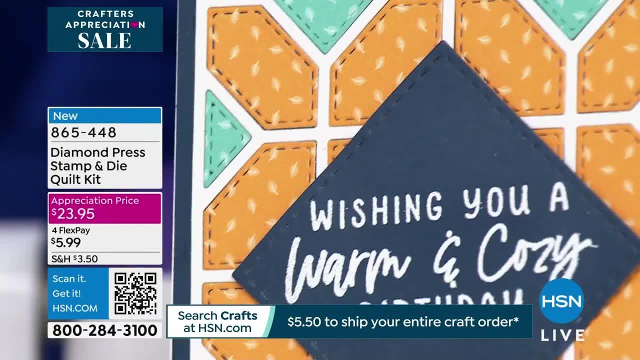 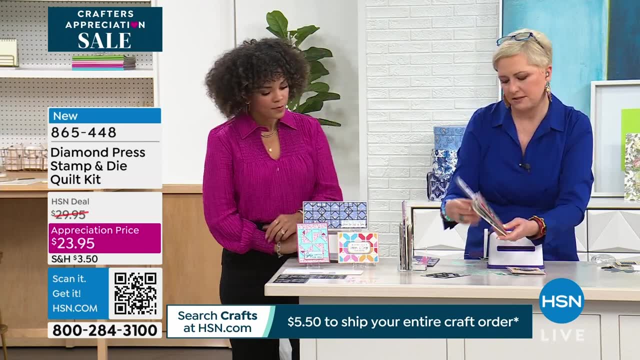 at these beautiful quilted cards that you're going to be able to make. And then you get sentiments like wishing you a warm and cozy birthday. Yeah, Aren't those so fun. Friends, like friends, like old quilts. Oh, my gosh, I'm going to put my glasses on. There we go. 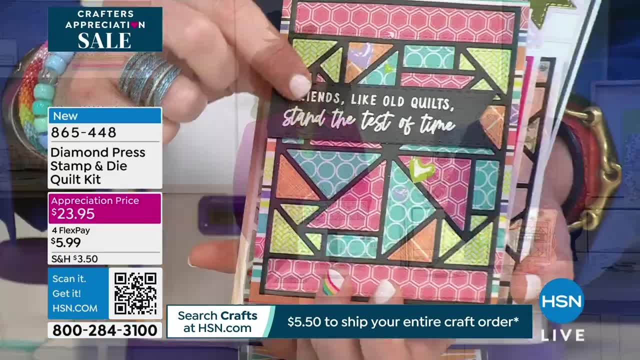 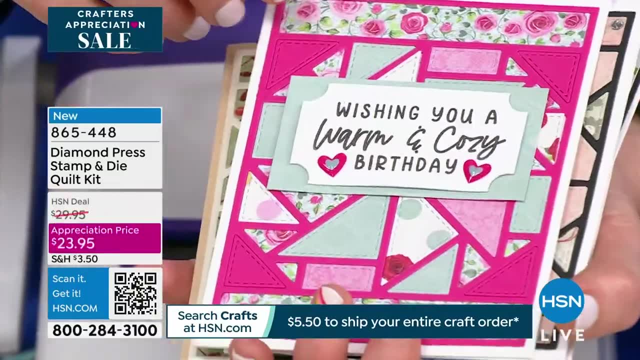 Friends, like old quilts to stand the test of time. but look at the details, And these are just with tiny scraps that you've cut out, maybe from other cards that you've been working on, Wishing you a warm and cozy birthday, sending warm hugs. So here's the, here's the. 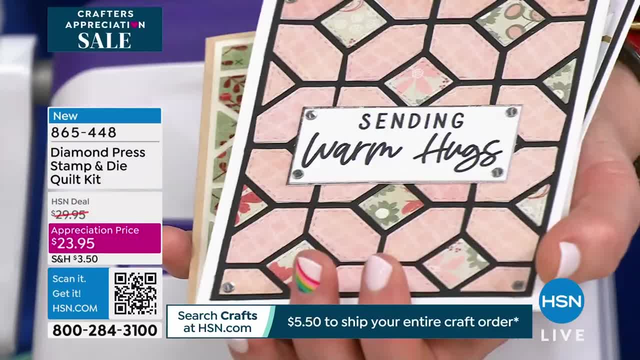 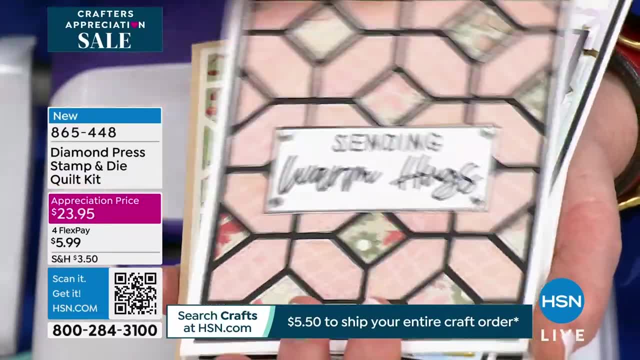 thing: If you're a beginning crafter- and I know I talk a lot about beginning crafters and advanced crafters because I want you to get sets that are going to work with you- So, sending warm hugs, you can do one where you just lay over the outline, like we showed with this. 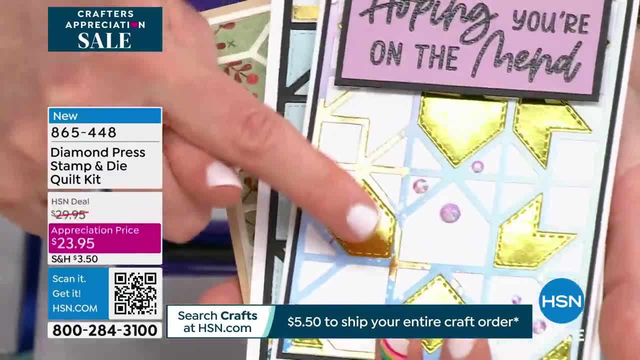 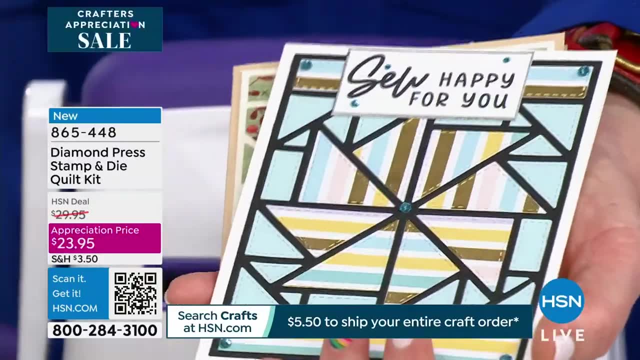 one, or you can do one where you add in the intricate pieces, though this hoping you're on the mend, So this set will grow with you. Everybody loves a quilt, whether you're someone, so happy for you, I mean. you know, I love a good pun around here. Um, a little note. 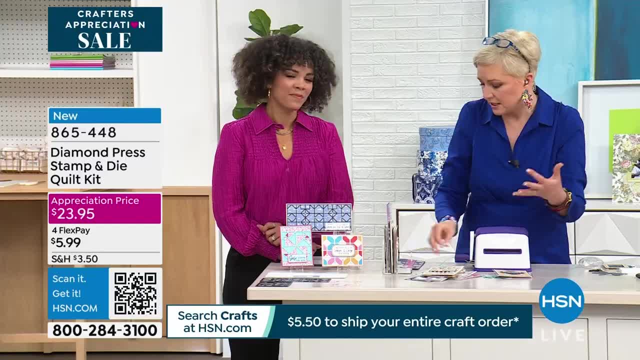 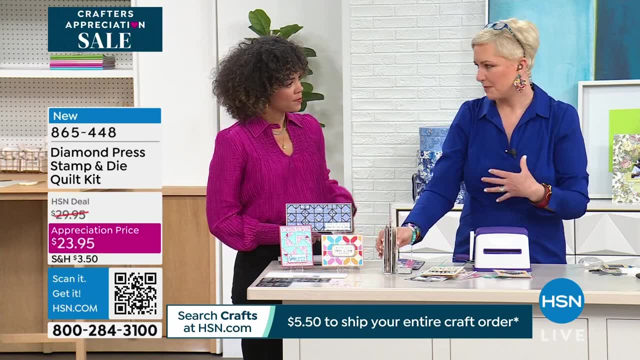 big thanks. So, whether you're someone who makes quilts- because that's a talent that you have, I think all of us, no matter our age, having, like my grandmother, made quilts when I was growing up- Um, my mom has quilts. 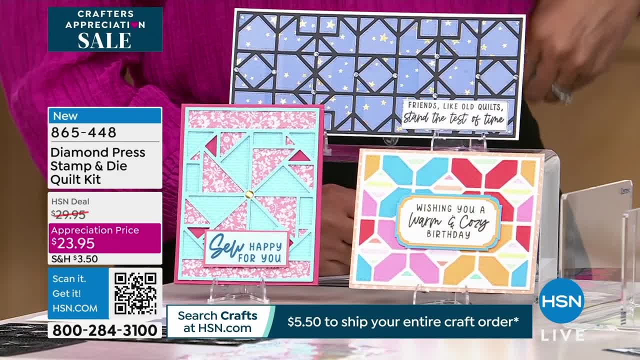 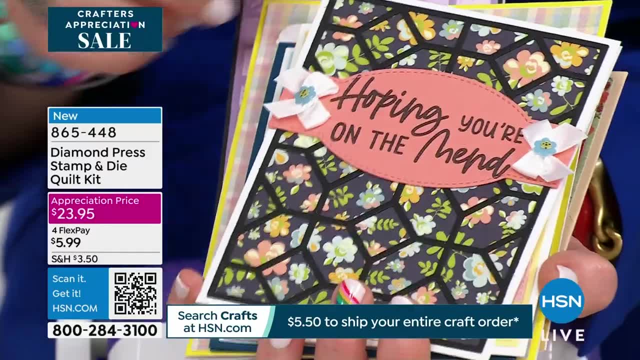 from her grandmother. Um, people are making baby quilts for their grand babies, So everybody has a quilt memory of some kind. It's just something that everyone treasures, and why not do that on paper? Why not create something beautiful that everyone is going to love? 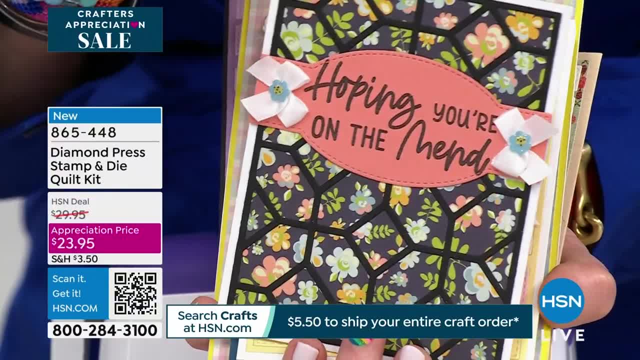 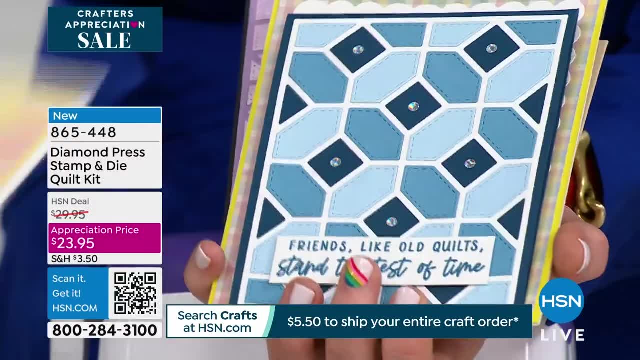 This is probably one of the most unique opportunities that I've seen too. I haven't seen a quilt set like this that we offer here at hsn. it's kind of far and few of what you see, and i love that. it brings back those great memories, that warmth that you know when times are just easy, just relaxing. 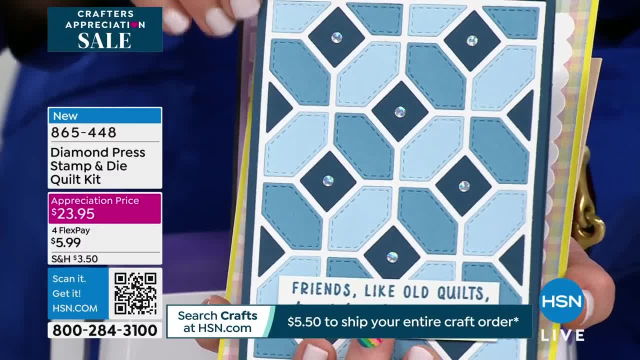 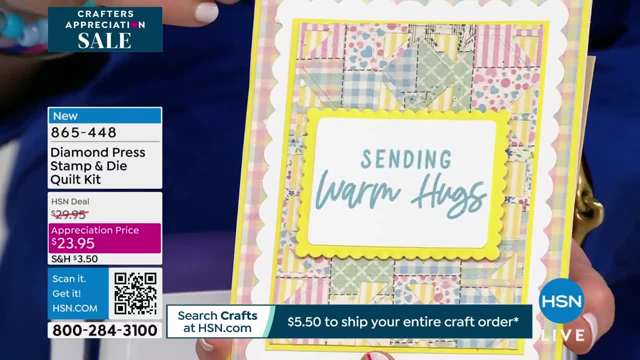 oh my gosh, yes, um, in front of a warm fire with a little cocoa? yeah, absolutely, and it can be celebratory, it can be comforting, it could be for sympathy, it could be for baby being born. i mean, it's just and you can mix and match the colors you want to use, the patterns you want to use. 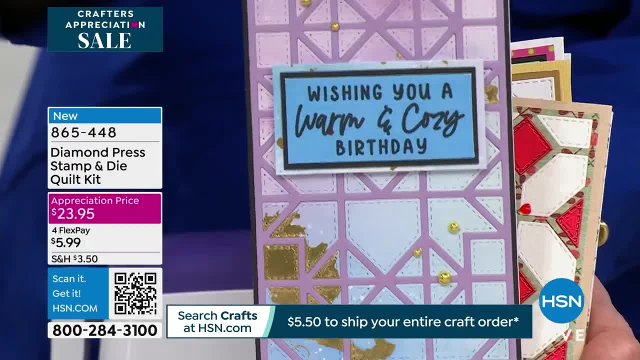 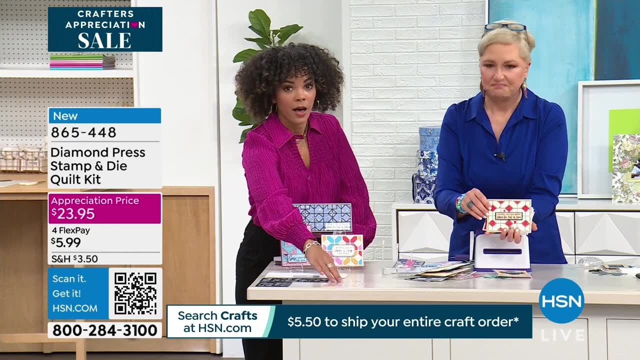 whatever scrap paper you've got at home, this is the set for you. i just love everything about it and these beautiful finished projects. i love that, and remember the stamps that you get. there's six of them that come, so you'll have all those beautiful sentiments, which is really nice. 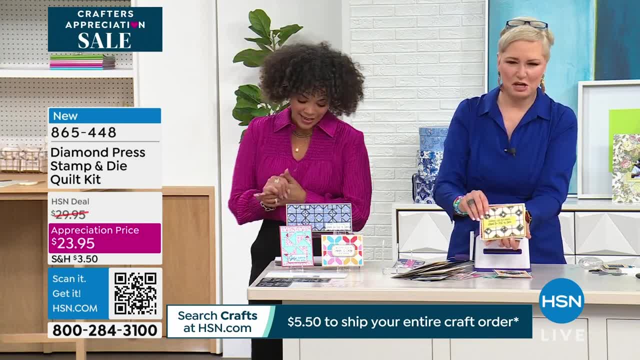 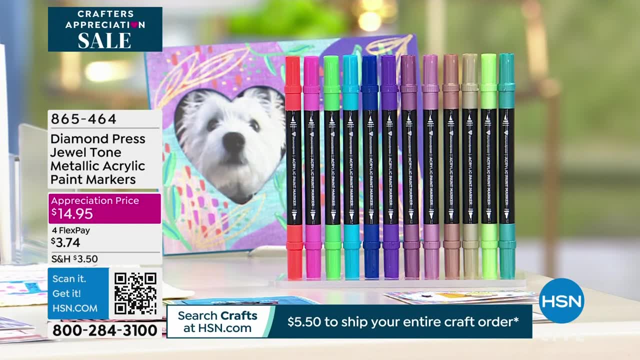 all right if you want to go ahead and grab that brand new eight, six, five, four, four. eight is the item number on that. one has been very popular, so make sure you're dropping stuff on the ground up your cart and check out. okay, moving things along. i'm really excited about this. i am a sucker. 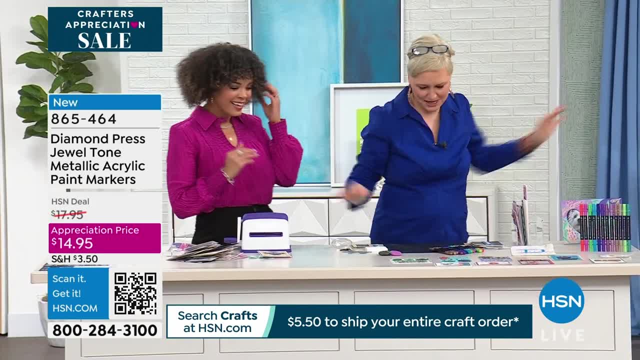 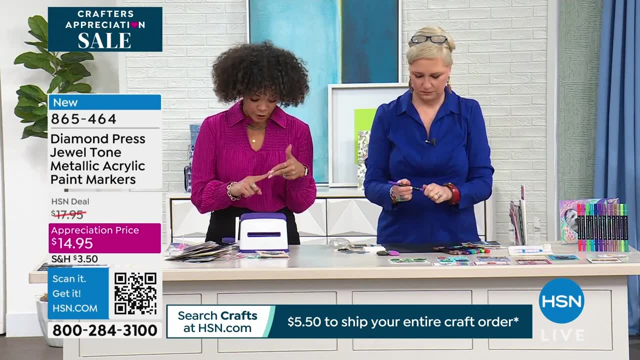 for, like, beautiful markers. i feel like i need to know why, like it's spread out the table because, see, things are about to get amazing. so here's the thing you're going to get: jewel tone metallic acrylic, acrylic paint markers. you're getting 12 of them and they're. are they dual ended? yes, 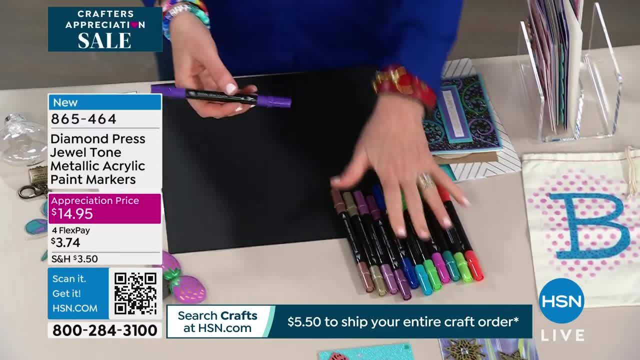 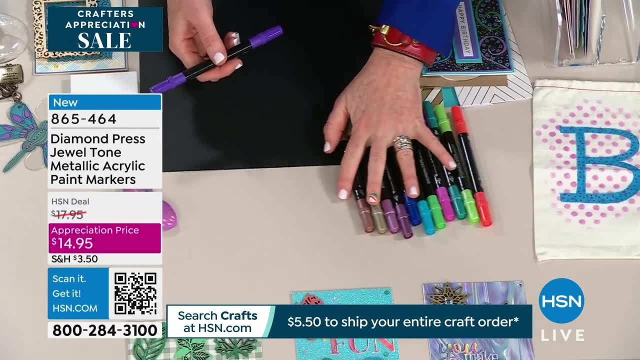 different tips, which i like, a different kit and you get some. we've got them set up. i hear what you're getting, but you get brights, you also get metallic, so it's an amazing mix and match. so if you have never seen our acrylic paint markers before, um, every color we've ever had. 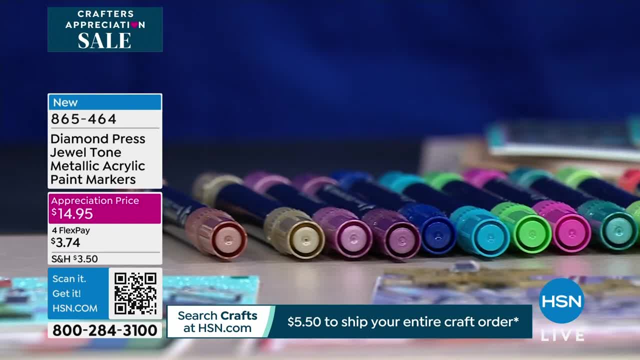 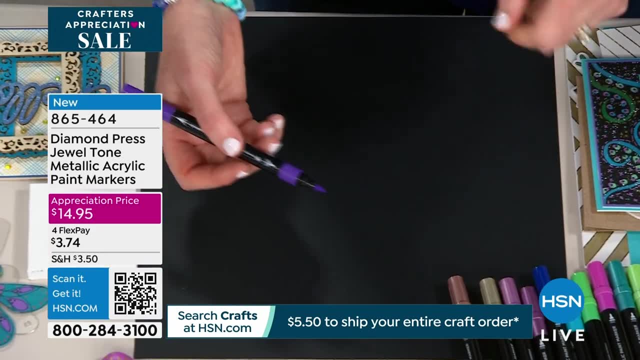 has been a customer pick, and they sell it like crazy. what makes them so special, it's the materials they work on and the saturation of color. so, oh, we've got this nice piece of black cardstock, okay, great, go get some of the pens you've already got at home and see if they will do this, because 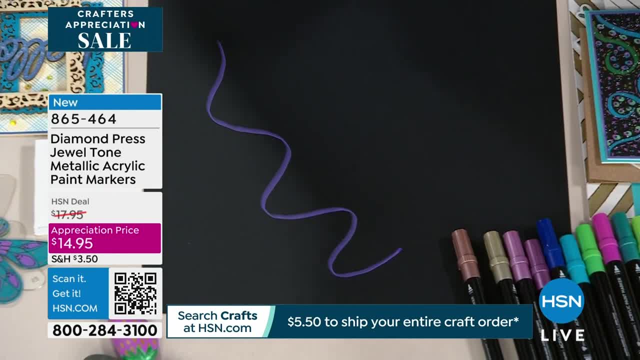 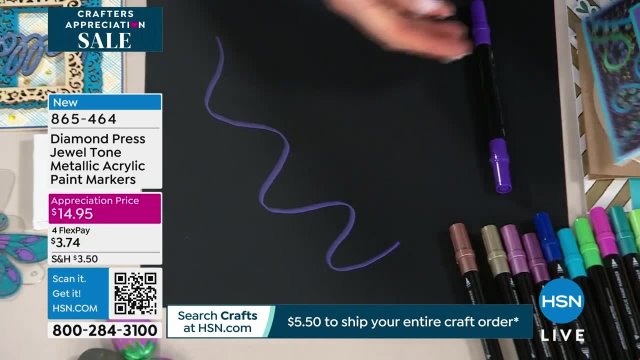 look, look at what happens on that black. you're right, usually it blends in. it usually blends in that you can't even tell the right, you can't tell the color. so you're turning a piece of black cardstock into something. i'll turn it around. there we go. am i right side up, upside down. 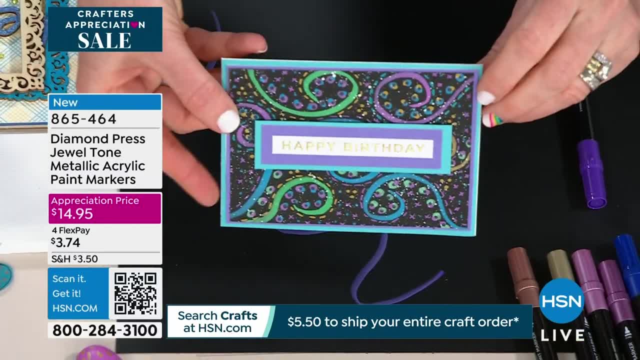 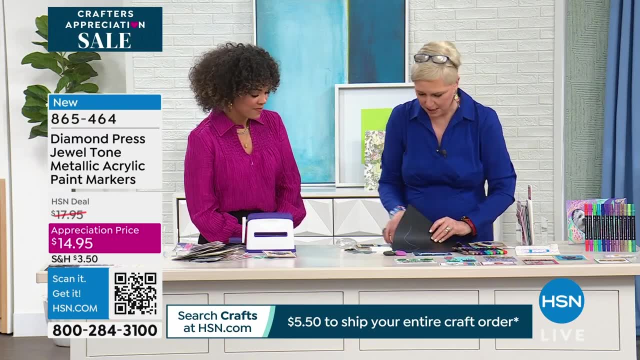 look, look at how stunning that is. just little tiny. if you're somebody that loves to doodle, if you're kids in your life that love to do crafts, it's just the most amazing thing ever. okay, so now we start out. we've done on black cardstock. i'm just gonna make a mess everywhere. all right, now let's try. 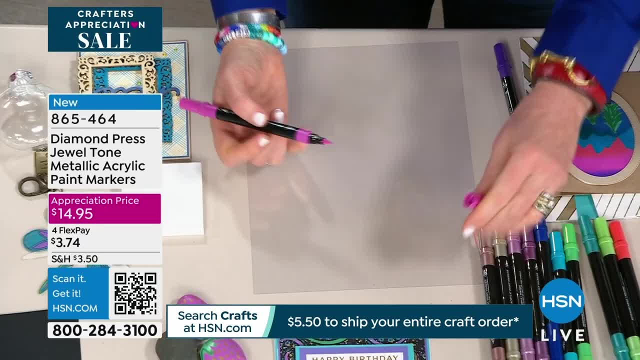 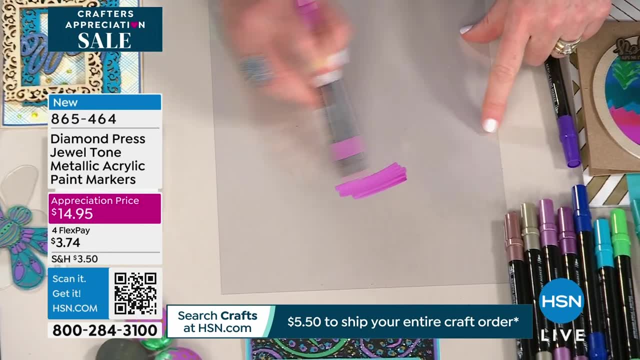 so this is acetate, right, and acetate is something that you get with a lot of kits and um or you can. it comes with packaging and you're thinking there's no way this marker is gonna, because look, look at the coverage, look at the bright color, look at this finished card. this is gonna. 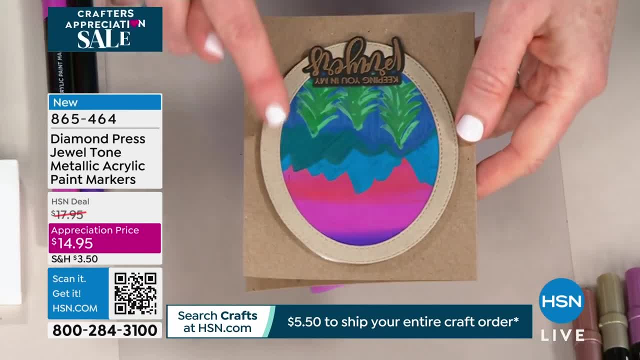 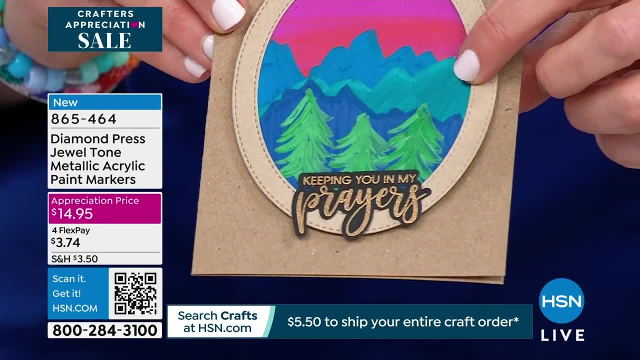 blow your mind. this is on, this is acetate. so this is like looking outside of a mirror: look at, look at that and then look at the like shimmery, oh, the metallic right there. i mean, come on, even with that there, you can see, right there, the shiny. that's how you can tell. 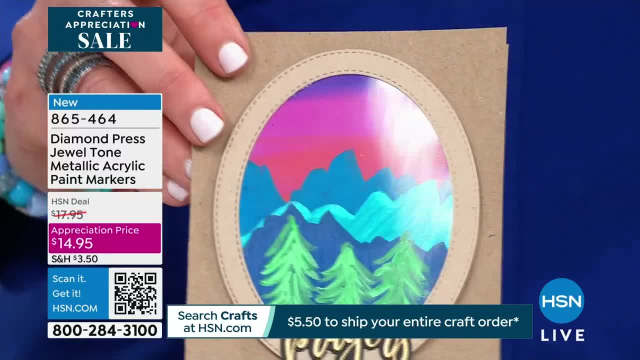 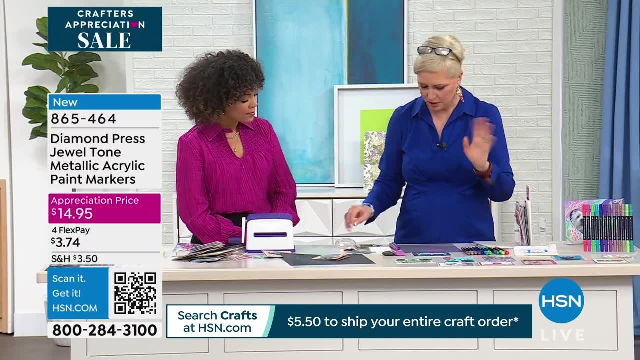 it's acetate. look at the saturation of color. so if you are someone that has always wanted to try these different techniques and you're like i don't have the right kind of markers, i don't have all right, okay, so we'll go back to crafting or scrapbooking, card making, whatever in a minute. 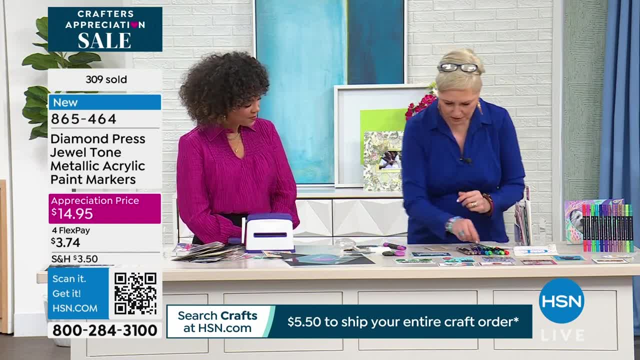 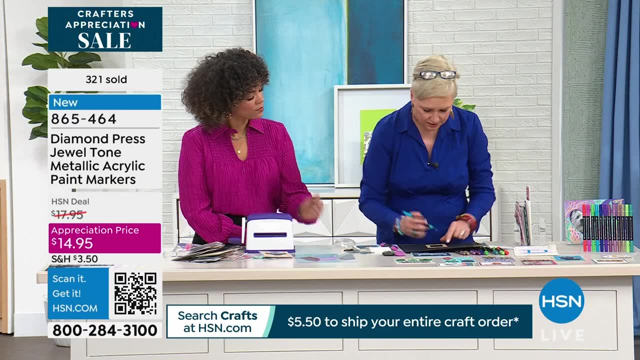 okay, let's talk about what else you can do. um, how about wood? everybody, let's color on some wood. so whether you like to do, we'll do it over here. whether you like to do um projects like for your cards, whether you like to look, look, it's like it's painting, the color payoff you get and look. 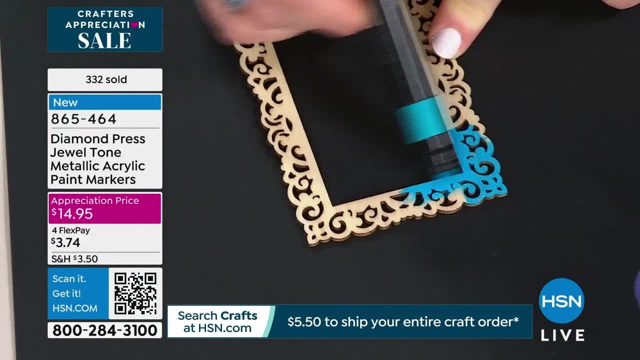 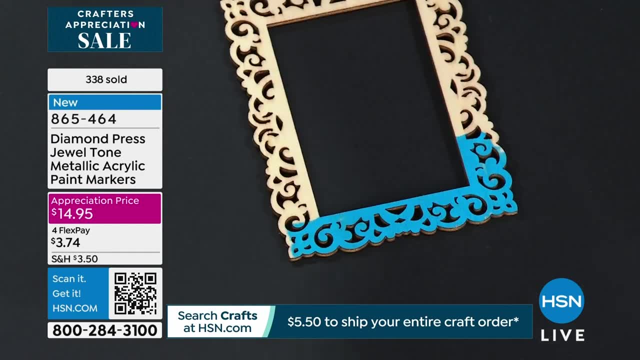 at how beautiful that is. so we have all been those people that we go to the craft store and they have like a bin of wood things that are like 10 cents and you're like, of course i'm going to use those. and then you get them home and you never do anything with them because you can color them. 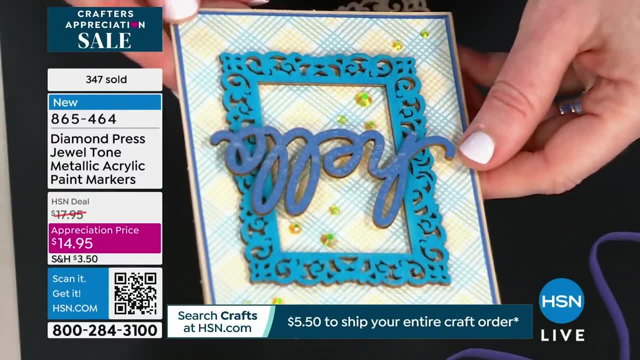 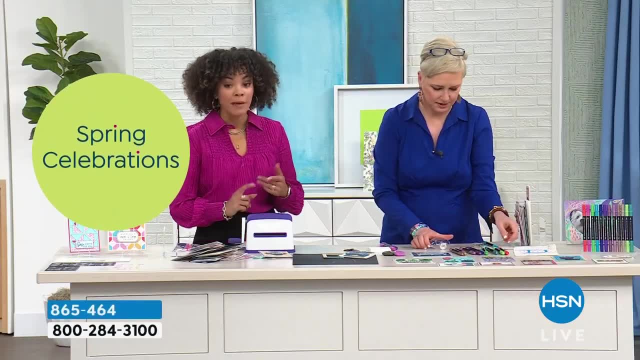 look at how stunning that just that added pop of color. okay, let's talk about what other kind of crafty fun things you can do with these things. so let's talk about what other kind of crafty fun you can do, and feel free. please jump in at any moment because i know we're getting busy in the 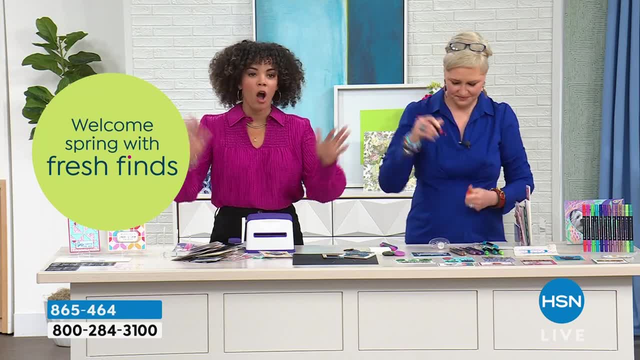 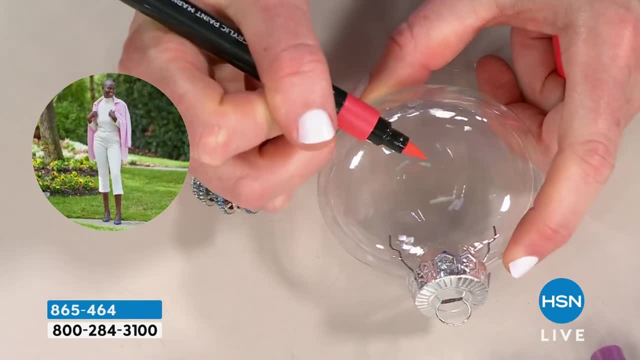 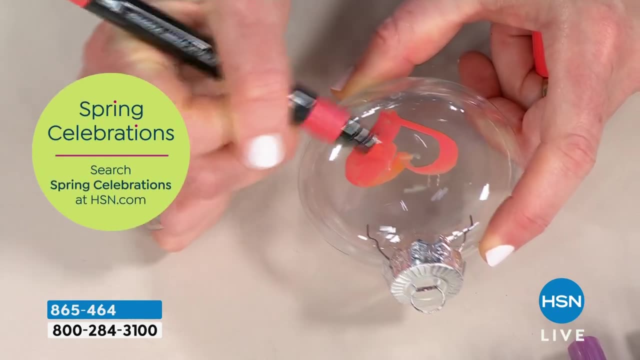 ordering process. remember: load up your crafting car all day long, all on airs. crafting it's a 24 hour event. everything's on sale, by the way, and if you load up your cart for 550- well, nicole, i bought five things and then i checked out- was it? i have to pay the shipping again. nope, 550 all day, that's. 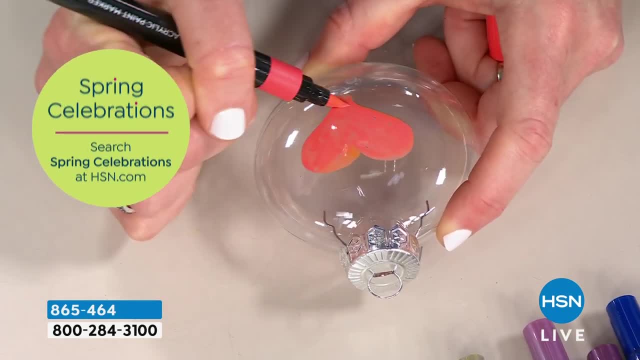 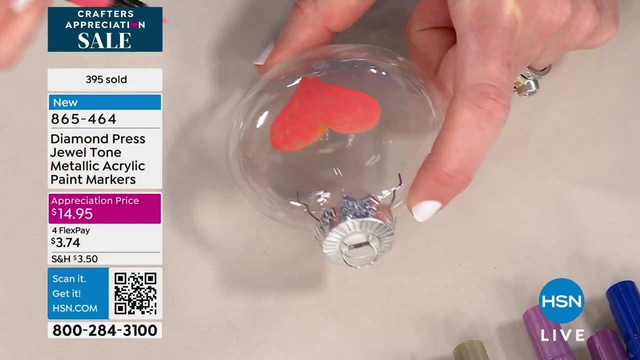 it just one time and then that's it. so if you want to grab it, 865-464 is that item number. now you're putting this on what? this is a plastic, this is a plastic ornament, but you could also put it on glass. so again, when the holidays come. 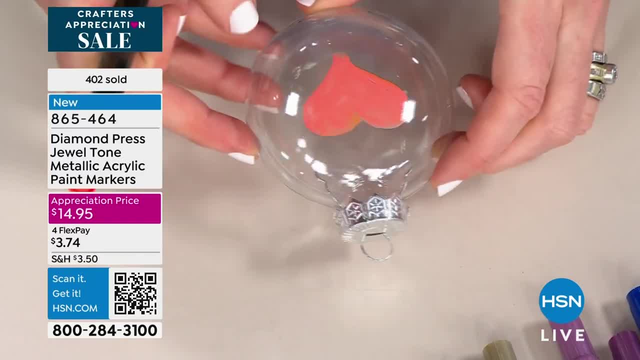 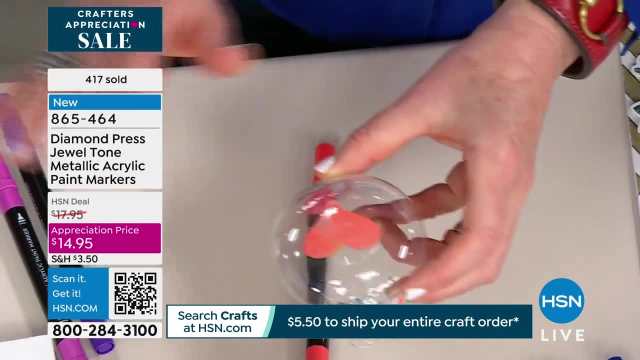 and you see those little kits and they're like make your own and you can look at. look at how beautifully that comes. how long would that take? the dry: you think it's dry already. oh, you won't touch it. i don't know, it's dry, it's a little dry already. okay, let's talk about what. 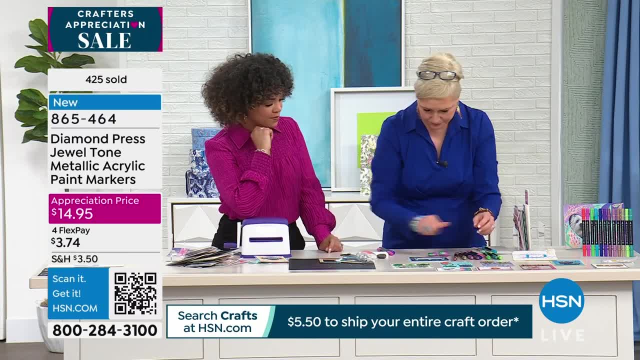 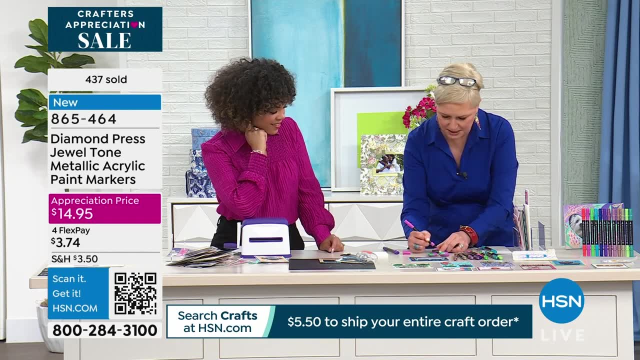 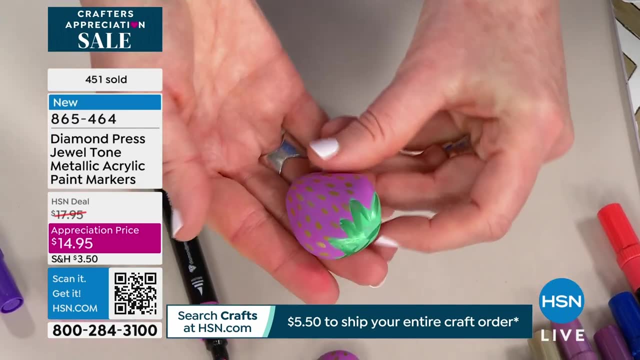 else, rock painting. oh okay, rock painting is very popular, so i'm gonna take my right, right, rock painting. so look, i'm painting with the rocks. okay, how fun it is. blah, blah, blah. you give it about you, and then you can add another color on top of it. look at the little strawberries. oh my gosh, look at. 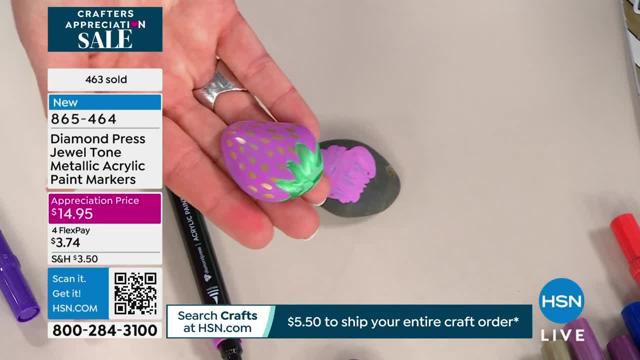 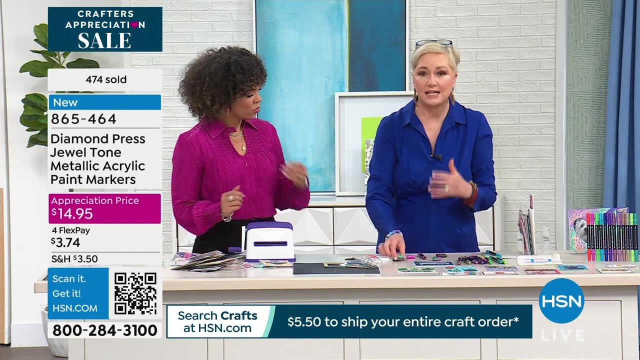 the little rock strawberries. so if you've got a child who loves to do all those projects that you see online- somebody- and they're like, oh, mom, can we try this? mom, can we try that? and you're like, no, because it uses paint and i don't want to make a mess, these markers are for you. if you've got an 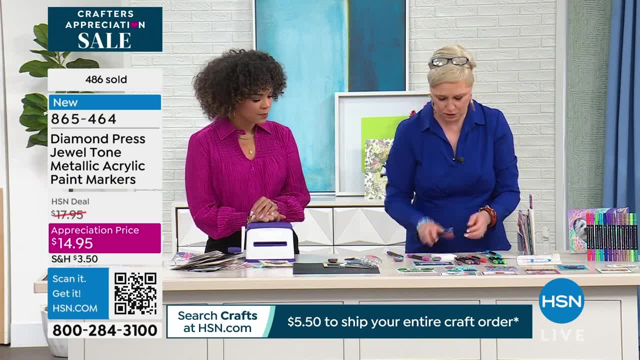 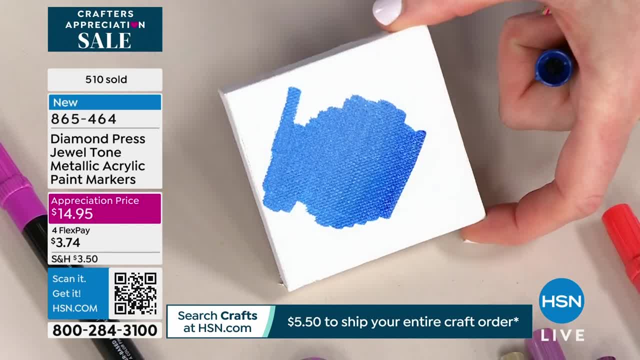 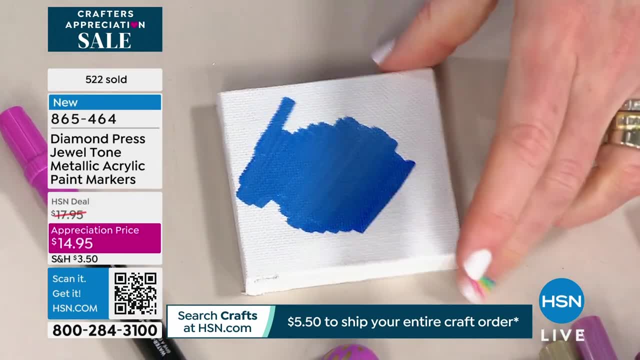 how deeply that saturates on the can, is that not? it's like, wow, i know, is this not the most incredible thing ever interested? it's almost like it has depth to it, like i feel like it's way you're looking at when that light hits it, just right, shimmer of it, because some of this 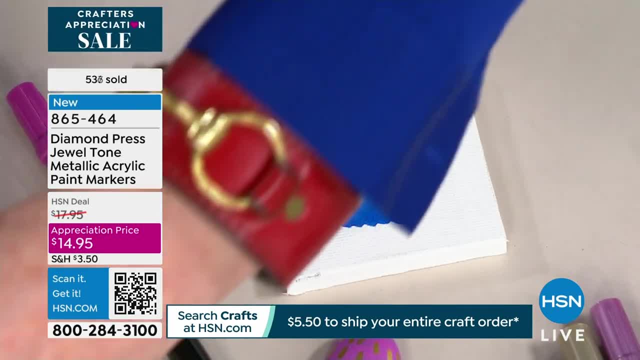 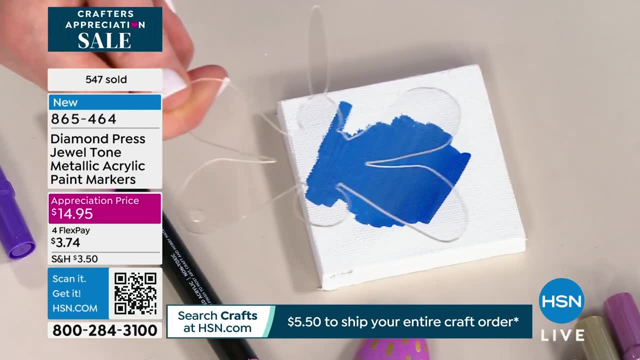 is metallic. okay again. and i talk about you know, things you can buy inexpensively at the craft store because we all do it right. you see these and you're like, okay, this is, i love this, i'm gonna do everything with this and i'm gonna make keychains for all my friends, but then you don't. 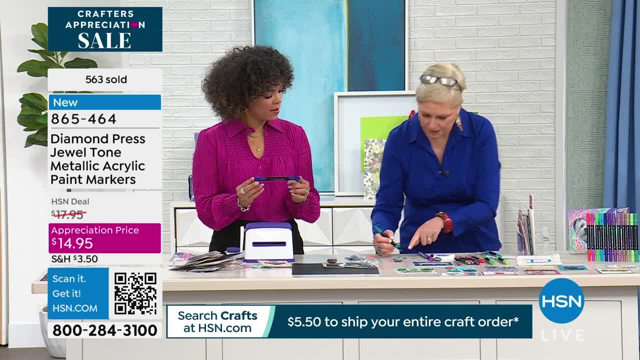 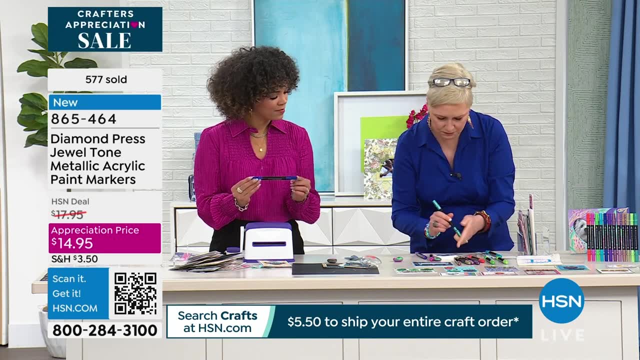 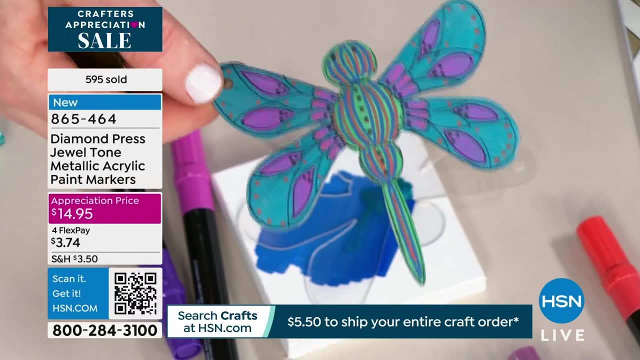 because you have too many things going on in your life. so look at how beautifully, oh, the wrong side hold on. look at how beautifully this takes the color and then watch what happens. watch, look at the finished result. oh, i love that. is that not? this probably costs five cents at a craft store. this little right acrylic thing, a random bucket that. 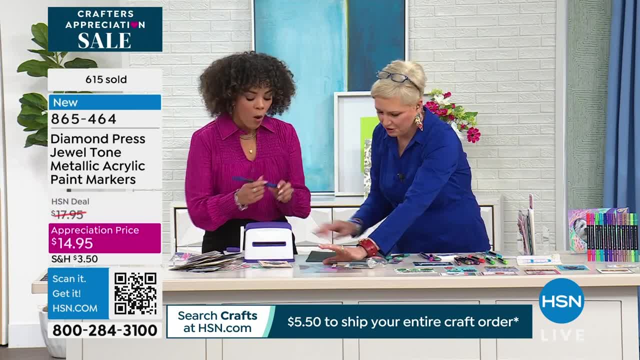 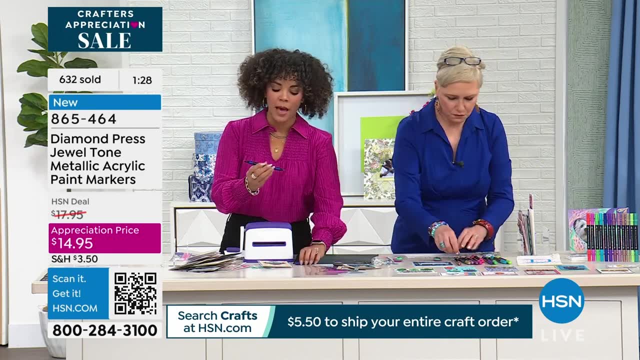 had everything that's on sound, which is great. i do want to draw on something. i do want to draw on something i also. what i love is that it's dual tip, so you saw beth using most of the brush, but there's also a fine tip, so i just wanted you to see that you want to do writing. 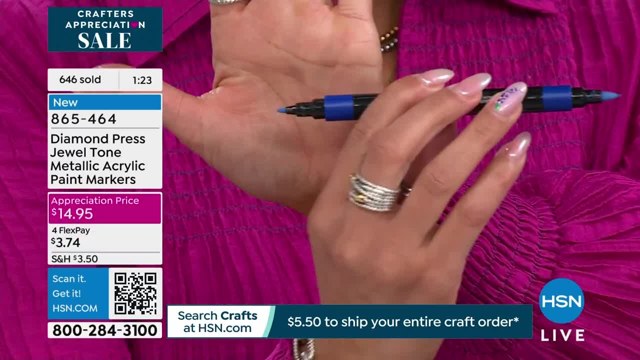 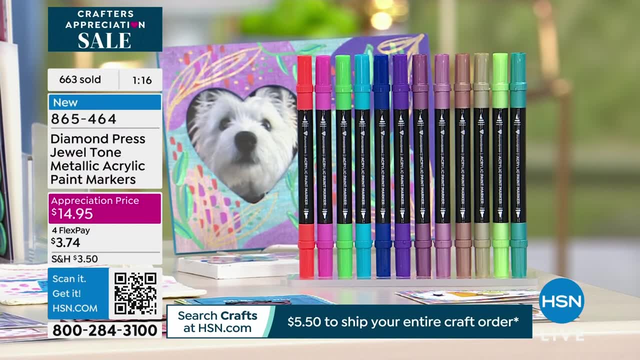 that's what's really great about it. so there's that fine tip that you see right there, and then there's your brush tip. so that's what i love. so you're getting 12 markers, but really it's like 24 opportunities in in 12, which is great. so it's double the amount. all those great colors i love. 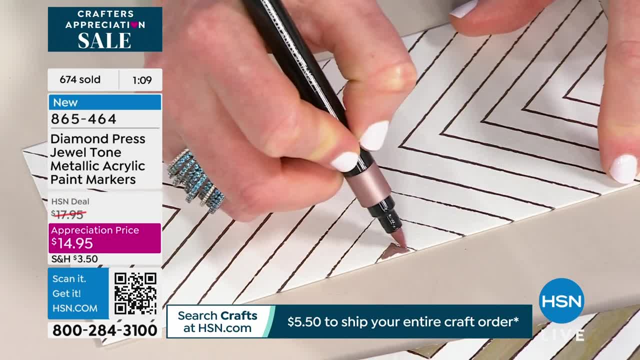 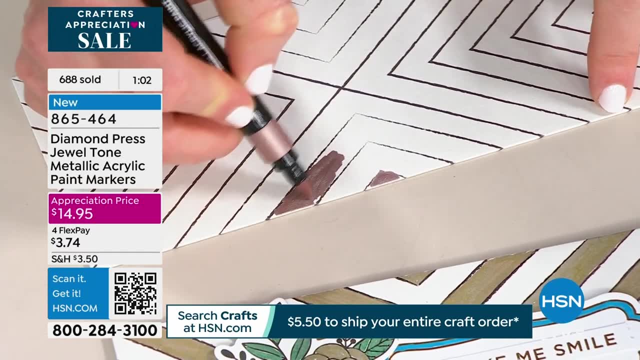 the brights that you get, but also the metallics that you get with this. feel free to jump in. well over 670, plus already gone. final 60 seconds to place your order. we added a little bit more time. it's 14.95. remember all crafting is on sale today that you're seeing on air. load up your cart. 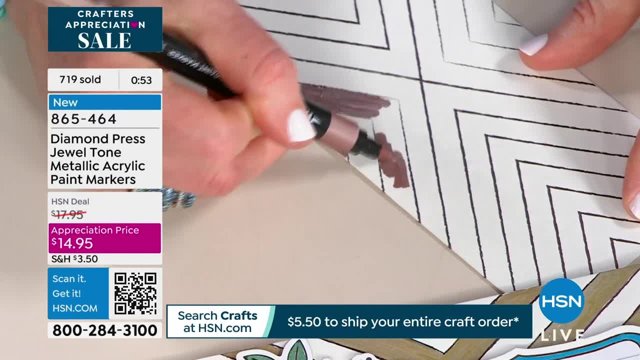 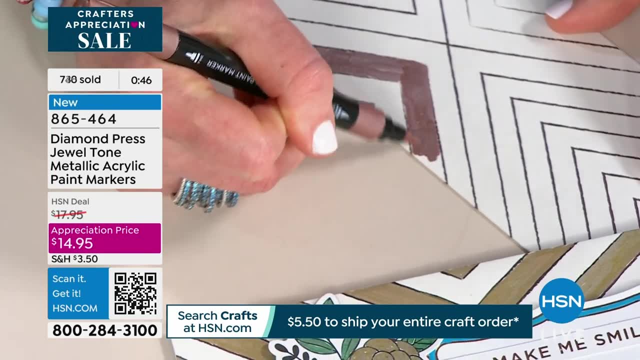 it's a flat shipping for all your crafting items. so even if you bought 10 things checked out, took advantage of the 550 shipping. when you add more, your cart is reflected that, hey, you already paid the five shifty, so that's all day long that you can do that. 865-464 is the item number, so i'm just 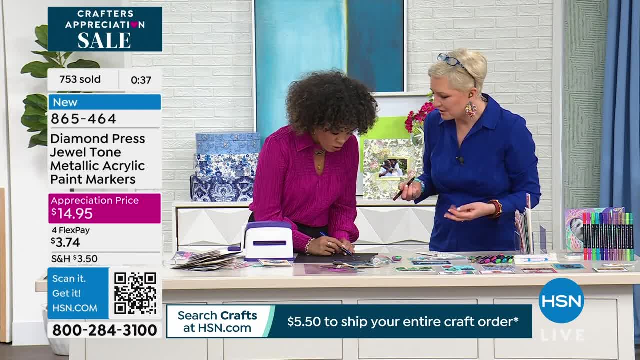 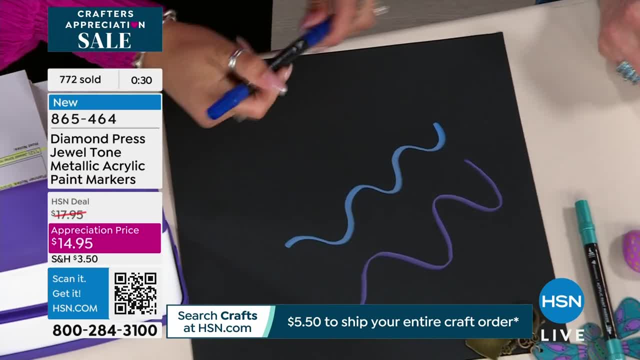 so impressed to try it. it's like it is so and it's soothing right because it goes on so smooth. because a lot of times you put marker on black paper and it doesn't come through, no, it just. but also look at how beautifully it comes through on white paper. so i don't want you to think, well, i can only use 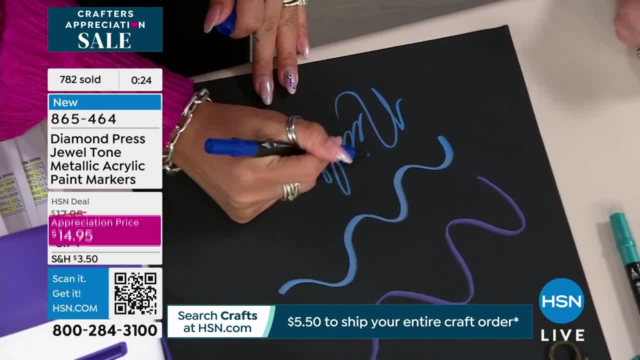 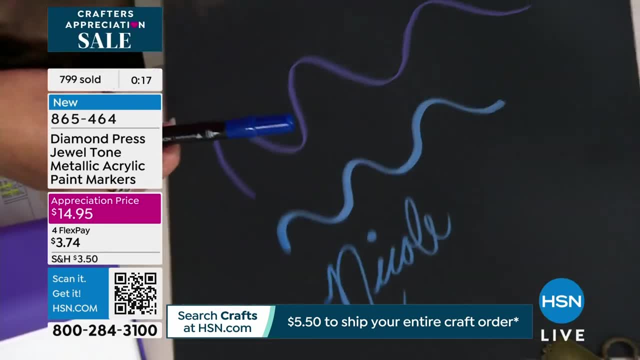 it on dark. so, yes, i've showed you a bunch of different craft ways you can do it. but for your card making, oh, i didn't even show all the finished projects because i was just so excited. oh, my gosh, a whole handful of finished projects. okay, just real quickly, i'll show the finish. yeah, hers. 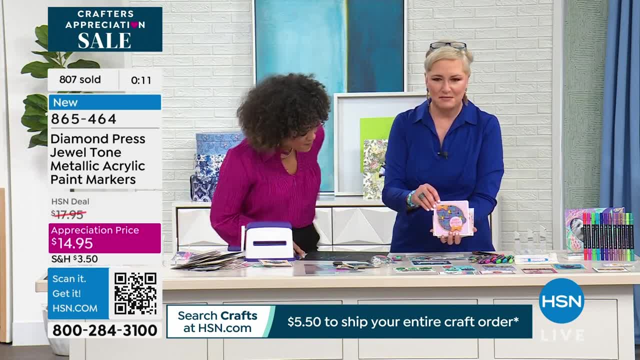 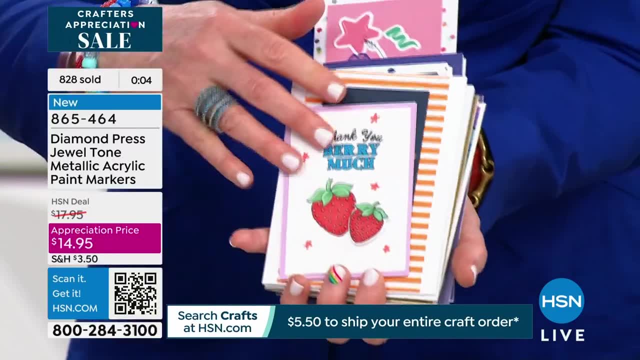 so like: look at these amazing finish, there we go. we're just these beautiful cards, i'll just go. so this is acetate, right, those little acetate, i mean it's just so much. they're like: no, beth, you're done, but so many great different cards you can do with it. but also the great craft supplies i mean. 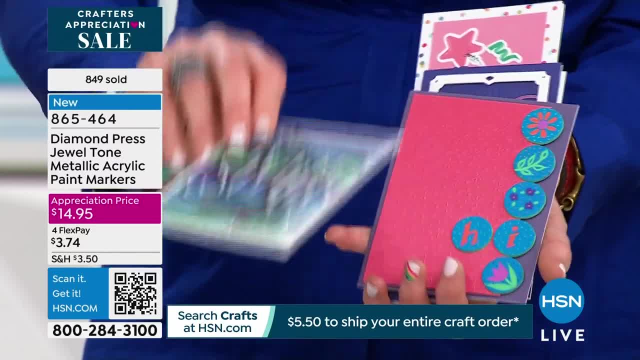 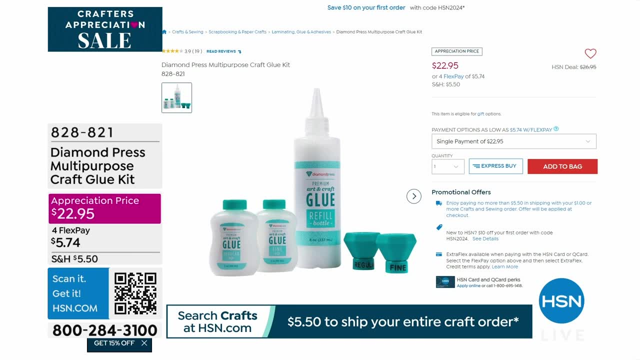 everything about it is stunning. uh, amazing cards, all right. um, almost 900 of those already gone. in case you missed it, very, very popular was over 600 gone of the multi-purpose craft glue kit. what's great about that is you're going to get two two ounce bottles with the glue. you're also going to get an eight ounce of the. 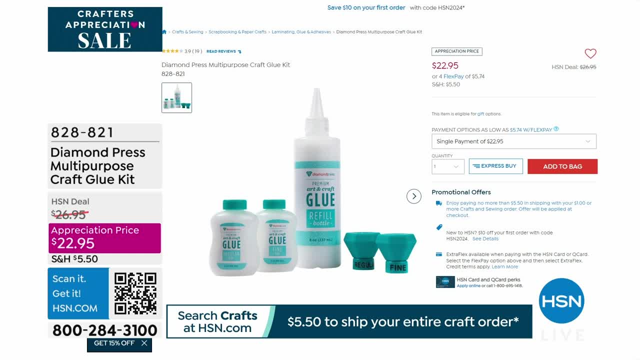 refill glue that you see in the middle, and then you get two tips: a regular and a fine tip. this a lot. what i love is beth was gluing on a bow a pom-pom, even those little things that quilting um set. if you pick up a few of those, you're going to get a few of those, and then you're going to get 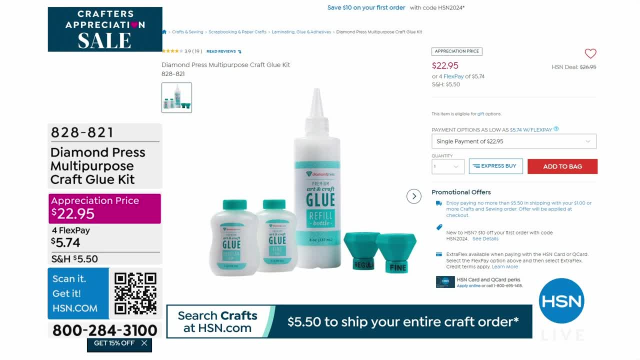 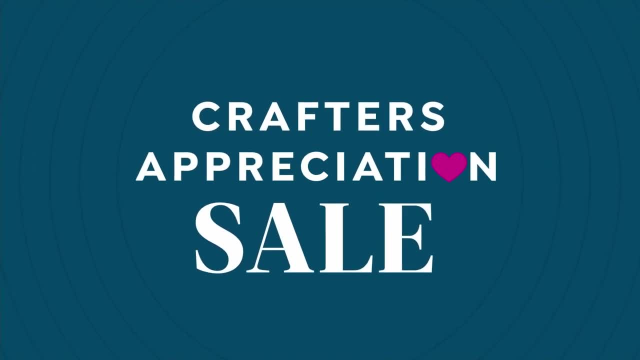 that off the little pieces? that would be perfect. use that for the little pieces. so you're going to use it on a variety of things. 828- 821 is the item number on that one. okay, moving on, as if it couldn't get more exciting. i, i just love, i love glitter, i love brightness and this is your neon glitter. 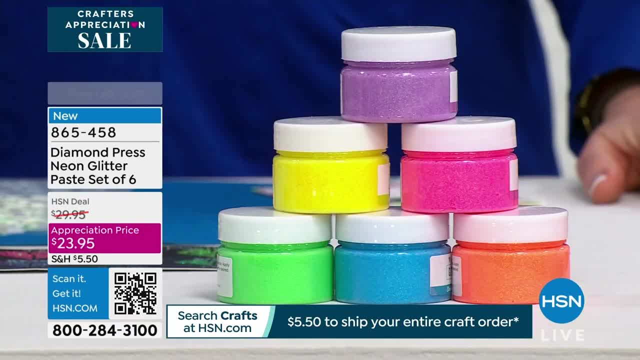 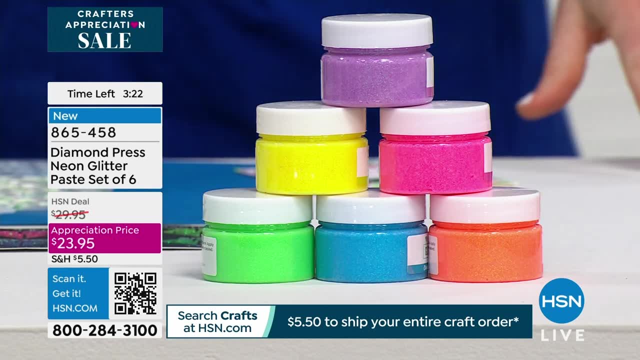 paste set so good of six. it's so good. there's all the colors that you get. they are stacked up so beautifully. does that not just say summer to you? it like it just says summer in a jar, summer, fun summer and a jar. i love that there. so you get six of them, all the colors you. 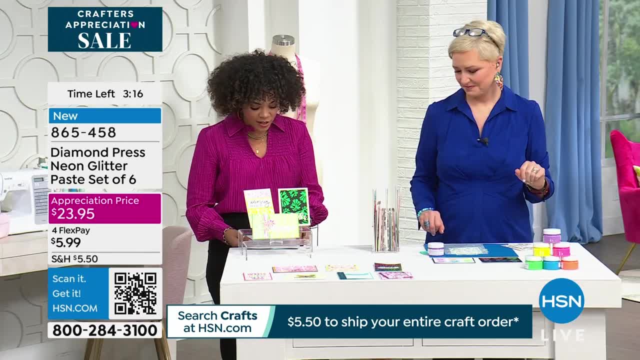 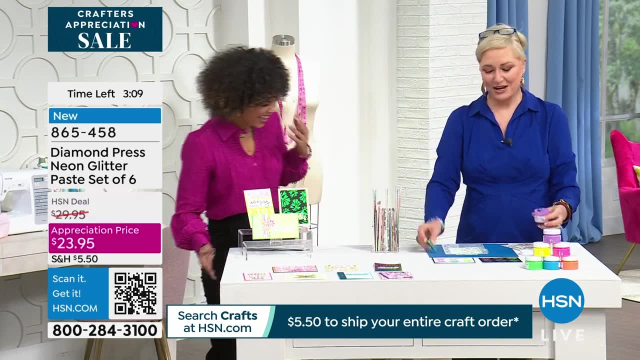 see, and they're 50 ml, so a good amount that you're getting for this. okay, show me how to use this. i'm so excited, okay. so, unlike the last demonstration, i will actually show you some finished projects, because i won't get so carried away, but so i really quickly do want to show you how it works. 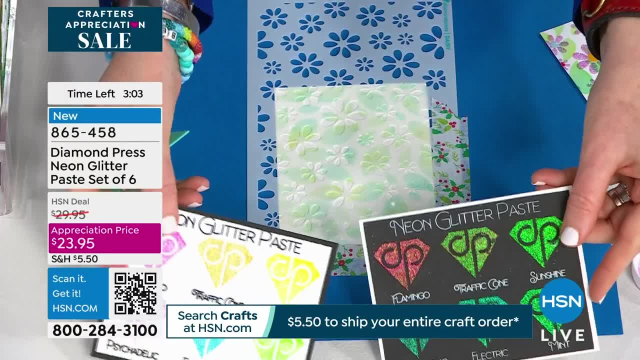 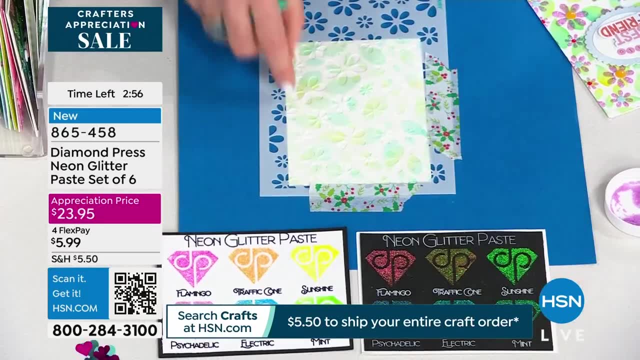 so this is actually a beautiful one of our designers put this together. this shows you what these colors look like on both white cards: dark and dark. look at how it glows on the dark. so this is how easy it is. we've all got stencils at home, right? we've all been making some fun. 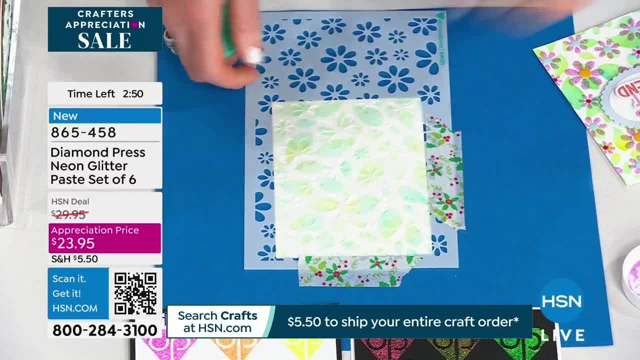 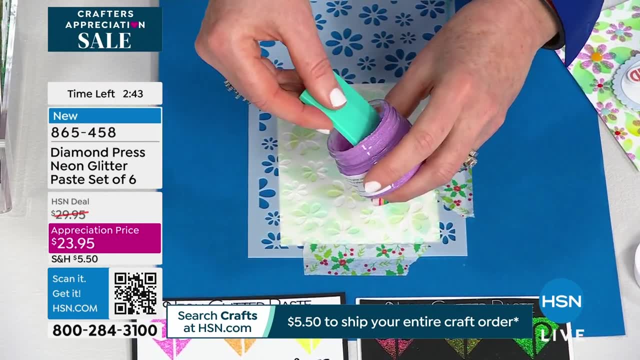 projects with our stencils, um. but so i've done a card. i've got a little bit of a little bit of pattern, i've laid the stencil on top and i just add a little bit of washi to hold it in place. i'm just going to take a little, a little scooper, um, or squeegee, or whatever you. 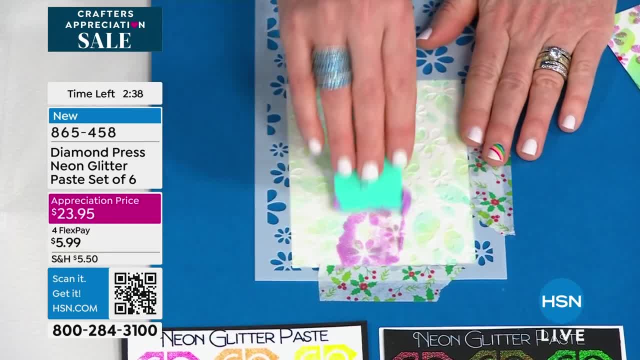 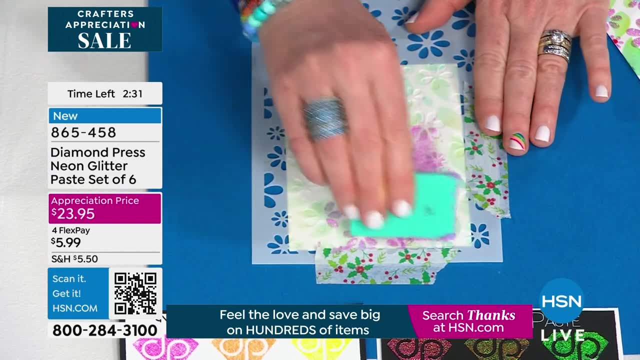 want to call it. i'm just going to take some, put it on my squeegee, slash, dauber, slash, whatever. and i'm actually going to start just smearing it. so if you're somebody that's a new crafter, this is for you, because you're just. there's no like rhyme or reason. there's no right or wrong. 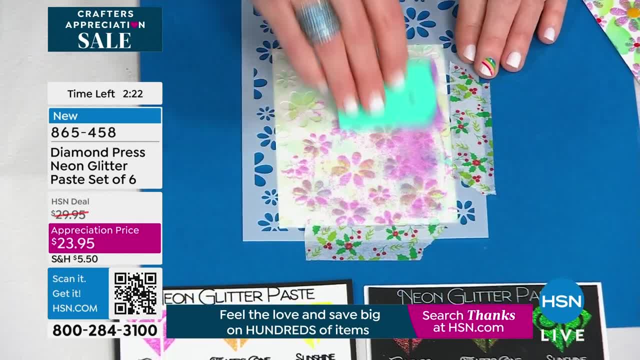 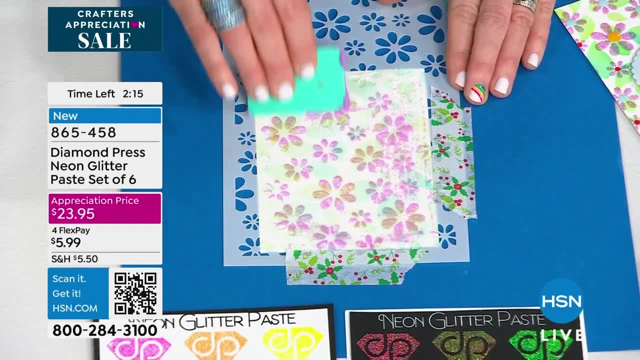 just going to add a little bit more and the great thing about someone said this to me. so i met a this weekend and some woman walked up to me and she was like i don't know, um, how involved you are in the diamond press uh process, but i just wanted you to know your glitter paste are the best in the 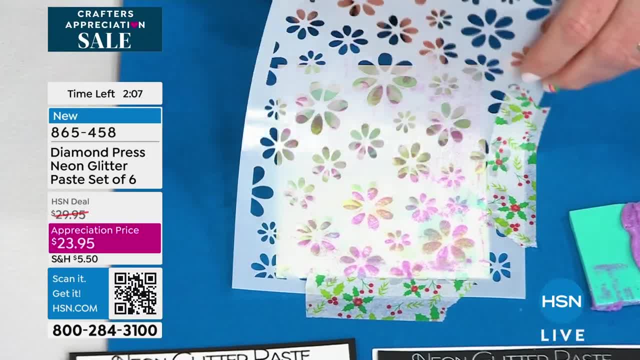 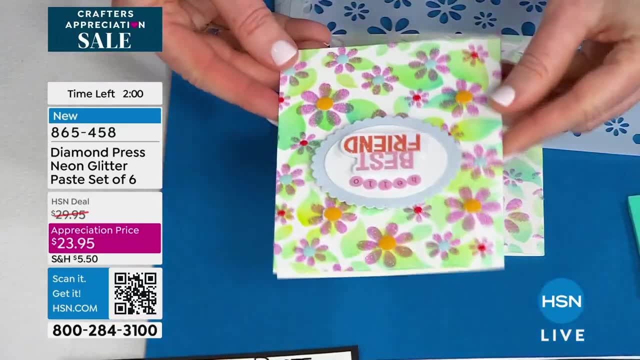 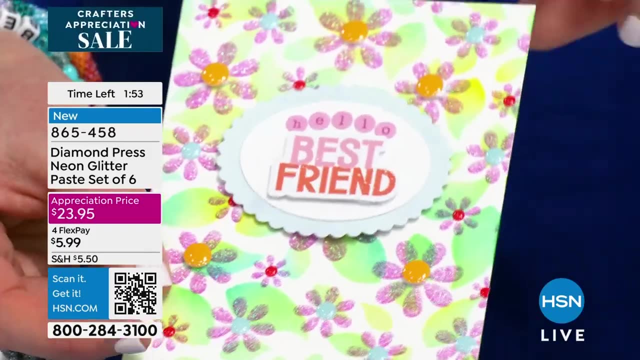 world and i was like: oh my gosh, thank you. so just a couple seconds, you lift that up, look at the pop and then, once it dries- let me lay this down here- once it dries, look, look at that shimmer. oh. look at the sparkle. oh, look at the glitter, oh yes. so here's the thing about glitter paste. i also love. 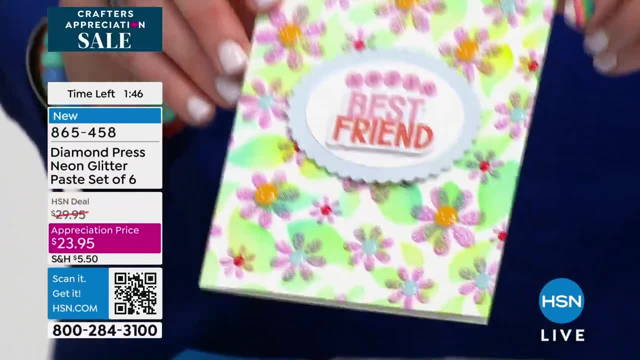 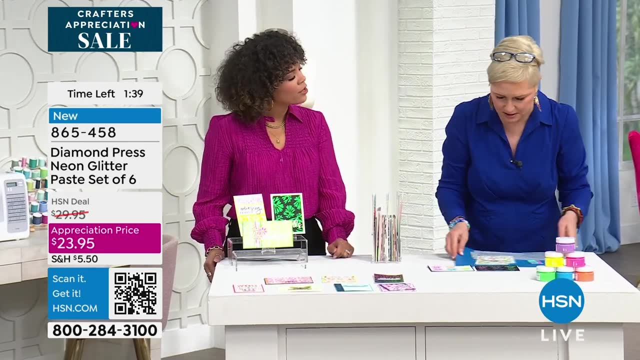 glitter all over everything that i own, including my husband and my dog. right, i don't want to put glue and then shake it all over. yes, this is the perfect way to do that. so that's the shimmer that it gives you. let me set this all right. can i use? you know the daubers that we had? could you use? 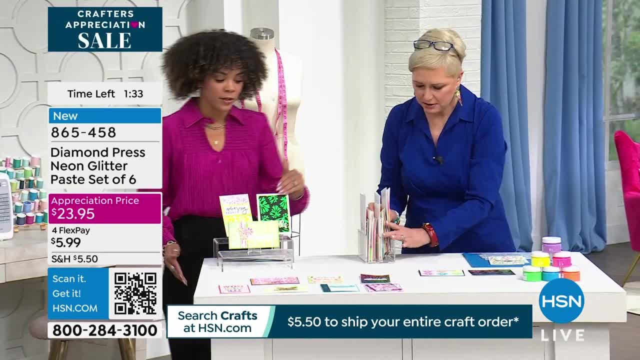 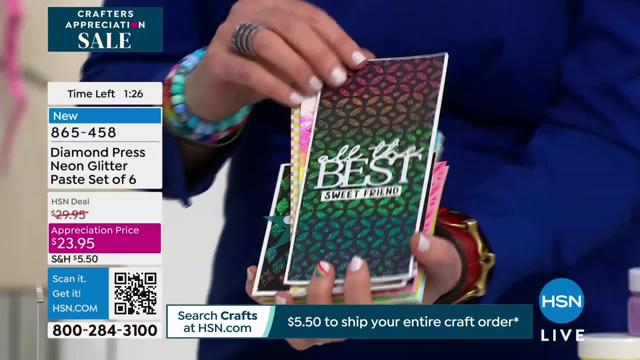 daubers with this. oh you, absolutely, oh my gosh. we have a kit of the daubers in three different sizes too, so that'd be perfect thing about. when you're getting things at this price, you can try them with different. can i use it with this tool? can i do with this? but look, look at this. this is. 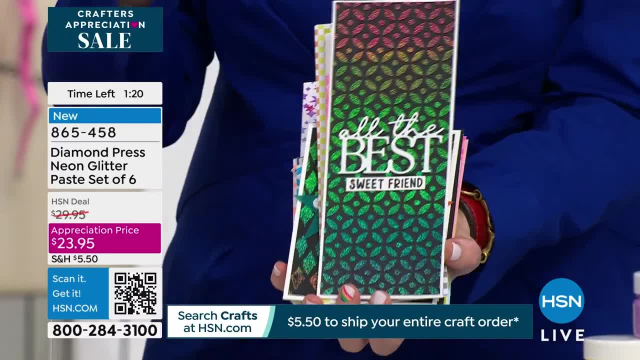 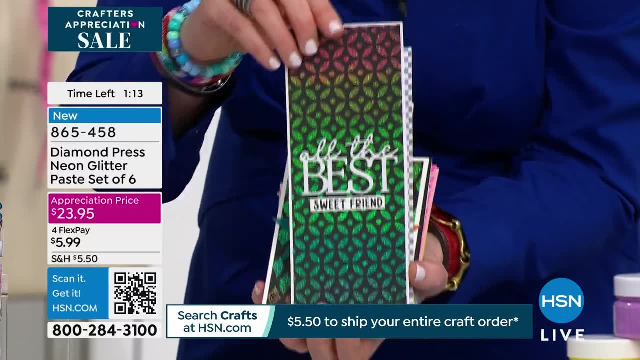 just plain black cardstock. you are going to take your project other level and here's the thing you can buy: cardstock that has glitter on it. it's two and three and four dollars a sheet. you're making your own custom cardstock with what you've already got. 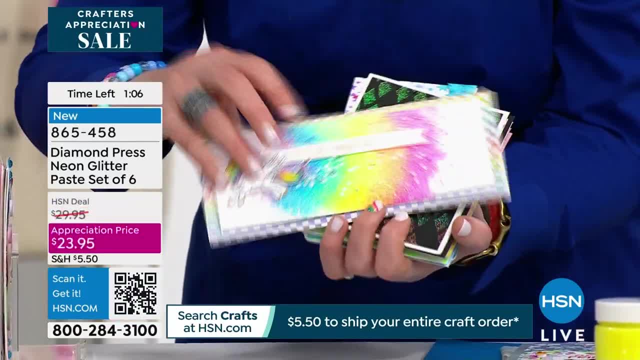 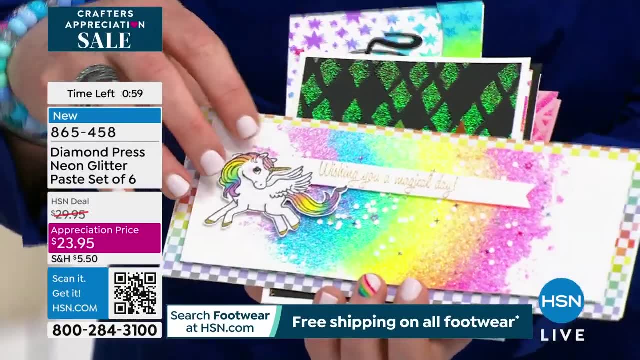 at home. um, look at this stinking- oh my goodness, precious card right here. that is what the color, the glitter colors, look like on your white cardstock. and here's the thing again. i love glitter. could you imagine like you're talking about? okay, i'm gonna put some glue here then. 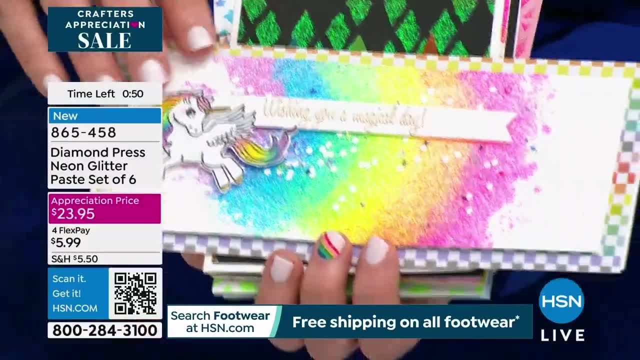 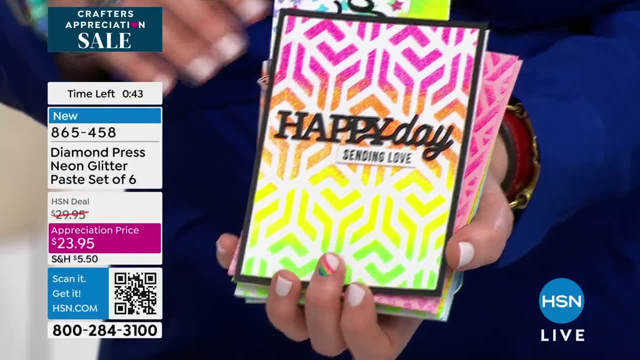 i'm gonna shake some purple glitter on, then i'm gonna put some more glue, then i'm gonna shake some more cooking oil and i'm gonna put some more glue on, and then i'm gonna put this little white gold thing on here. all of the colors are so beautiful and i think i'm gonna need a little. 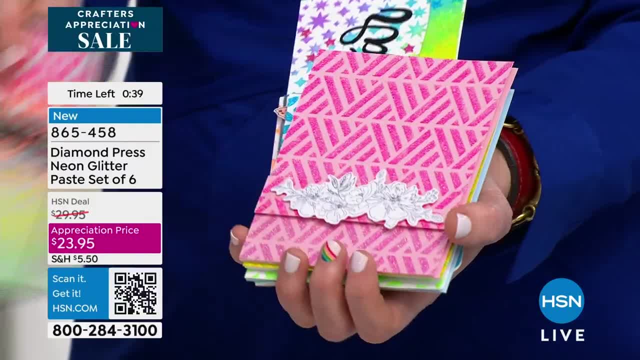 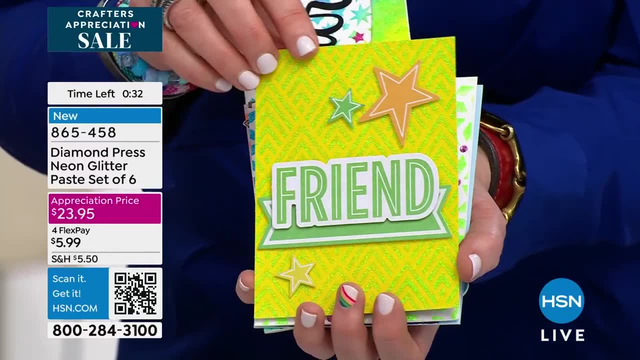 bit more of that glitter. um, it's not gonna go that well for anybody look at. but look all those stencils you've got at home that you've been like: okay, you know what, i have them, but i don't know what i'm gonna do with them. right, get this and make these gorgeous backgrounds perfect for all. 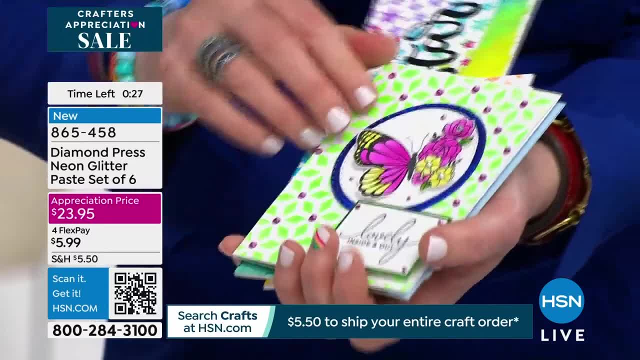 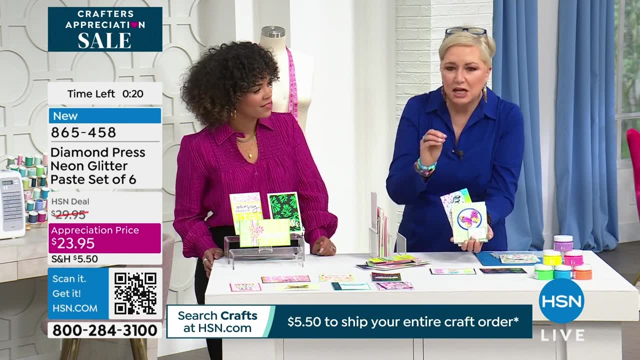 your summer cards, perfect for your scrapbook layouts, perfect for your little tag. i mean, look look at how bright and fun these are. these colors are incredible. and the quality of diamond press. if clear glue and then glitter and clear glue, Look, there is glitter as far as the eye can see, Every. 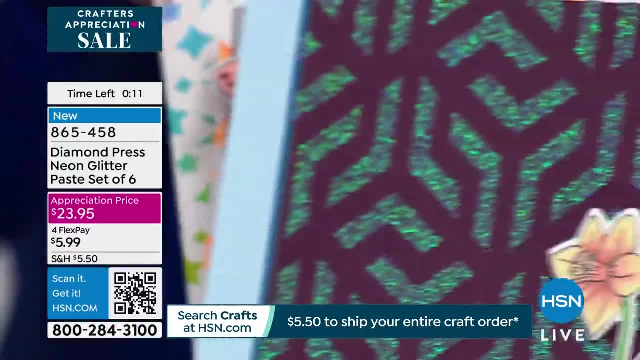 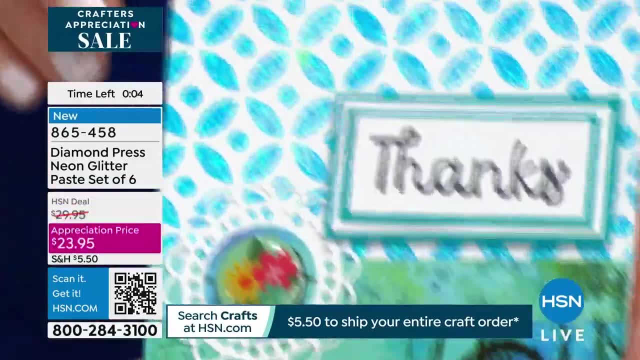 single spot where there is glitter to be had, there is glitter. That's the quality: They're beautiful. That's the quality of Dive and Press Glitter: everywhere you want it and nowhere that you don't. It's just the most. And the colors, the way they just pop off Gorgeous. The white. 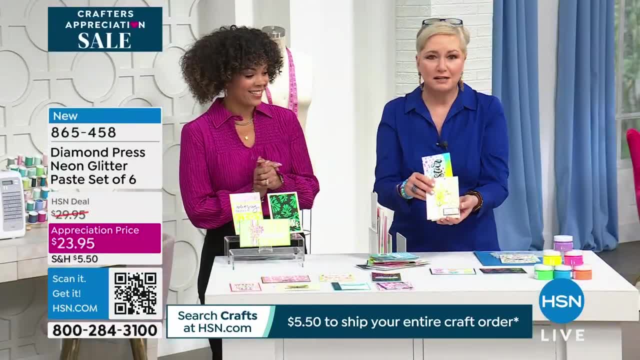 and the black. It's so good. Oh my gosh, Oh my goodness, I get too excited about it. They are so pretty. I mean, who doesn't get excited about glitter? And you don't have to like glue pour. 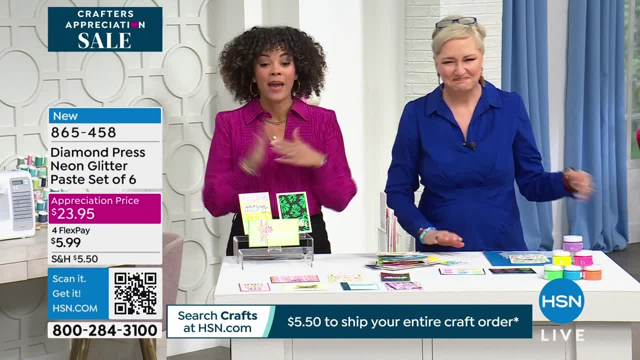 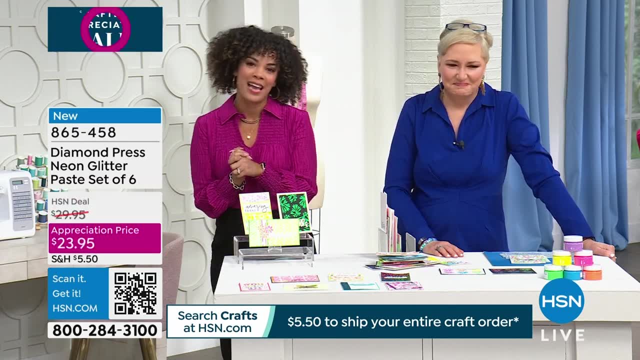 glue pour. It's like: yes, all done for you. Yes, I love that. Okay, If you want to go ahead and grab it brand new, just for you and at that customer appreciation price of $23 and some change. 865-458 is the item number. All right, You may be spotting some of the beautiful plants. 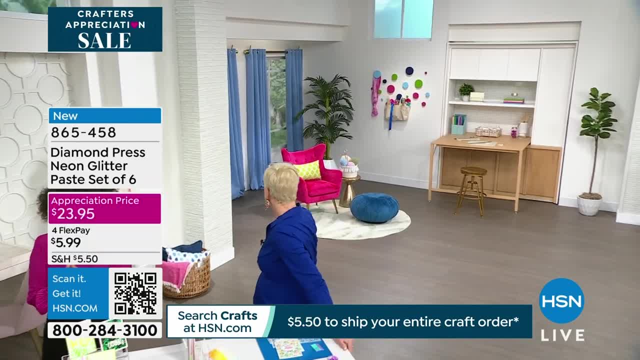 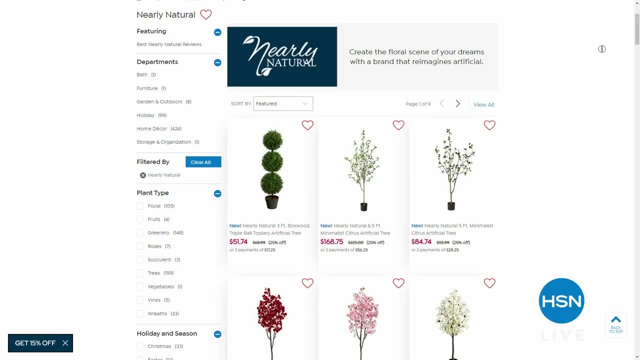 that we have here on set And if you're like, wow, do they remember to water that? No, it is not real. You don't have to. It is a faux plant from Nearly Natural And it's just that it looks almost real. 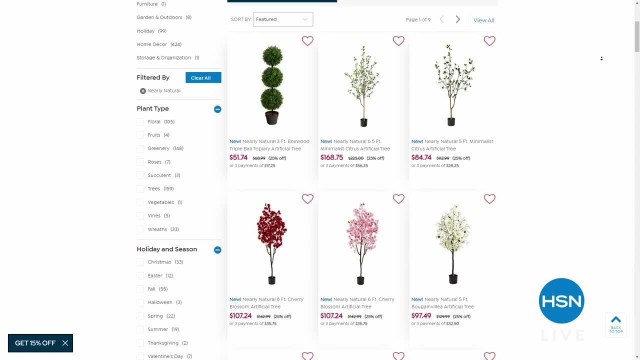 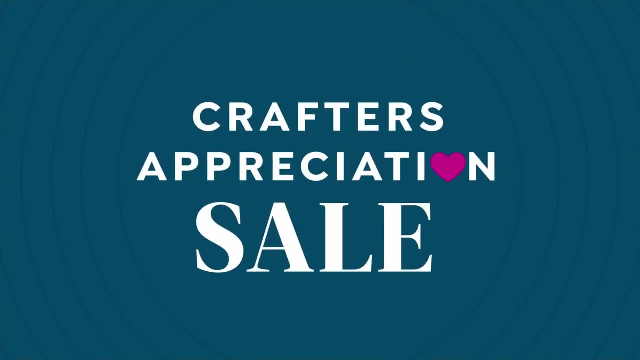 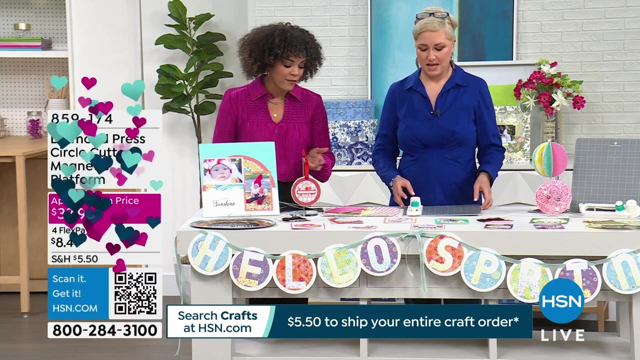 You can search Nearly Natural on hsncom. We have incredible sell prices available, even up to 25% off on some of them. So just search Nearly Natural on hsncom. Okay, This is super cool. It is super cool Because you get all these, you know, you have your card stock and maybe you even 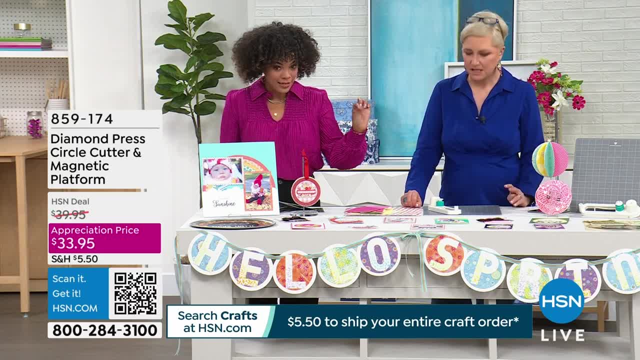 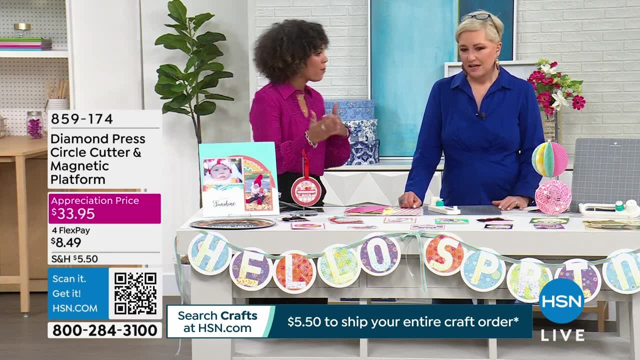 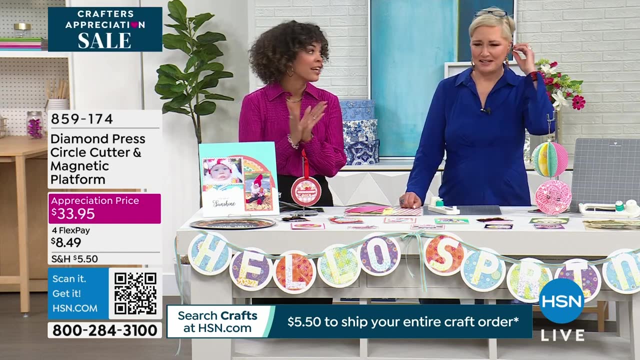 have a little bit of. you know your acetate. You need to cut it. This from Diamond Press is your circle cutter and magnetic platform. So really great for you know. small projects, large projects, whichever one, Look at the price: $33.95.. So customer appreciation month, right And all. 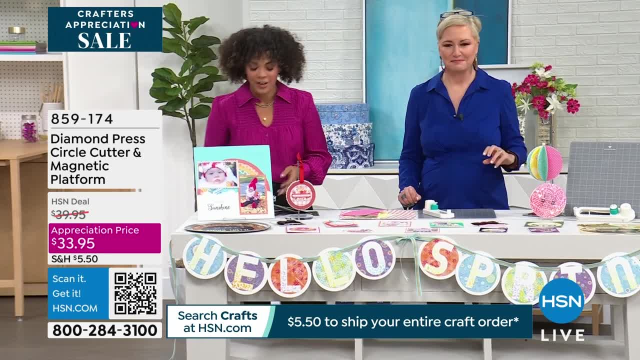 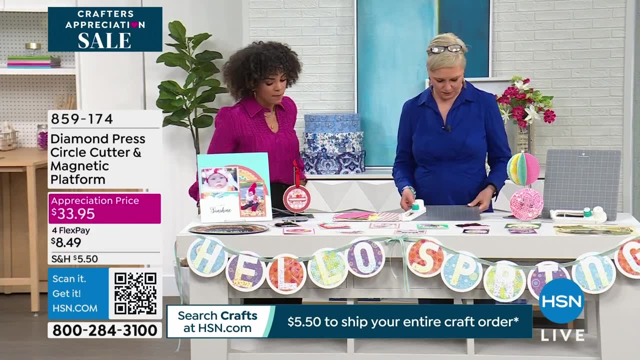 today is crafty. I feel appreciated. You should be very appreciated. I know We love our crafters here. that come here, Okay. So you'll get the circle cutter, the ruler and the cutting mat- all that you see right in front of Beth. So here's what's so amazing about this. is I so? if you've? 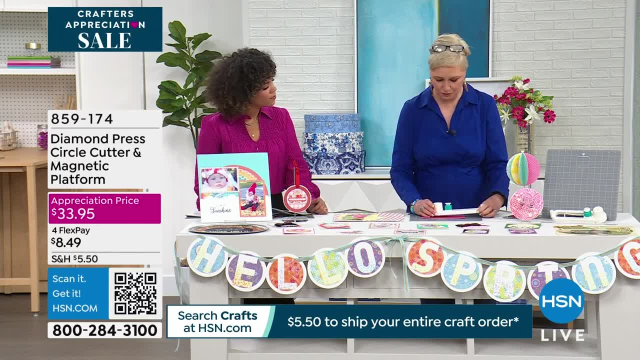 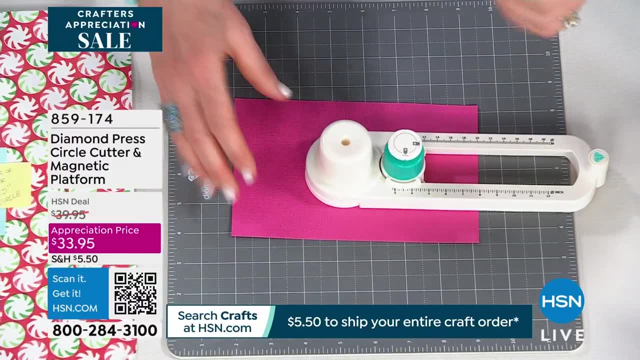 been an old school crafter for a while. you know circles are sort of like the bane of our existence, because you either use punches which are large and take a lot of room right, Or you had to get out your digital die cutting machine, which I love my digital die cutting machine, but sometimes I 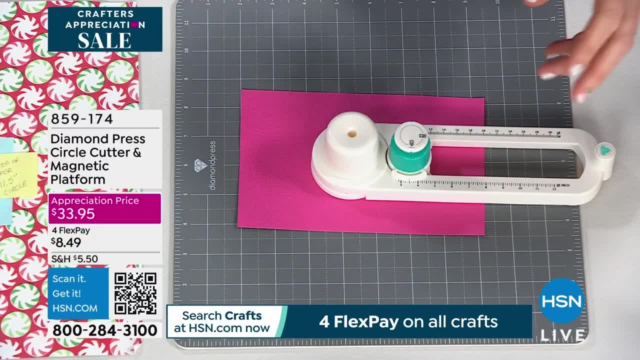 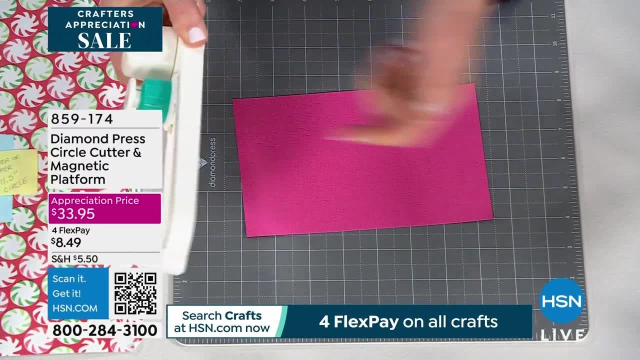 just want to cut a circle. So Diamond Press has created this tool. I'm going to show you how it works really quickly, And then I'm going to blow your minds with some finished projects. So this is all magnetic. This is magnetic. There's a magnet in here, There's a blade in here, Nothing. 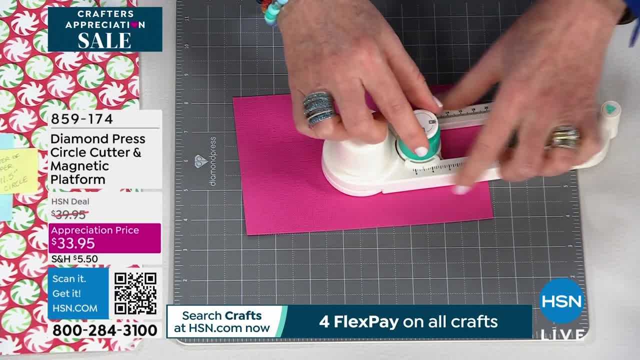 moves, Nothing moves. I'm going to set this down. my paper I'm going to this is set at three and a half inches. I'm going to lock my blade into place and we'll talk about adjusting the time I'm going. 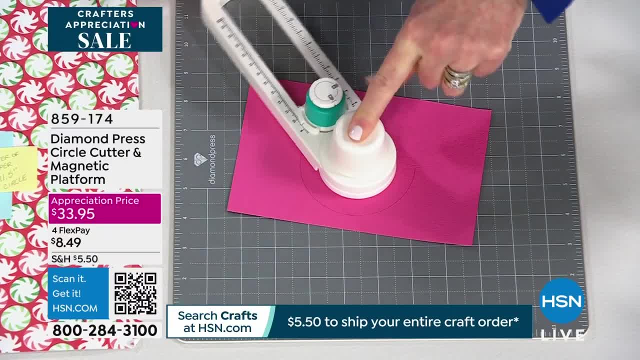 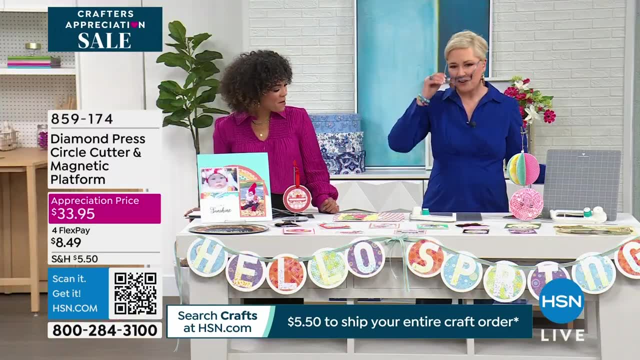 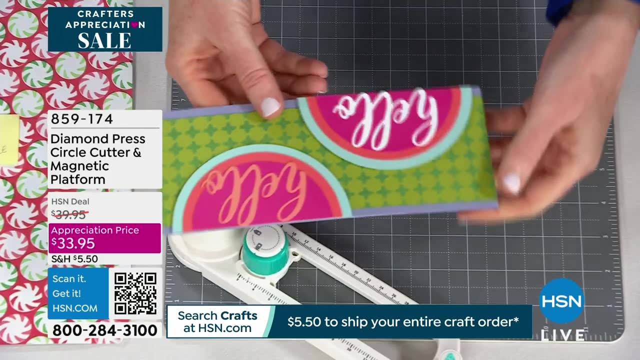 to hold onto it here. It's like a protractor that cuts. It's the most fun. This is the most fun ever. Wait until you see the finished project. So here's why this is so important again, because you don't have to get the punches out. You don't. 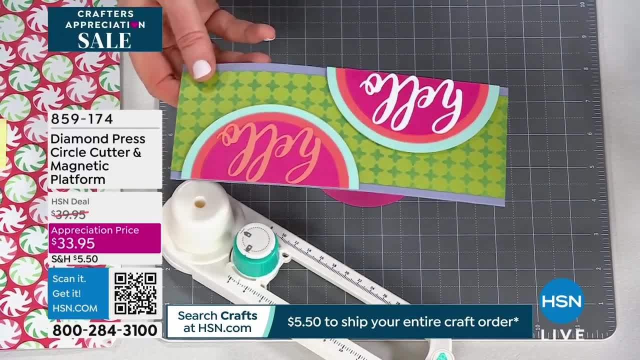 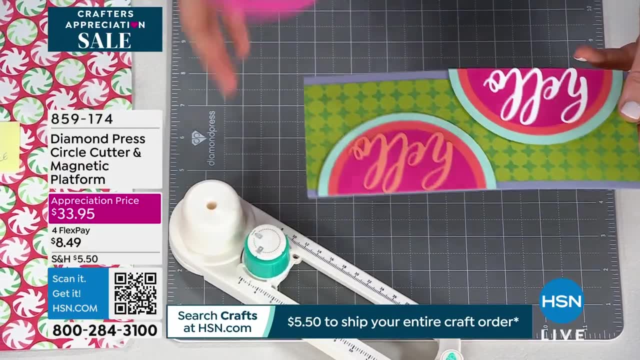 have to get you know. okay, well, I want to do this size circle, So I need to get out this size punch, I need to plug in my die cutting machine, all that stuff. You're creating these beautiful circles. So, yes, I this one you could cut in half to make this beautiful card. but Oh, by the 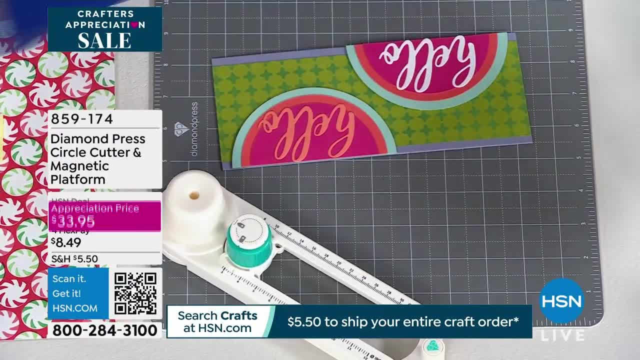 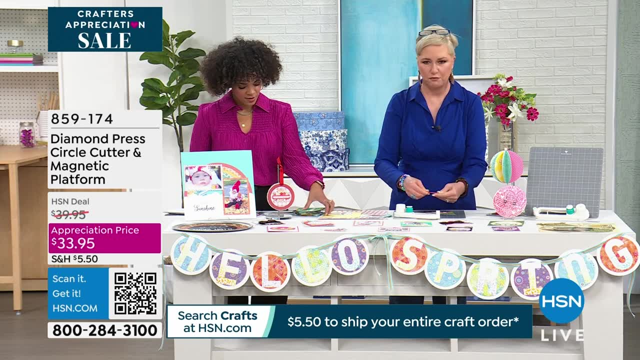 way we have some rocking. Where's my rocking card? I have it sitting over here, Girl, I'm just going to make a giant mess everywhere. Yeah, there it is, If you want to make rocking cards. rocking cards are put together by folding a circle in half. 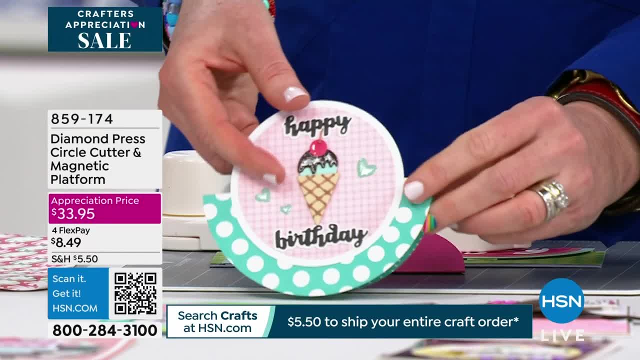 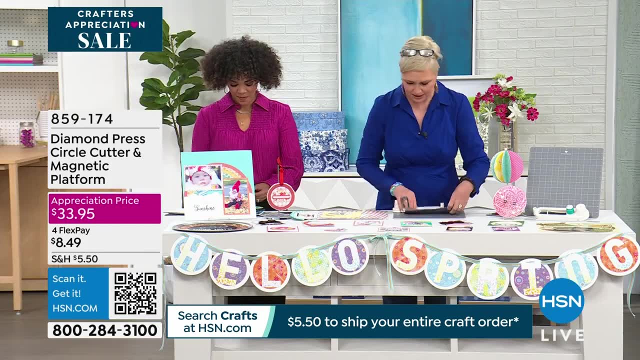 and then you set it down: Um, look at how precious this is right here. That's what the circles that you're creating with this. So that's how you're creating beautiful projects like that. Let's talk about some of the finished projects, And then I'm going to show you some more really cool techniques. 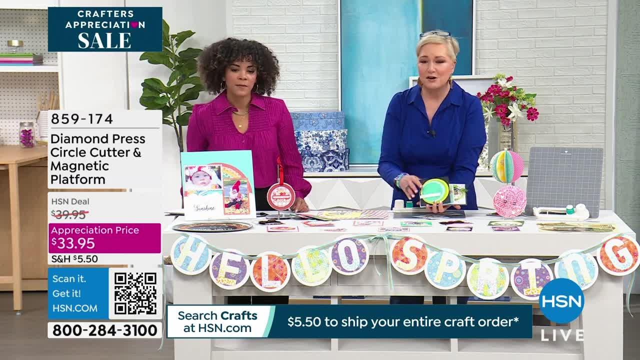 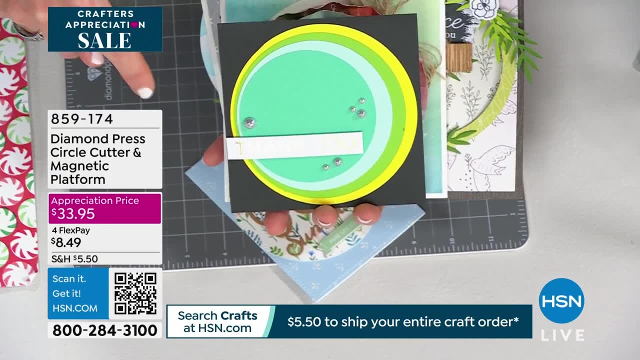 So all of these again, if you wanted to make this card. I know I keep talking about beginning crafters, but I feel you deep in my soul because if you were a beginning crafter you'd think, okay, well, I have to have four different size punches to do this circle or I have to get out my die. 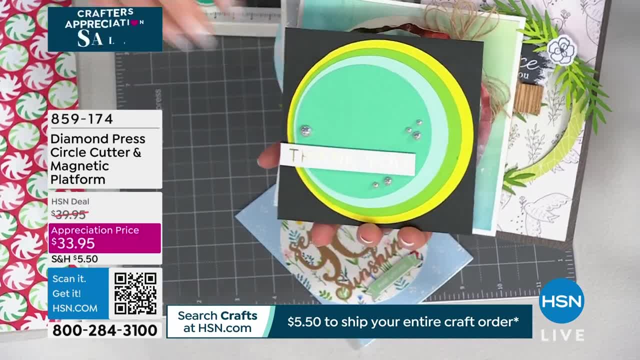 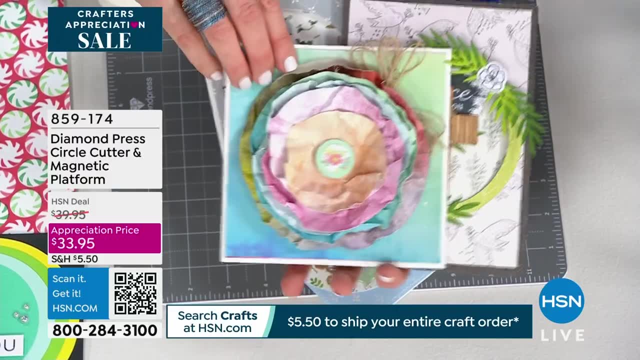 cutting machine, my electronic machine, and be like: please cut a three inch circle, please cut a four. you're doing it in just a couple swipes around the circle. look at these beautiful three-dimensional flowers that you can make with this. look at these beautiful finished cards that you can make with. 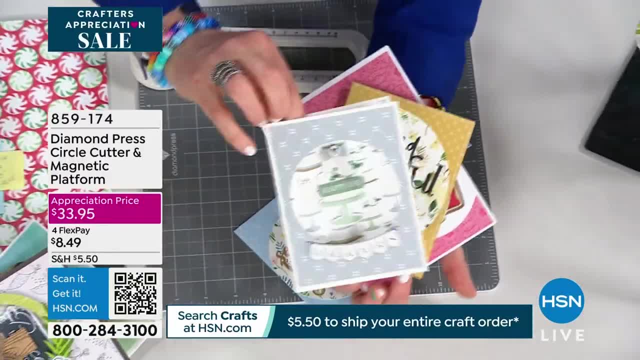 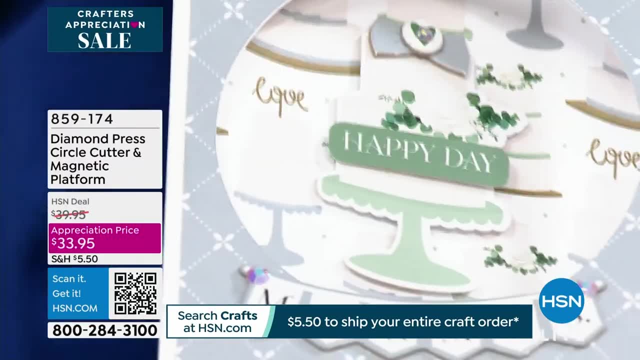 this. it's so easy to create these kind of cutout cards that you always thought you had to buy, or you had to spend five hours trying to measure and be like, okay, well, I can do a half an inch on one side and a half an inch on another and then cross my fingers and pray that it actually cuts in the. 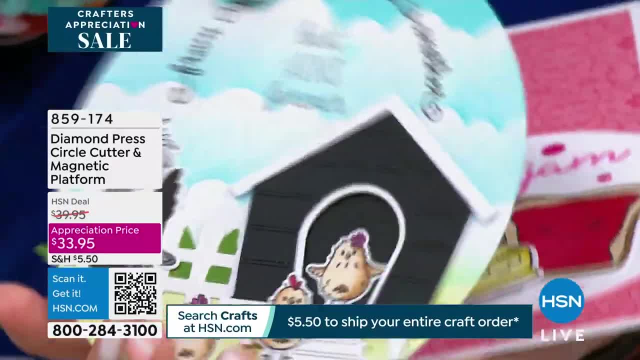 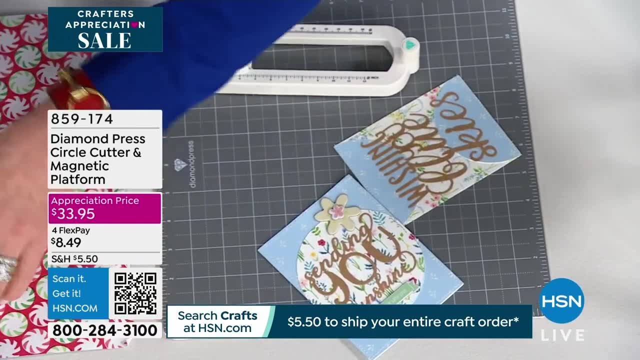 right place. all of these different projects you're going to be able to create, all these circle cards you've always wanted to create. this is so easy. let's also talk about the fact that you can cut multiples. so I've got my piece of paper and I know I'm going really quickly, but we just don't have a. 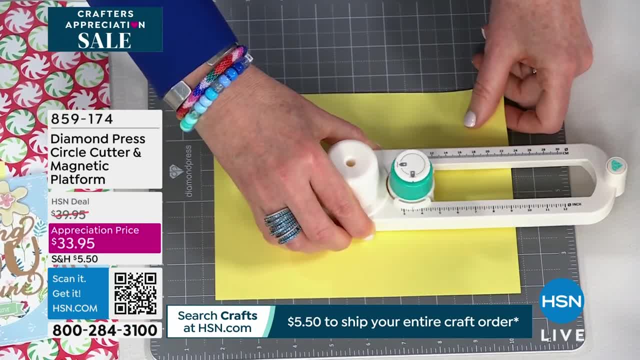 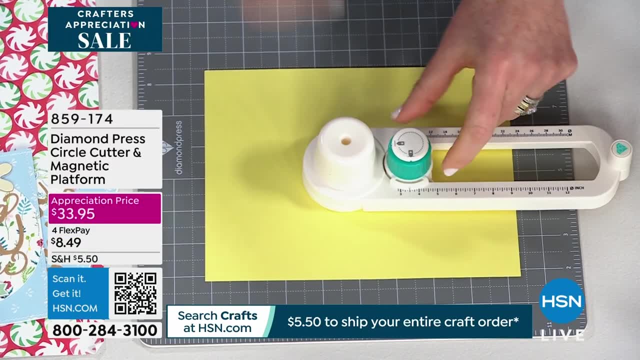 lot of time and I just want you guys to have it, because I always want you to have it, because I also want to talk about the size of things. so I turn right here: lefty, loosely, righty, tighty, whatever they said back in school. you can see there's a little ruler down here. so three and a. 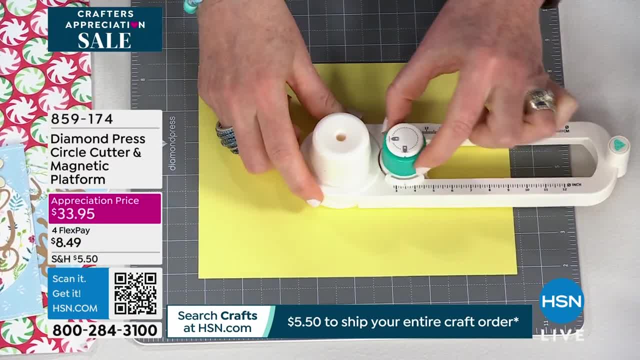 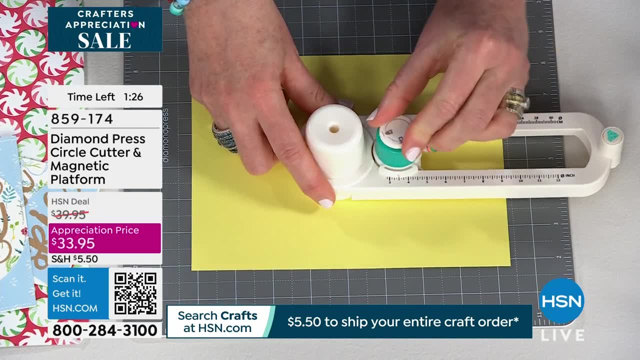 half four. this does a quarter of an inch, but here's what's important. you can see, I'm trying to move this and it's not going. it will not move if the blade is locked in place, because it wants you to be safe. so I unlock the blade, I move it down to five inches. oh yeah, because the blade 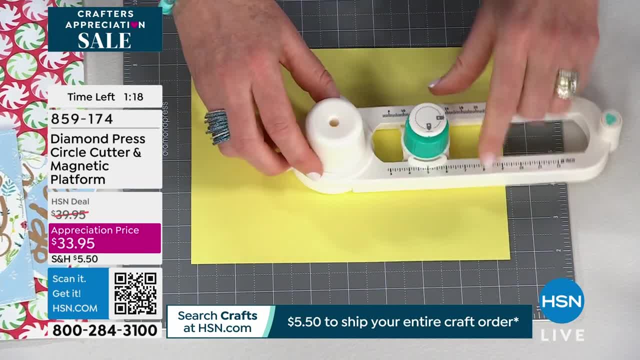 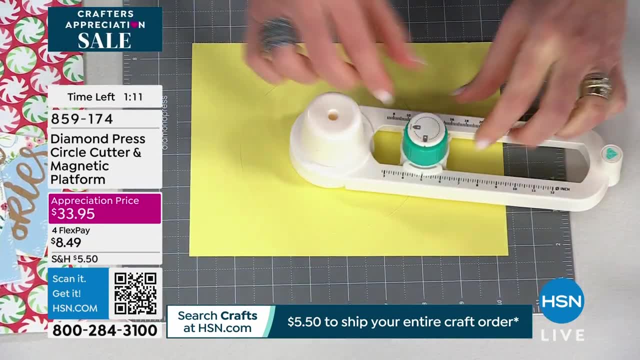 retracts, the blade retracts. yeah, because we want you to be safe. so we're going to put this down here, lock it in. I'm going to hold this, cut my circle, but now watch what happens. okay, so I want to make the shaker card. so I'm actually gonna unscrew this, move this in about three quarters. 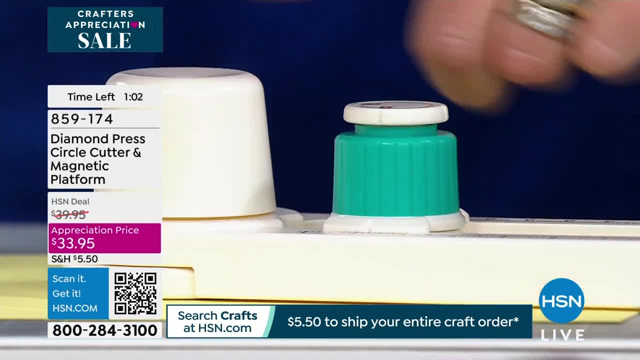 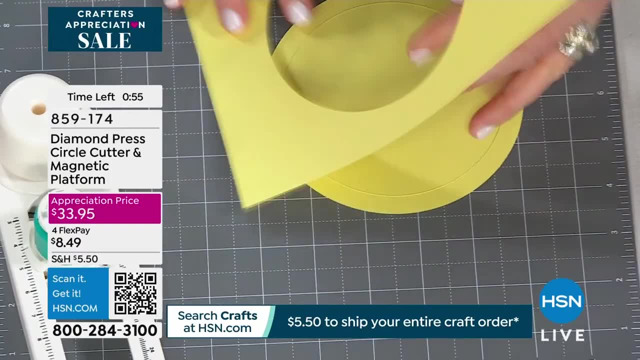 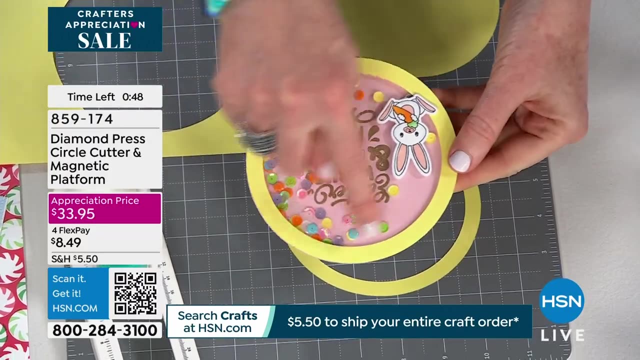 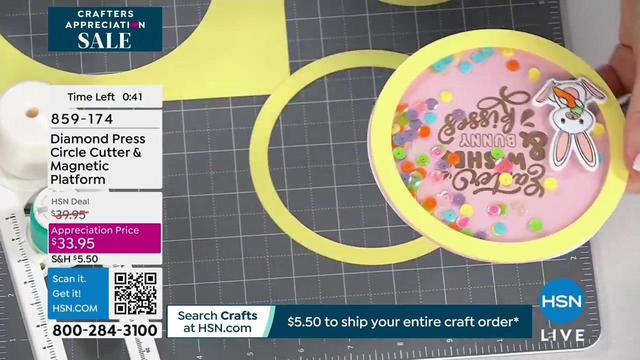 of an inch. I'm gonna screw it back down. do those in. do it again. and I have cut that is perfect, a perfect shape in about 15 seconds. and look at what I can create with this, because I can also cut the, the, the. I can also cut the pink with this, so you are creating these perfect cards in just seconds. do? 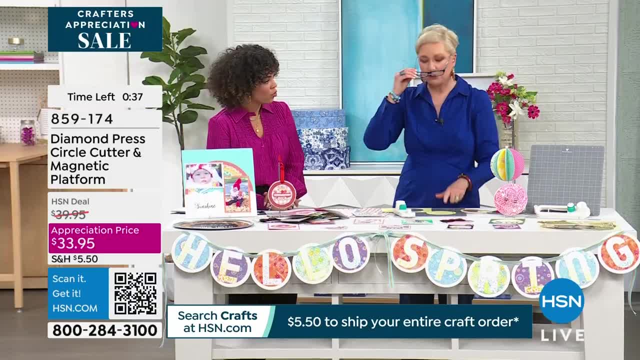 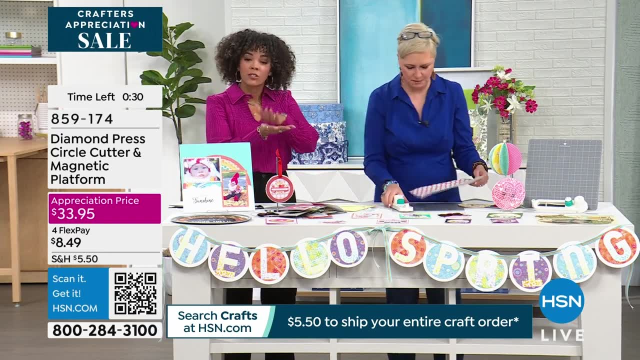 you know how long. if you are a crafter, you know how long it would have taken me to physically get out a ruler and cut these and try to figure it out, and you might shift a little bit. the fact that there's a magnet that holds it down while you're adjusting your ruler, you don't have to worry about. 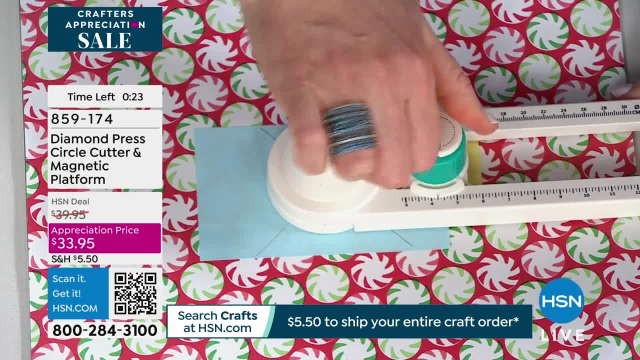 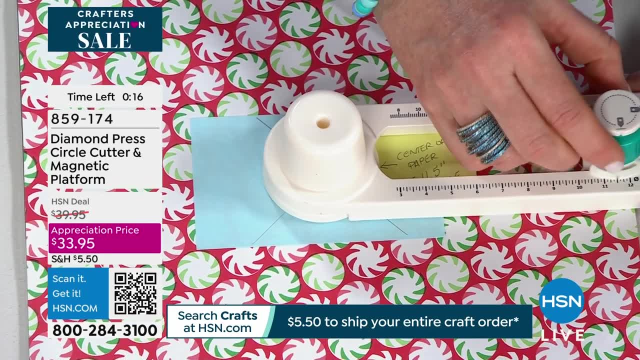 it shifting whatsoever. so here's the thing: final moments, if you want to go ahead and grab this, this is perfect for any. you know, if you're making a card for a baby shower, baby's first birthday, and just want to add that little extra detail, make that rocking car that is so cool, add this to your car item. 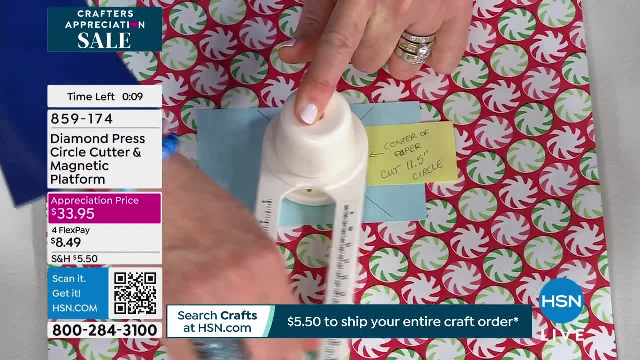 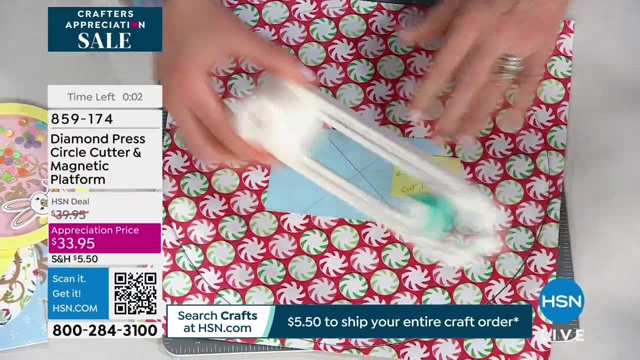 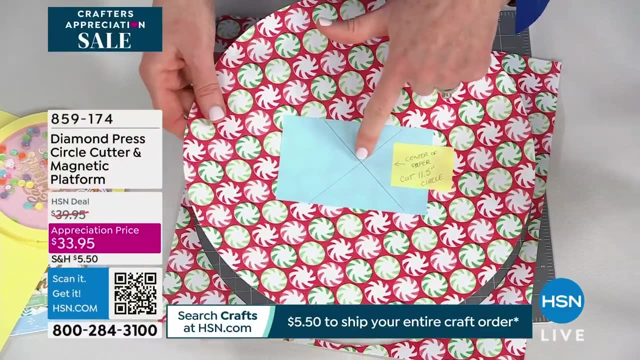 numbers: 859174. remember, load up your cart on your crafting days: 550 shipping, 550 shipping on your entire cart and then, once you check out, you still no shipping charge. 550 is all you'll pay today, which is really good. okay, here's another tip. so if you have a bigger piece and you just want to put, 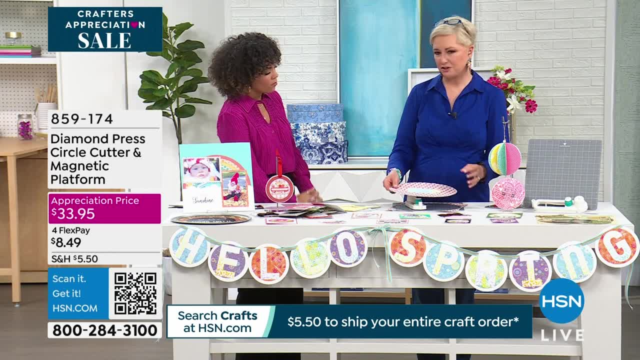 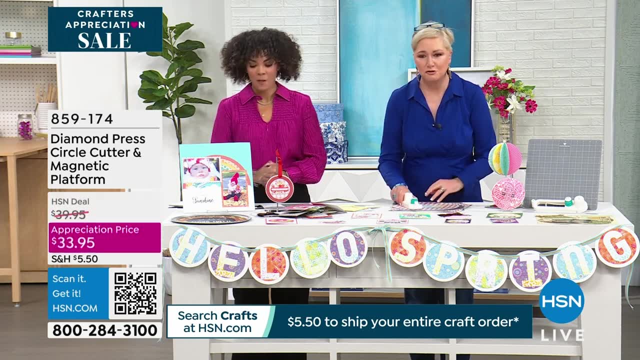 an x where it goes your die. cutting machines cannot cut full 12 inch circles. this can. so this is going to take your crafting to the next level. so if you have a bigger piece and you just want to cut it to a whole other level, it's gonna make things. so get rid of all those circle punches. get. 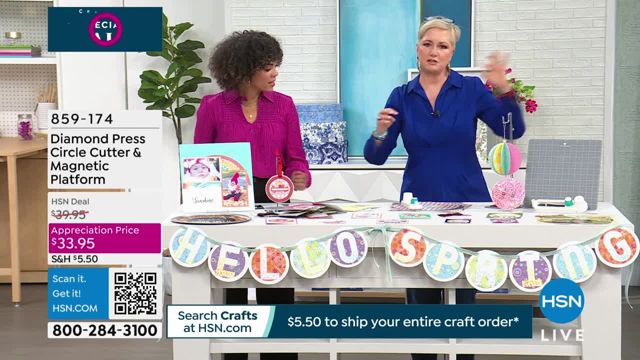 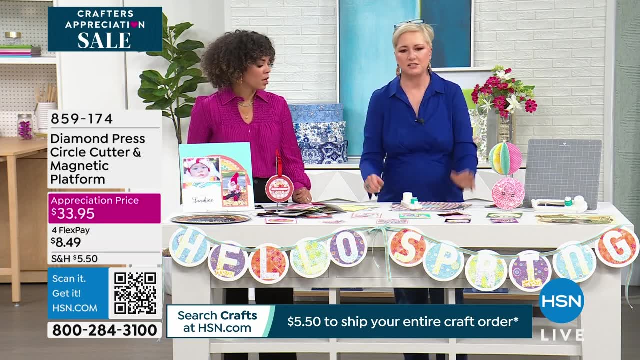 rid of all those rulers and those stencils where you're like, okay, now let me measure a half inch down this way and a quarter inch down this way so that you can get this to cut. it's such a fun and, by the way, you can use your stencils on it because it's magnetic. i mean, it's just. it's just makes life. 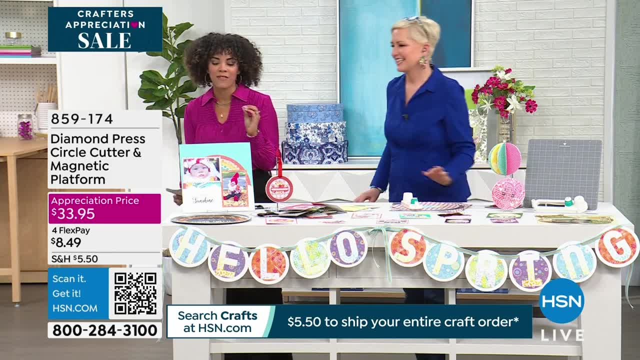 so much easier. all right, 859174. all right, come on over one more item. this was a late addition to the show, so i'm really excited that we get to share this with you. welcome in. i'm your host, nicole hickle. beth kingston is in the show today. 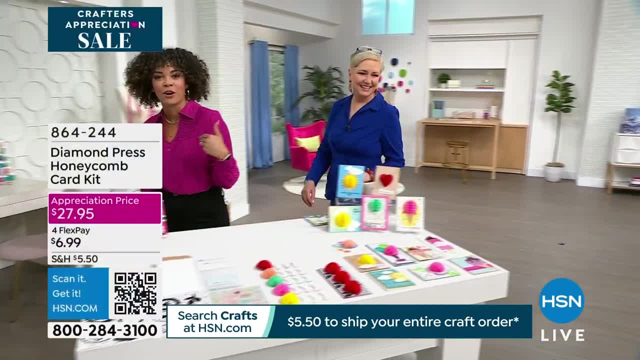 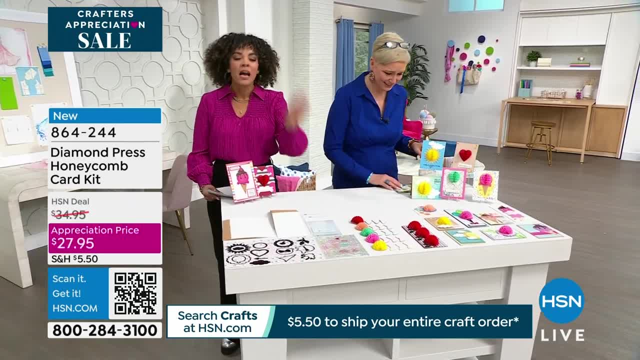 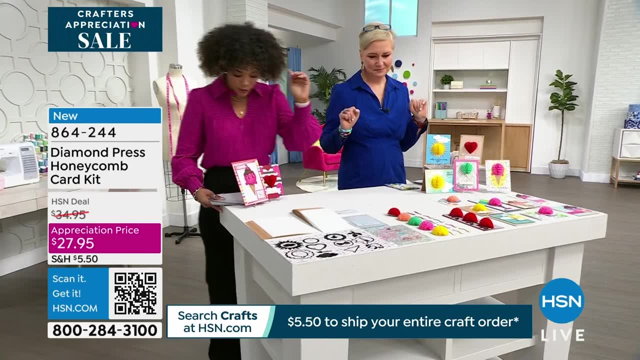 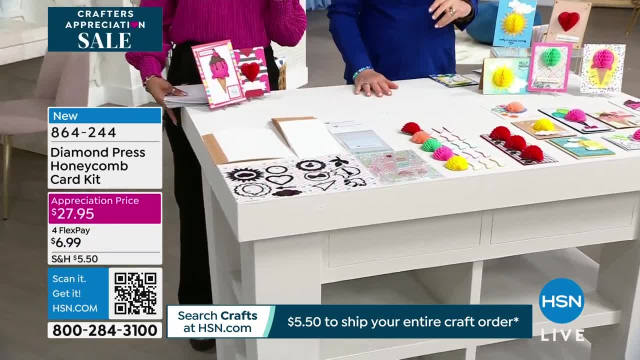 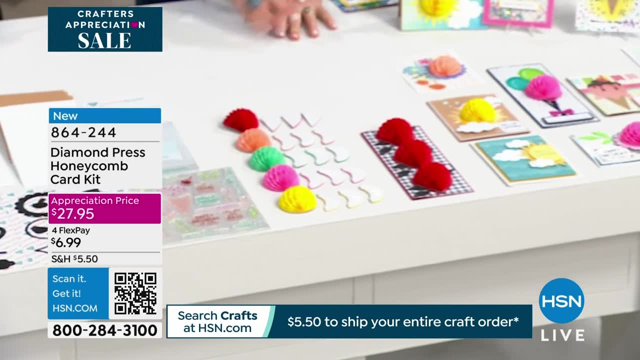 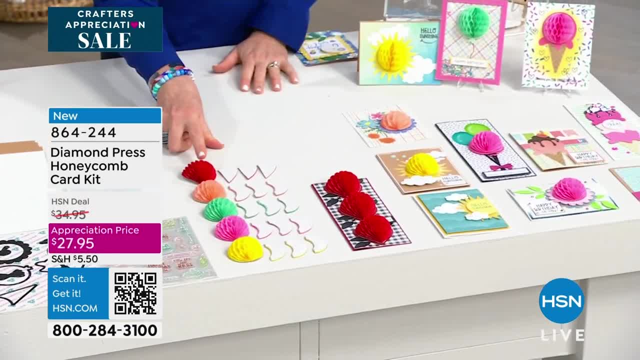 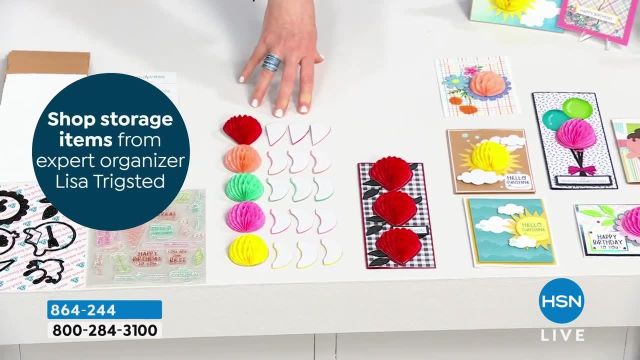 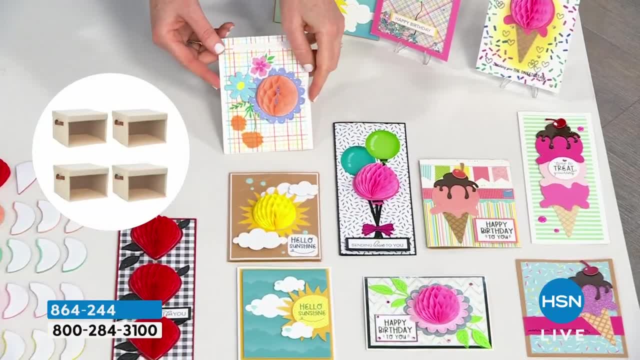 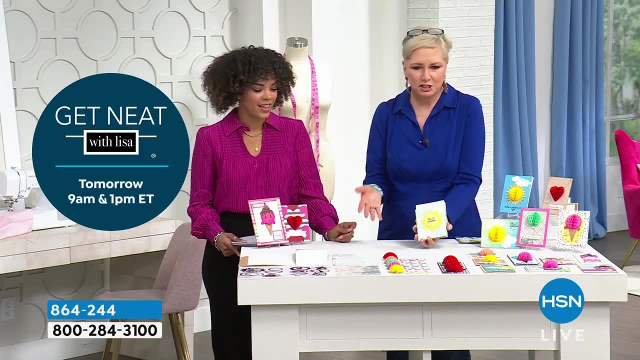 if you're giving them as gift cards, obviously you can put them on the front. i mean, it's just so fun. i'm going to show you how to use them in a second, but the real fun is putting them on the inside. so someone's going to get a card and they're going to be like, oh, this is such a cute card, thank you. 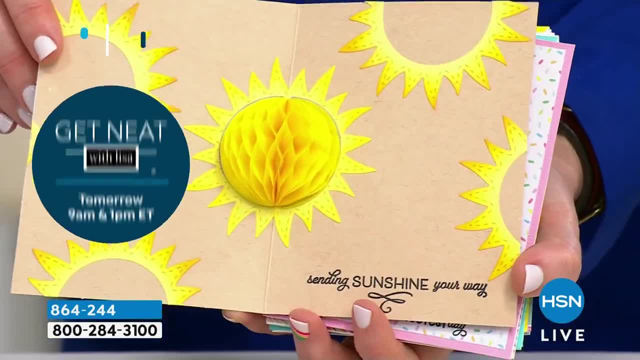 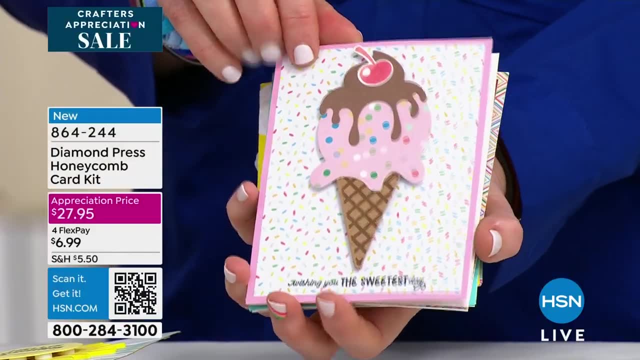 so much for thinking of me. and then you open it up. look at how cute that is. so you get the die for the sun, you get the sentiments, you get all that fun stuff, and you get the cards in the envelopes too. you get everything, yes. and then so you get the dies to make the ice cream cone. 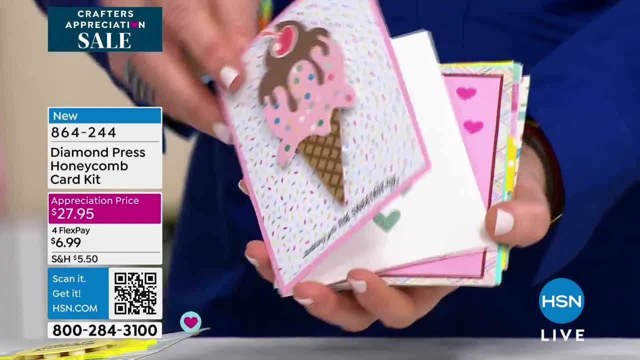 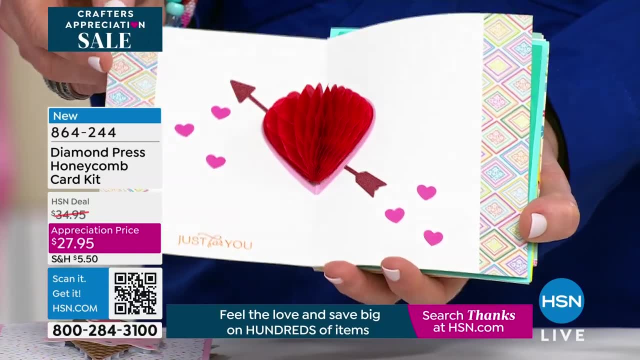 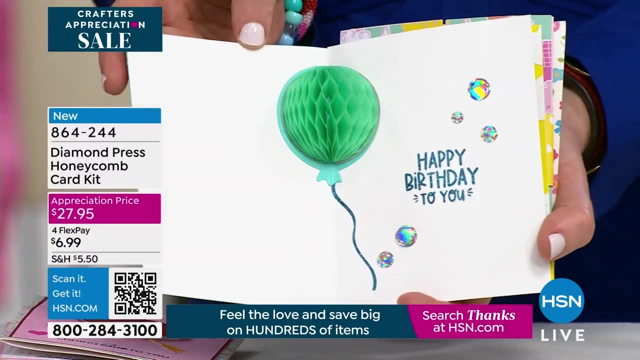 open it up, hi, it's just so fun. and here's the thing: they honeycomb paper is sold at stores. it's real confusing and hard to try to cut a shape out of it, because i have tried before. diamond press has done everything for you. i mean, it's just like if you have kids in your life, this 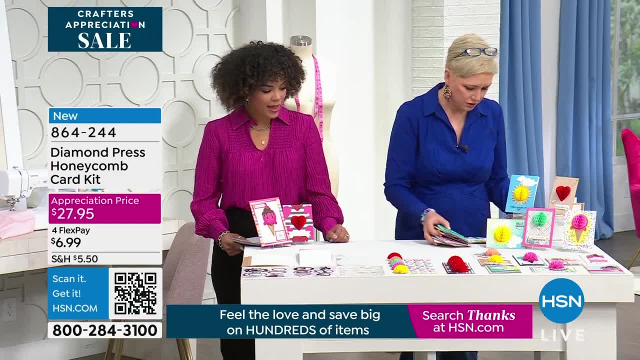 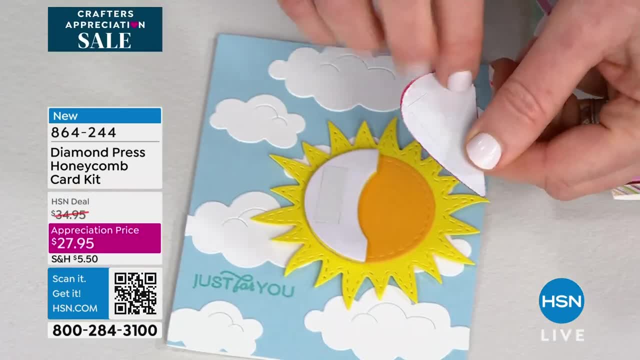 is just gonna be the most amazing thing ever. here's what makes it so cool: all you're doing, doing it's got adhesive on both sides. there's already. you're not having, you're not having to cut anything, you're not having to try to figure it out. there's adhesive on both sides. so say i, 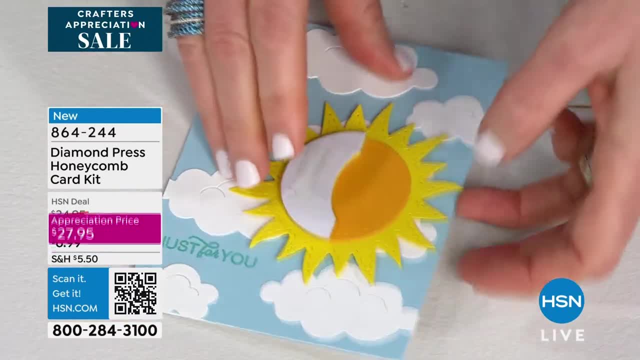 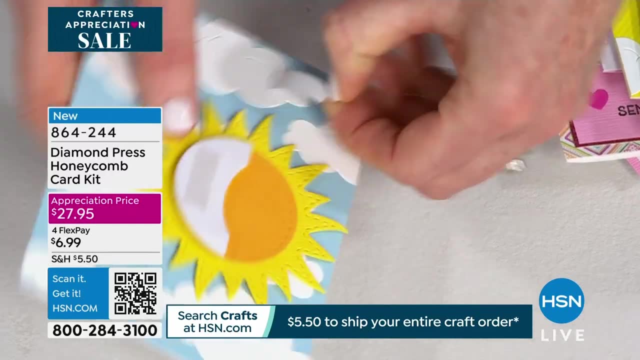 want to put this on the front. i've already added adhesive to the one side. i just peel this off and if you look closely like, there's no guessing where it goes. it goes where the circle is right. so that makes it nice and easy. i'm going to take this, peel it off. you just flip it over and press down. 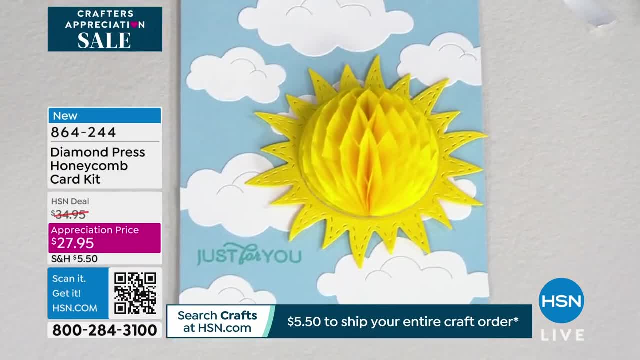 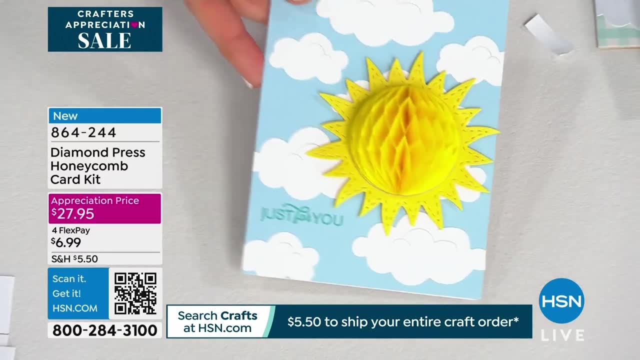 and that's it. so it fits perfectly on that, perfectly on the sun, on the ice cream cone, on the balloon. you are creating these really fun works of art. oh, this is a fun, i know, isn't it so fun? everybody's gonna love it, and so if you want to do an inside, let me show you really how quickly. 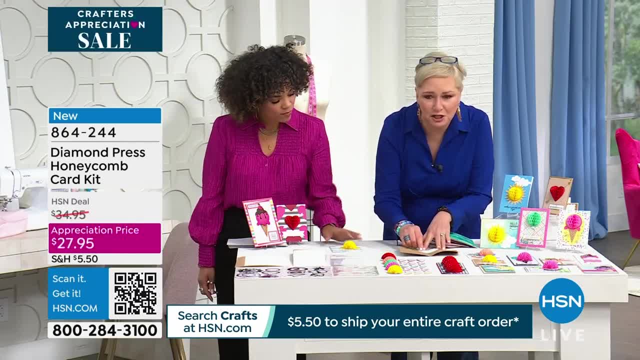 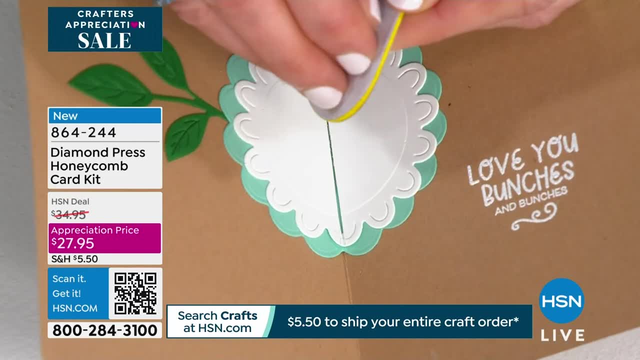 easy that is. and again, it shows you exactly where it goes. so you're not. you see this little like outlined ridge right there that comes on the dies. so you're not having to be like: well, i hope i'm getting this centered, because i don't really know what i'm doing, so you're gonna peel this. 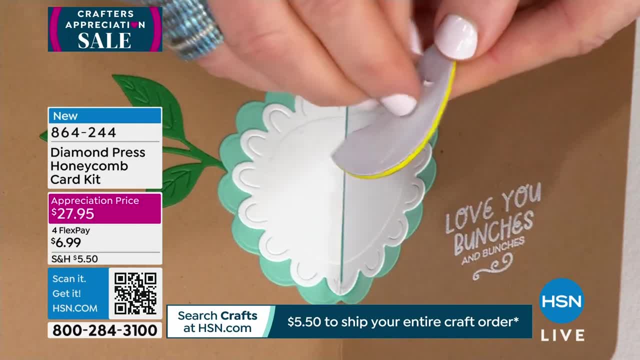 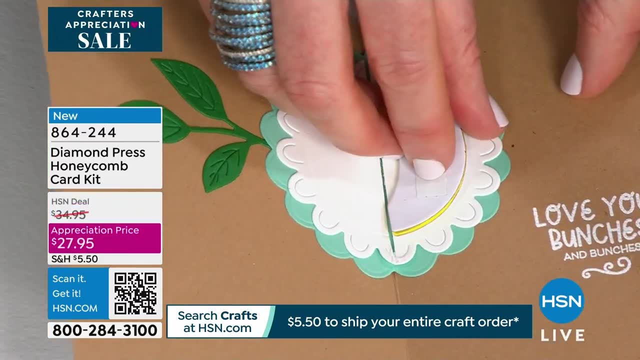 on the side, and then you're gonna peel this off, and then you're gonna peel this off, and then you're, and you're gonna come with me, i'll put my glasses back on, and there we go. okay, so it just lines up perfectly, yeah, and then you just lay it down and then you peel it off on the other side. 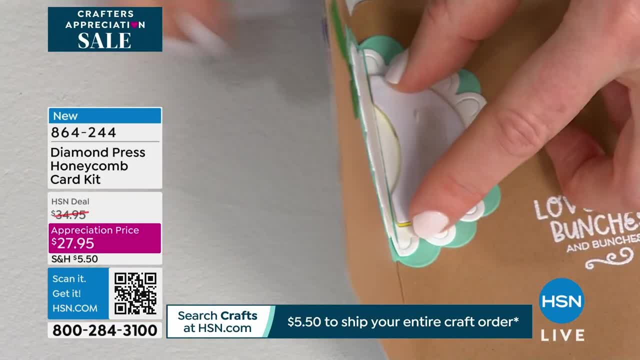 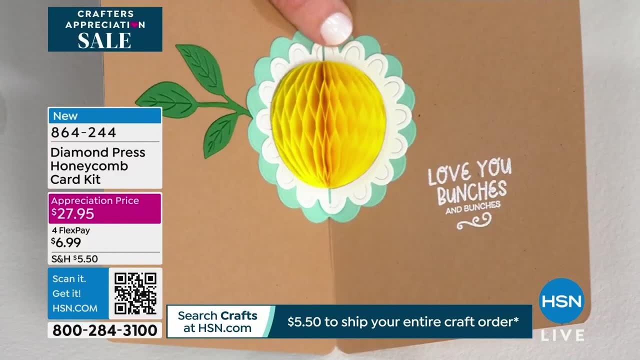 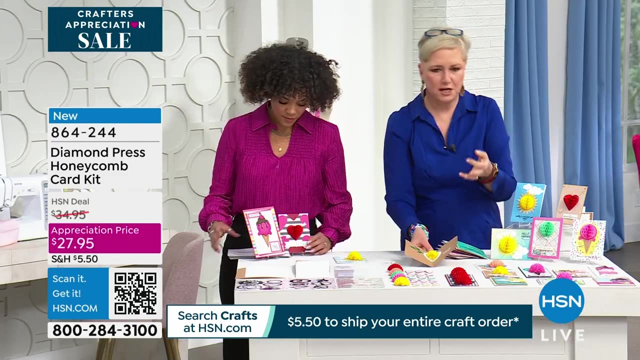 and that's the beauty of it is: you're not having to get out adhesive and you can. i'll just fold it down and then be surprised. i mean: but look at how perfectly centered everything is, perfectly sized. you're not having to guess and be like: okay, well, i need to punch a two inch circle with a two. 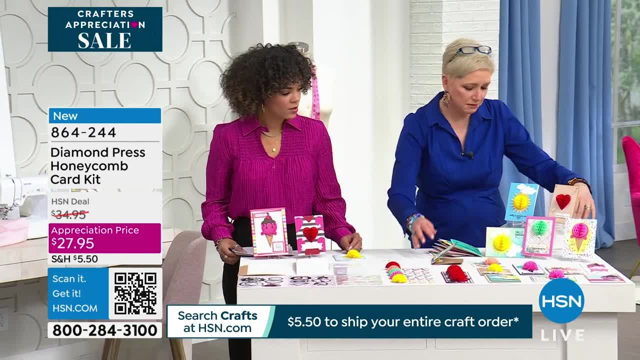 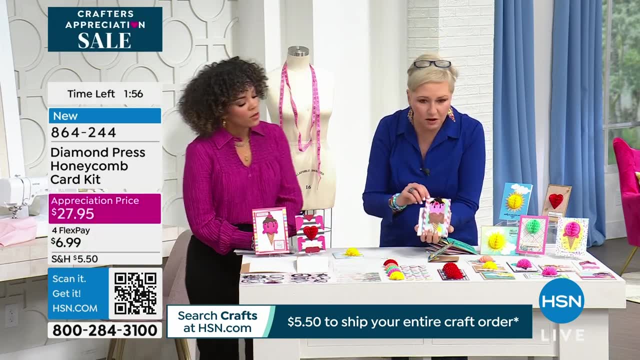 and a half inch flower. everything you're getting comes with and it just makes the most amazing cards. but the beauty of diamond press sets is you may say, okay, yeah, this honeycomb is fun, but i might not always want to make a honeycomb card. right, the cards are just as precious without. so. 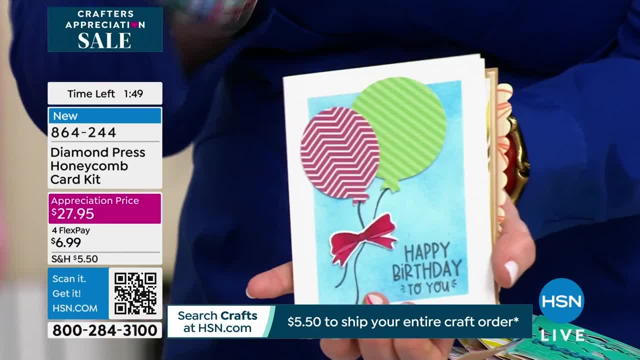 this doesn't have a honeycomb anywhere in sight, and it's just as much fun. you will use this balloon dye all day, every day. you will use the sunshine dye all day, every day. you also get the rhino card. so if you're not going to finish, you'll have to make a decision. if you don't want to. 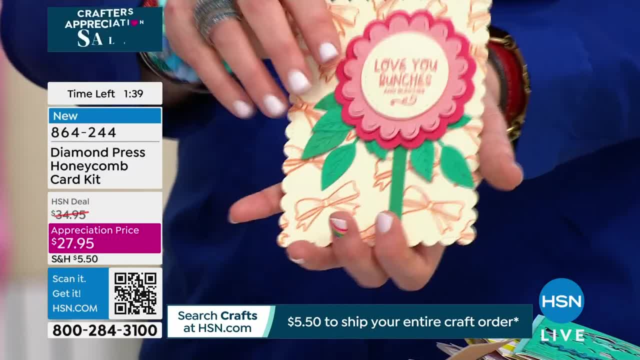 make a Jedi bench for your, it's fine. if you think you're not a Jedi bench, you're not going to make a ice cream dye, the floral dye. These are things that you will use over and over and over once you've used the honeycombs, But imagine giving this, like with a floral bouquet, and then sticking. 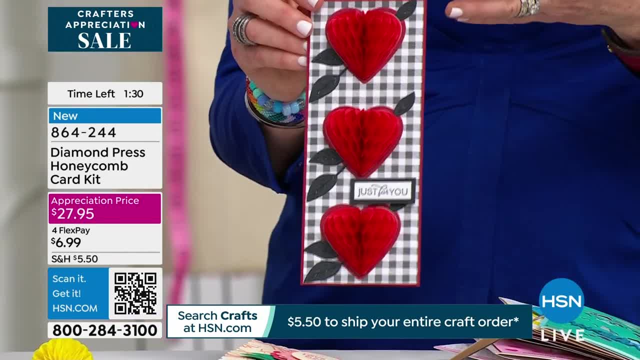 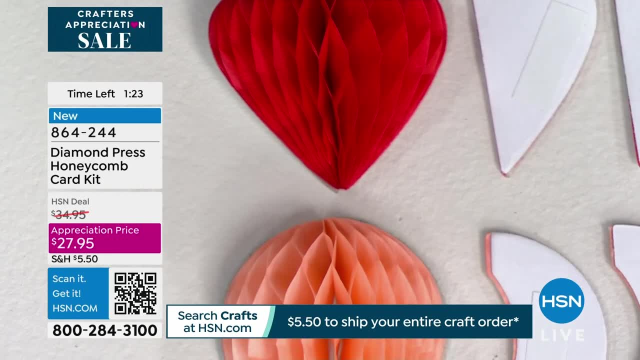 this inside? Oh, this card. We keep talking about how expensive cards are. You couldn't pay for this $12. probably you'd pay for this card because it's got the three dimensionality of it, Right, But you can, or you could use it on tags, You can use it on all those beautiful stuff, But it's just so easy. 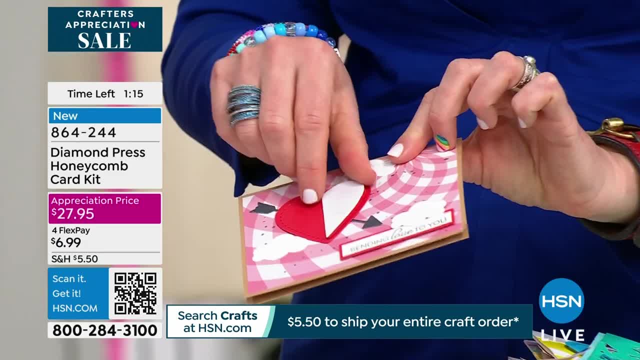 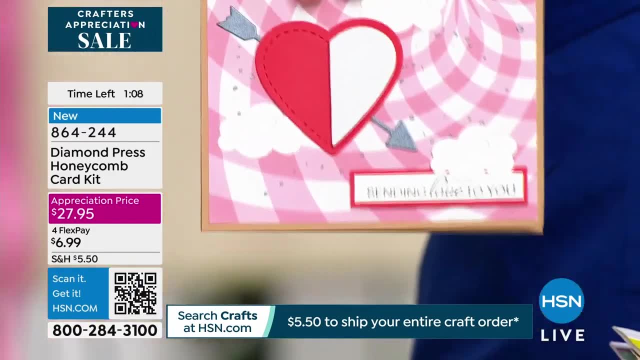 Or you could send it like this and let them do the other side sticky and fold it open. So that's another great way if you want to do it on the front. There's just so many cool. So like an interactive card for you. But you get all the cards, You get the dyes, You get the stamps with. 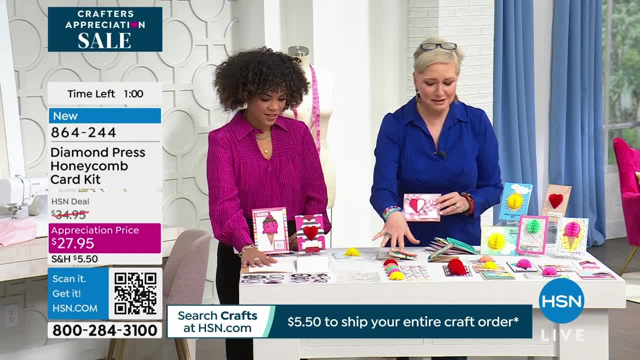 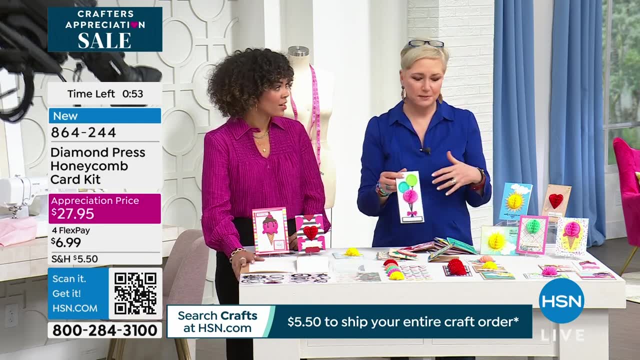 all the fun sentiments. You get the adhesive sheets, You get all the little honeycombs in the heart and the four colors of the circles. It's just such a fun. I mean, it's just so precious A throwback to our childhood, Something that kids of all ages will love, Right, Which is hard. 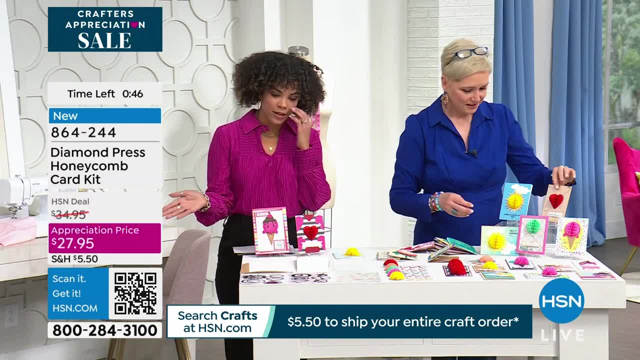 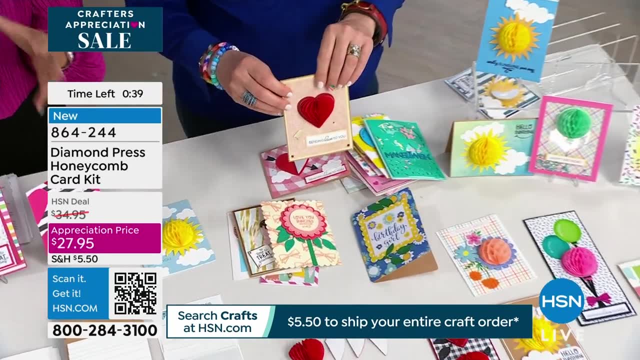 I mean you're at this, You're making 10 cards at this price of $27.99.. I mean, that's just a couple. Oh my gosh, A card. I mean that is so good, You know a little bit less than that. I mean, it is such a phenomenal. 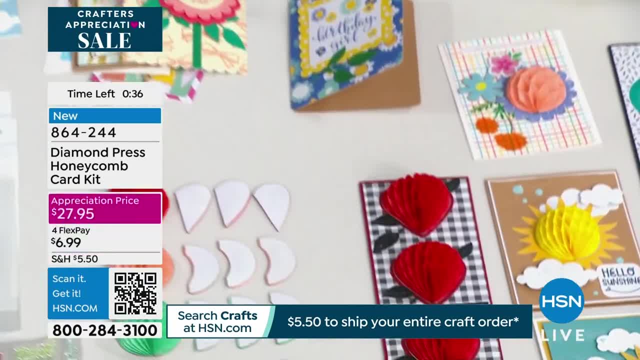 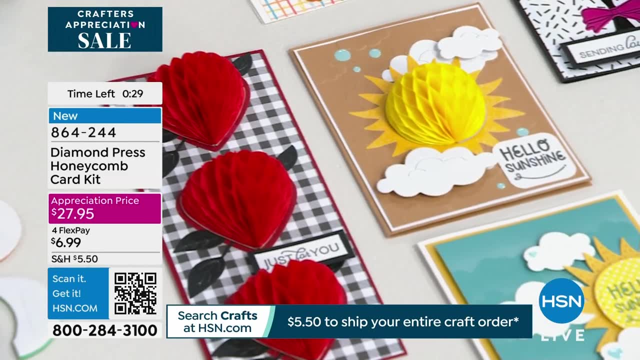 phenomenal deal. So the final moments to place your order. HSNcom, HSN app, Remember- your entire craft order ships for $5.50 today. That is your fee, only today, $5.50.. So take advantage. 864-244 is the item number. That's really. I mean, that is your card making kit. 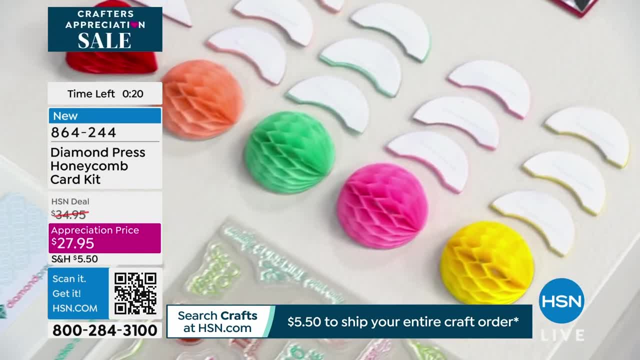 Truly. Oh, it is. It's everything you need. You don't even need adhesive, because the adhesive is on the little honeycomb. Come on, It's so good You checked every box for us, Beth. thank you so much. It was so good to see. 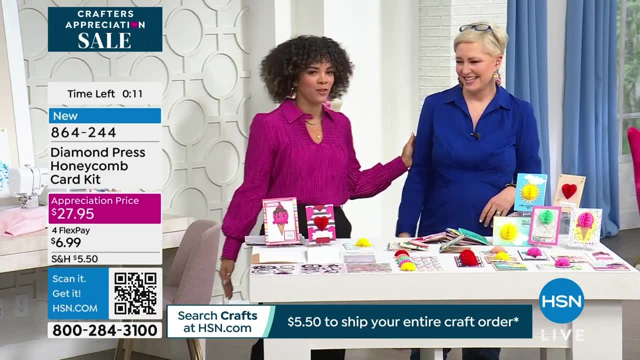 my friend, Next time I see you I'll put some shoes on. That's okay. I love you as you are. I mean, we're about the same height. I just might as well. We're good, All right, Well. 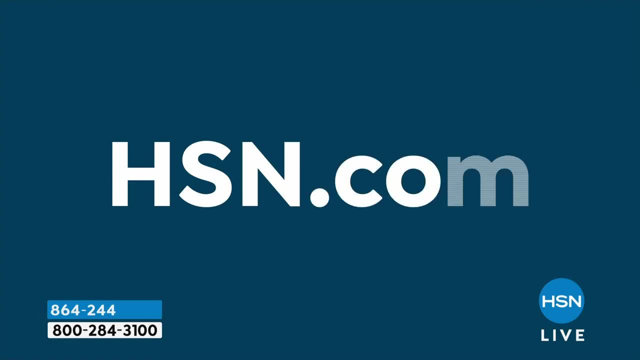 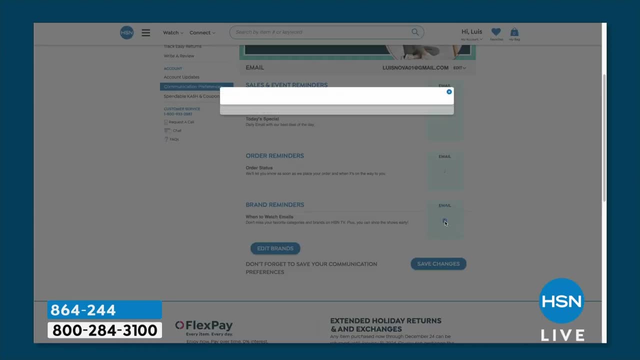 if you want to always know whenever Beth's going to be here, whether it's with Diamond Press or with her Kingston Crafts, you can sign up for our win. to watch emails, Just go to your account, your communication preferences, and then you sign up for the brands that you want to know. We break. 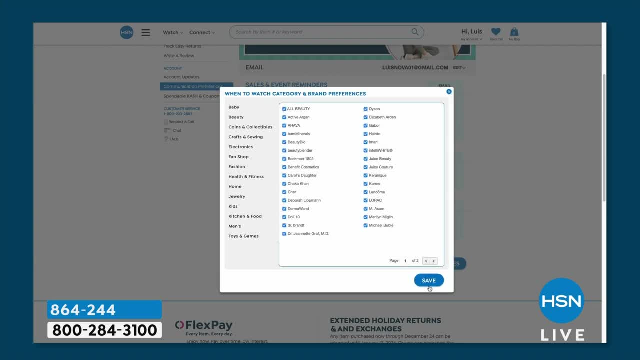 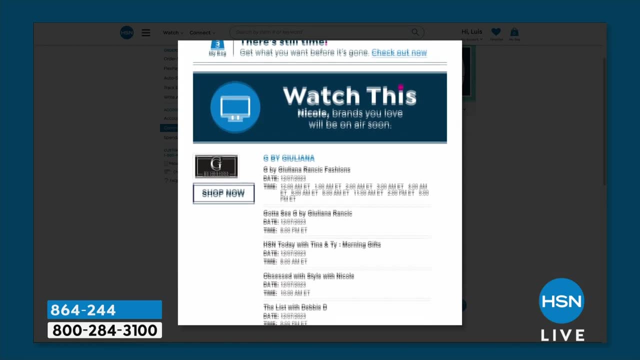 it down into categories so it's really easy to locate And we'll let you know when your favorite will be live on air. All right, We're going to take a really quick break, but come on back more after this to load up your cart for our crafters appreciation sale. 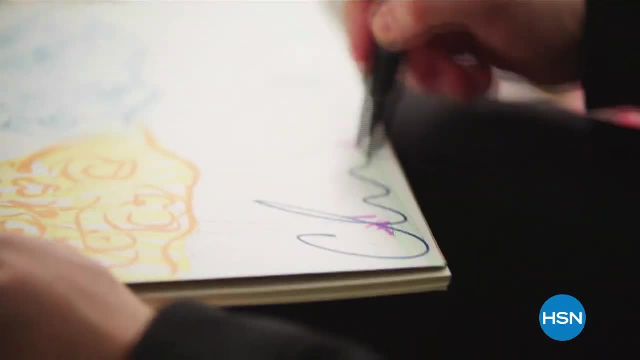 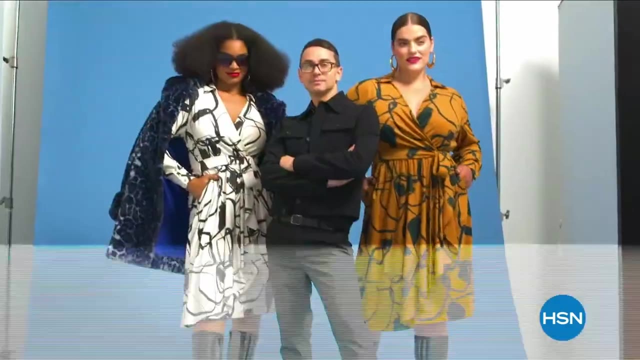 I'm Christian Siriano and I'm a fashion designer. I really wanted to bring something whimsical and a little bit of fantasy and fashion to HSN, but still something that was very wearable and beautiful. We have had so much fun the last year creating. 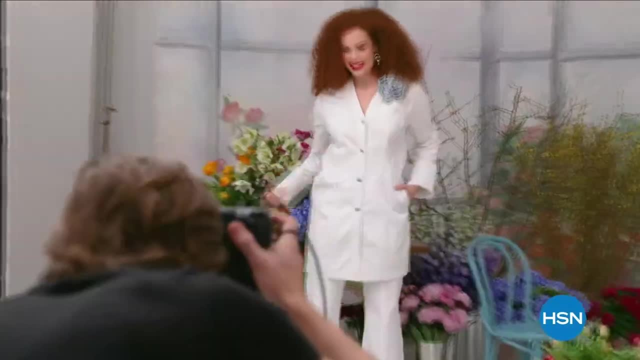 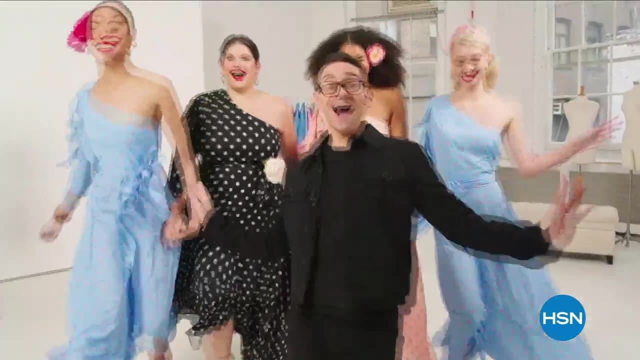 such wonderful pieces that I hope people really feel good in, and it's just been a blast. I've designed and dressed first ladies, fashion icons and movie stars, and now I get to design for you Only at HSN and hsncom. 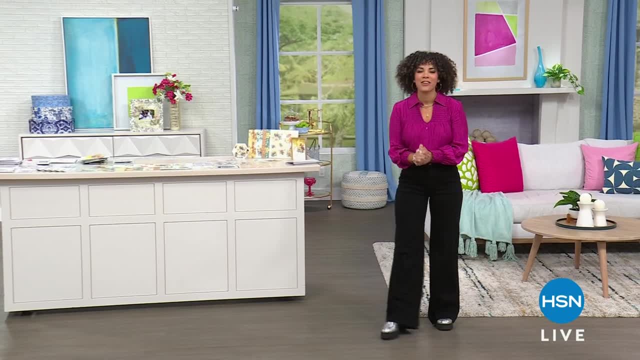 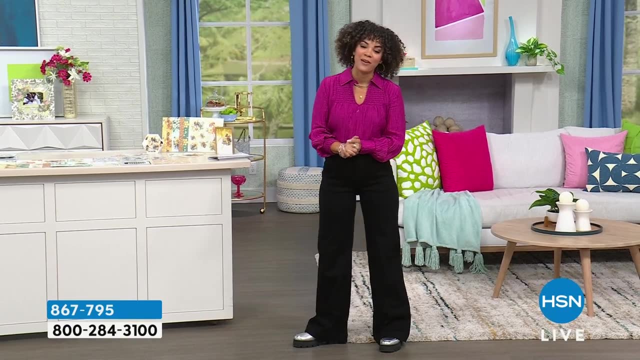 Hi everyone, Welcome to HSN on this Monday. My name is Nicole Hickel. It's customer appreciation month all along in April and today is our crafters appreciation sale, so we're so excited to be with you. One of the most questions we get asked as hosts is: what are you wearing? So I'm excited to say 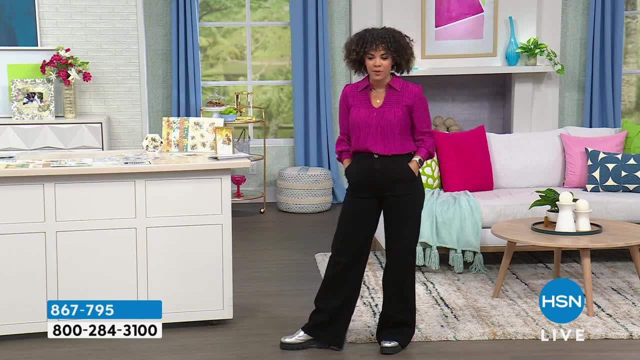 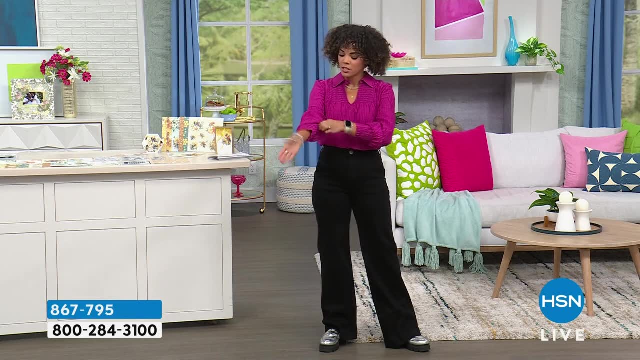 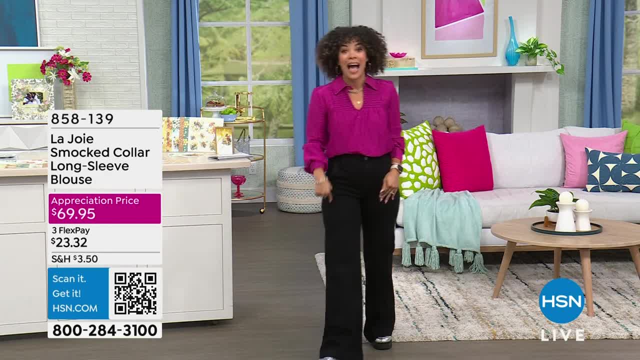 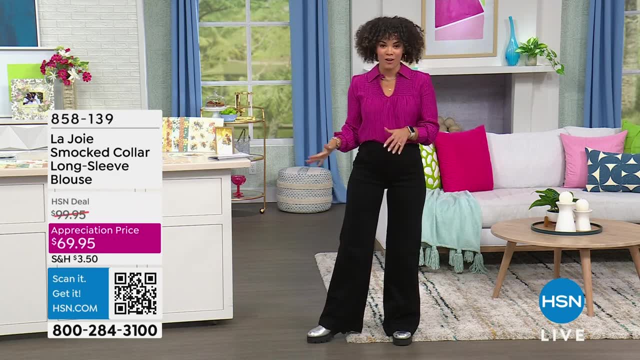 The appreciation price is $69.95.. You know, I found out, my jeans are also $49.. They're also at appreciation price. so you can shop my look by le joie on hsncom. You can always search Host Closet on our website too, and you'll see a breakdown of everything that I wear. 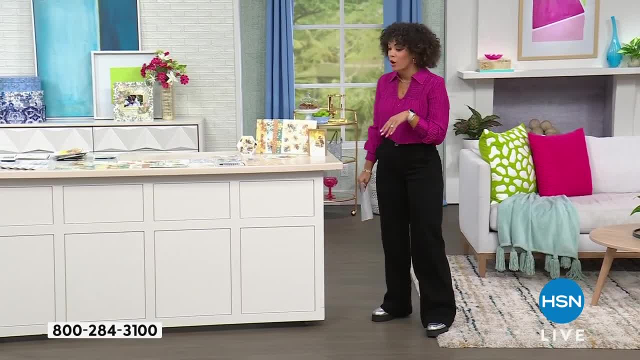 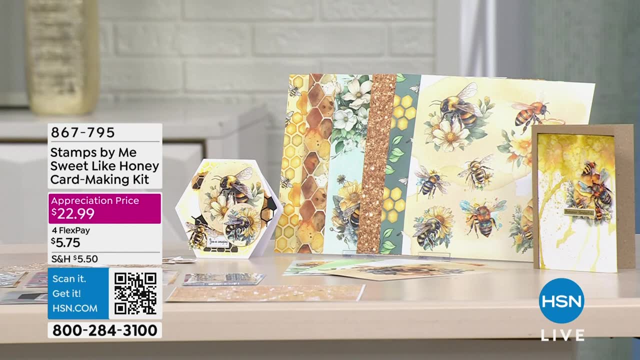 Debbie D wears Natasha, Emily, Tina, all the good things. Okay, are you ready for this? So I said we had something special for you towards the end of the show, featuring stamps by me, brought to us by Tony Darik. So here's the thing. 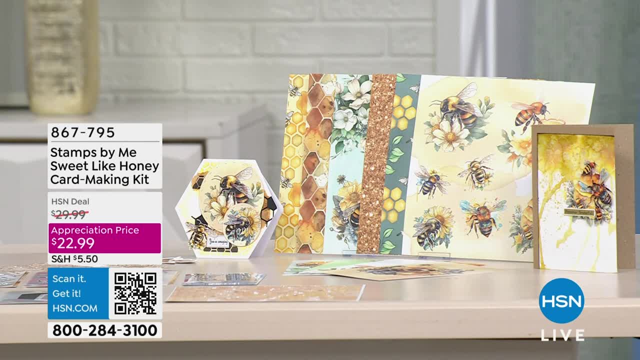 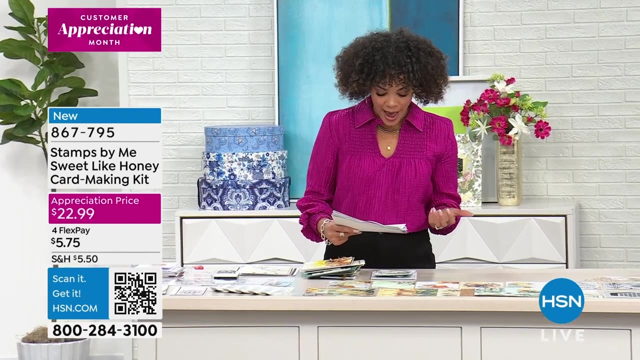 We just got this in and look at the appreciation price at $22 and some change, So you're going to get everything that you need to create these visually stunning cards with the sentiment sheets, the stencils, the sheet paper pads, the stamp sheet. 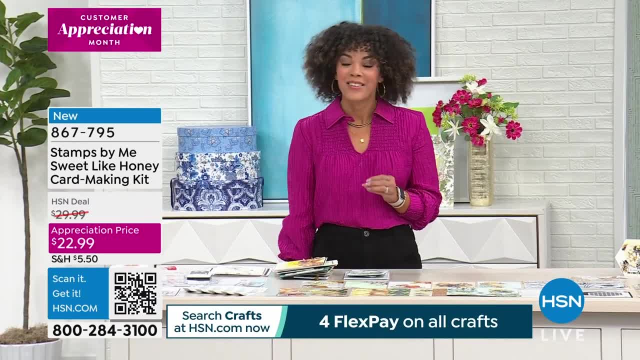 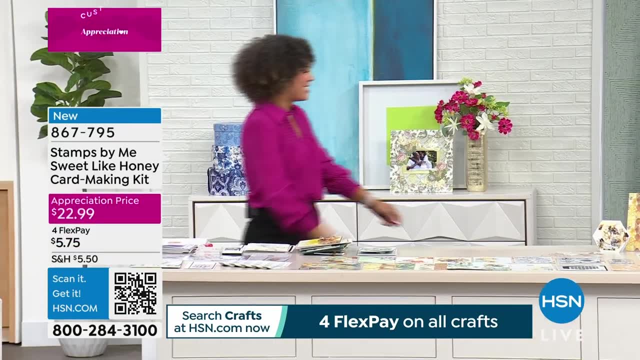 Here's the thing: 780 of these, and then that is it: 867-795. is that item number? Let me introduce you to the beautiful woman behind stamps by me is Tony Darik. So good to see you. Good to see you, Tony. Oh, my goodness. 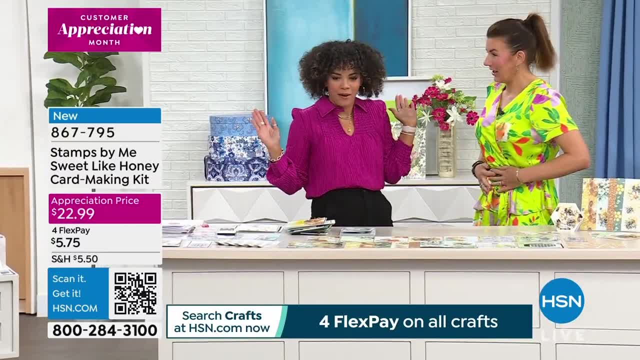 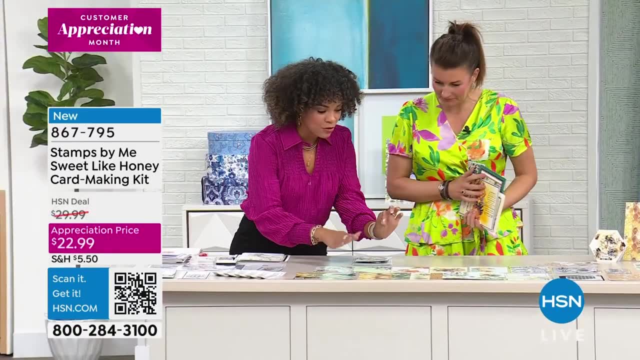 Nice to see you again. Yes, we are. We're springing it up. We're both like very bright, We're very paradise. I love it. Okay, I'm excited about this because this is absolutely gorgeous. Wow, And I said it this morning, the price is correct. 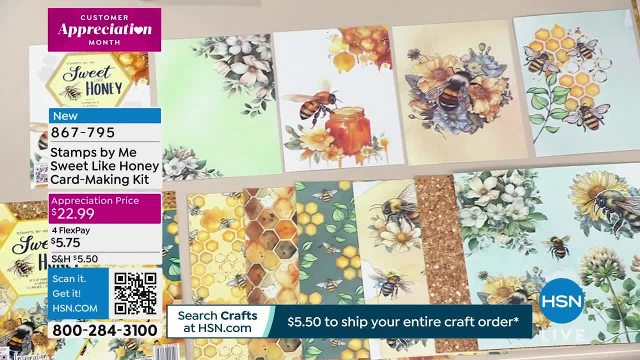 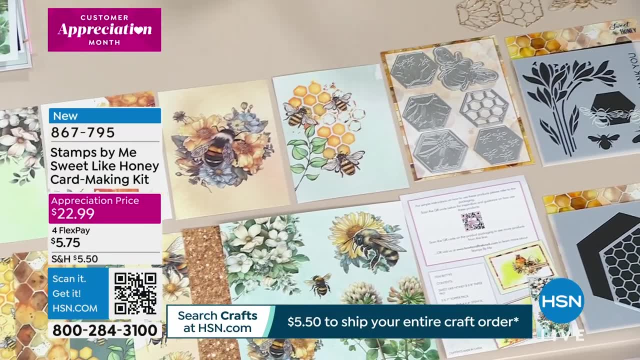 Yeah, I know For what you get. honestly, I was this morning. I was in total shock. I knew the price before I came to her, but my goodness me. So it's a beautiful eclectic compilation of the bees, the honey, the honeycomb, and it's a kit. 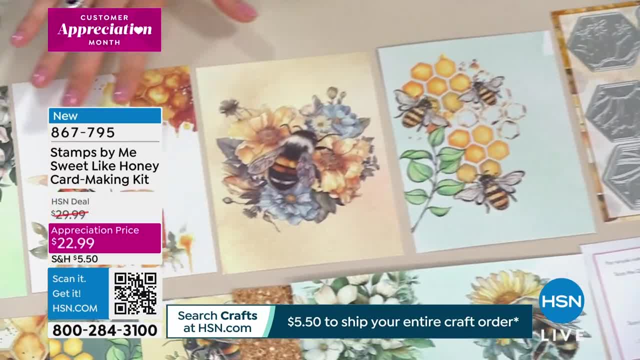 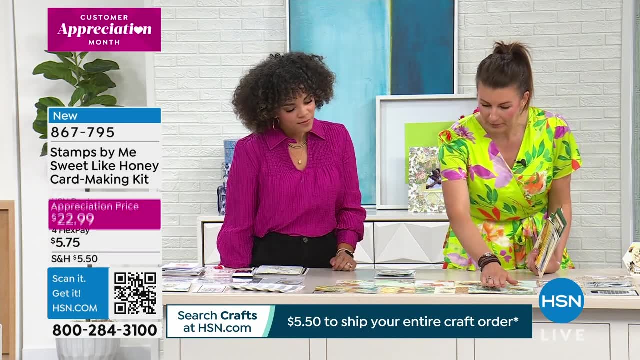 That 50% of it is going to be consumable. so you can use it on paper wise and your toppers, but the rest of it you can use for the rest of your crafty days. So you have a whole bunch of papers down by here. Then you have your pre-painted mounts here where you just have 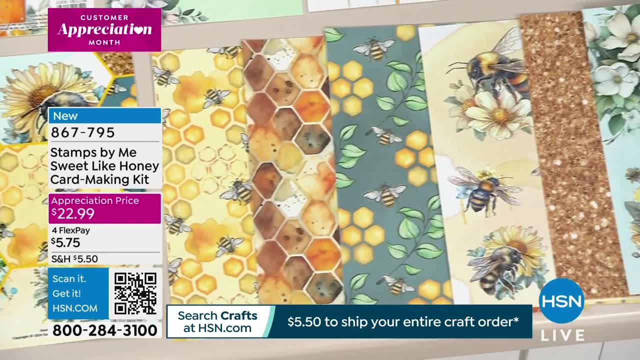 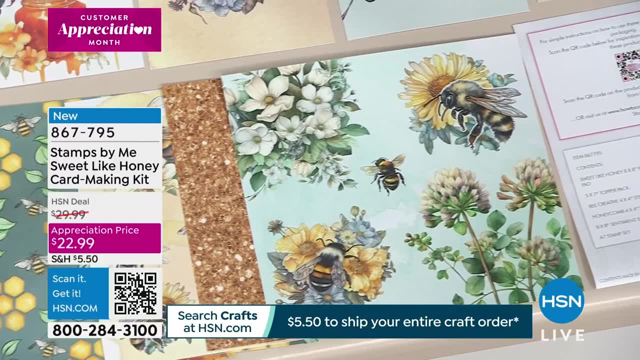 to have a sentiment. if you want to, Then we have our wonderful patchwork die set here, Absolutely stunning. These are going to show you how you can take your craft to that next level. So let me show you these patchwork dies here. 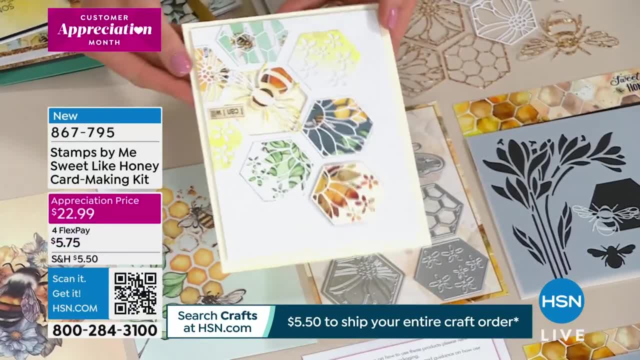 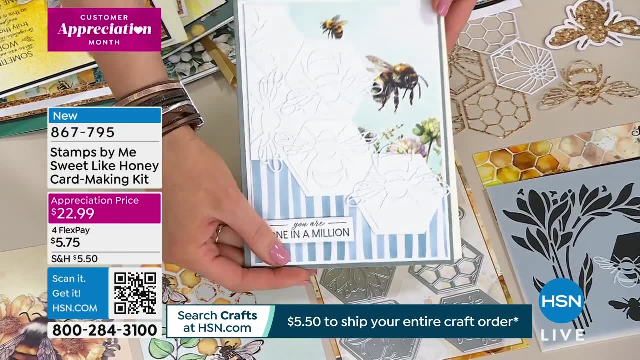 So when you build them in and you put the layers underneath, look at how you connect it and make a wonderful- if you want to patchwork quilt or if you want to do a connecting design where you put the layers on top and build it in with the papers In the set, you also 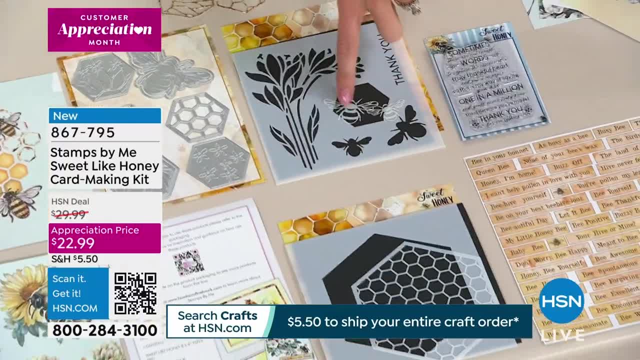 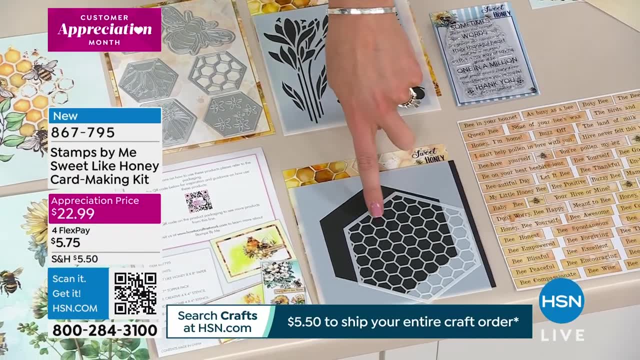 get your two stencils which have the masks as well. So you have the little buzzy bees. so you can stencil through these if you want to. You have the floral designs. you have the hexagons which go behind the dies. Then we have the hexagon, sort of honeycomb design. 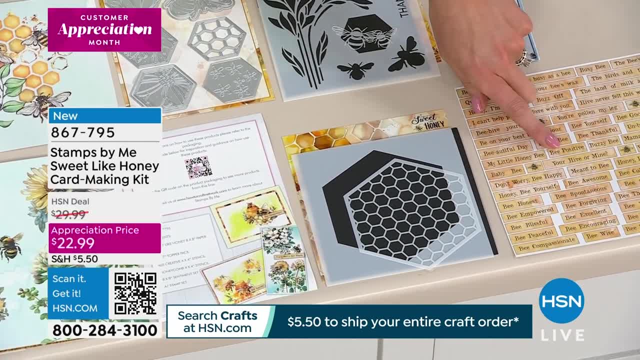 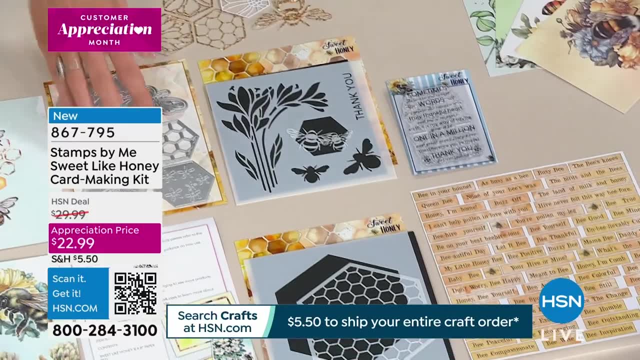 the interior and the exterior. Then we have a whole bunch of words here. There are over 100 elements in this particular kit. Wow, for $22.. I know, and the die is worth that on its own, I know. So this one, I was horrified, but it's. 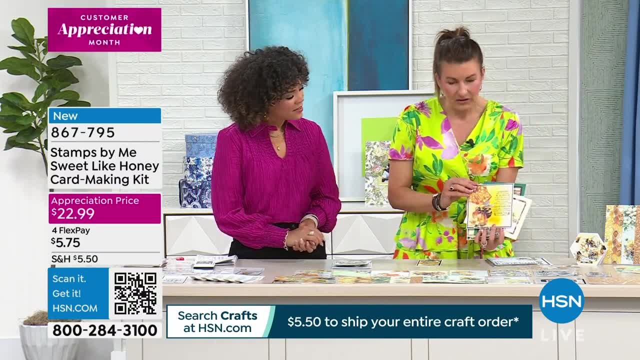 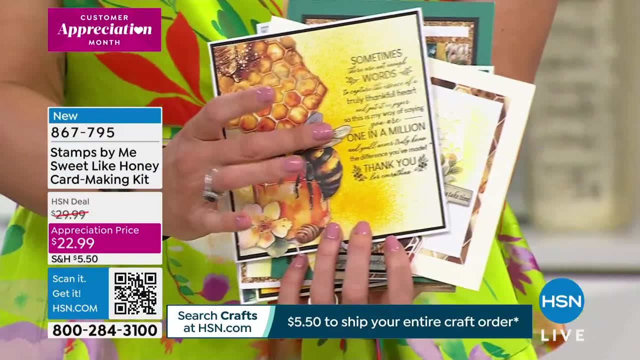 brilliant for you guys at home, because it's giving back to our wonderful customers, isn't it? So let's just show you some of the wonderful samples. Oh, I've missed it as well: The stamp, the sentiment stamp. So you get this beautiful and I'll read it in a second, but I'll just 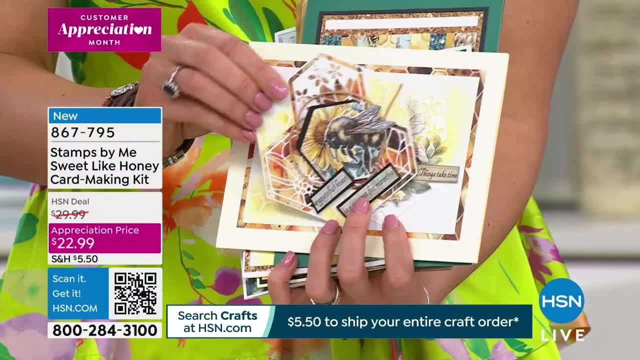 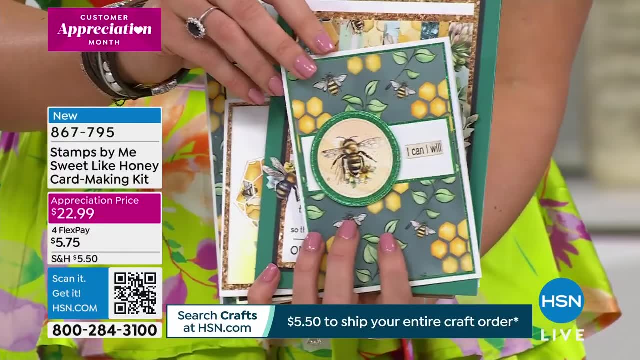 show you some of these wonderful samples that just evolve. So this is the stamp that you get to evoke spring. They can go into summer too. You can build the elements together, fussy, cut the elements and you can see the threads of teals. 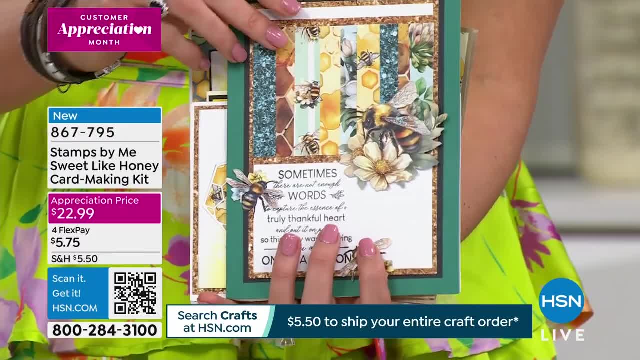 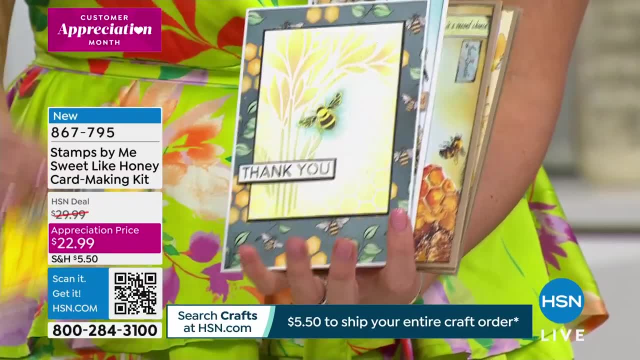 and the light blues running through there just to change it up a little bit here, make it a little bit different, because although there are tones of yellow and gold, it's always nice to have like a breaker color in there, just to break those designs up and make them. 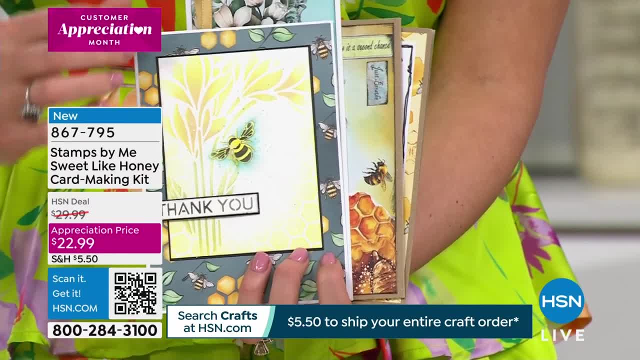 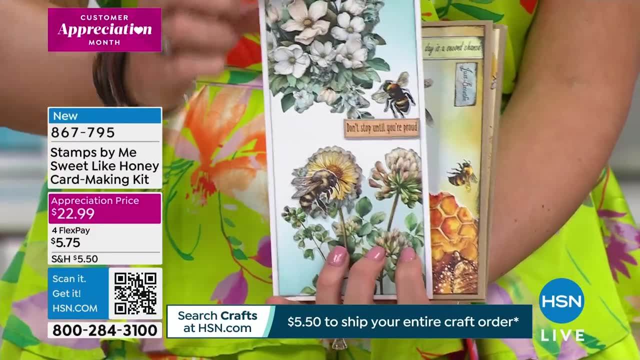 a little bit different, And here we can see that wonderful stencil, the buzzy bee stencil too as well. But the hero product is absolutely this patchwork quilt here with the designs that interchange. They're such sophisticated cards. as I look at them I mean wow. 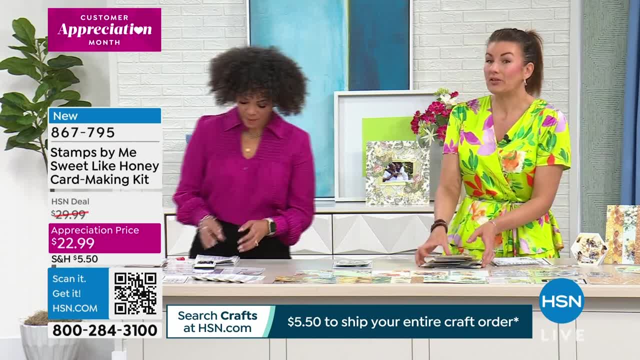 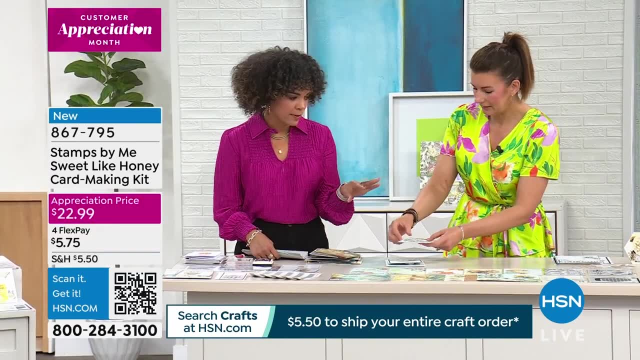 They are really, really pretty. So shall we do a little bit of demonstration, because I always have a ton of demos? Oh, absolutely, I love it And I love that you're already set up for success. You get all these pieces that you're seeing, with the sentiment, with the dies that are included with the paper. 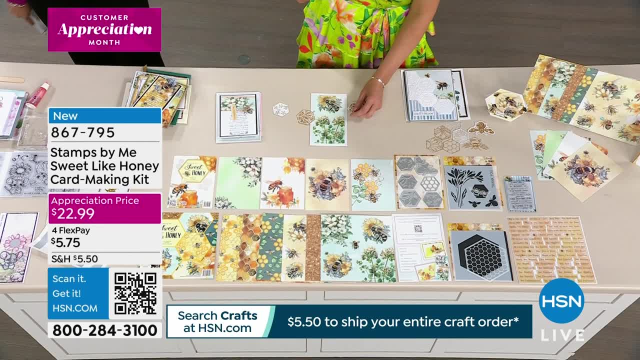 that you're getting at $22 and some change, So it's brand new for you. As you're watching a Tony, feel free to jump in at any moment on hsncom, your HSN app. key in that. I'm number 867799.. 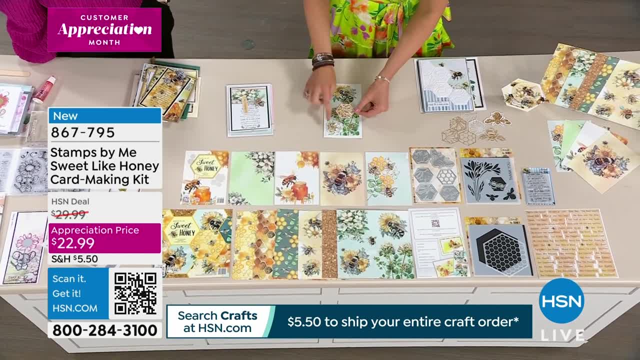 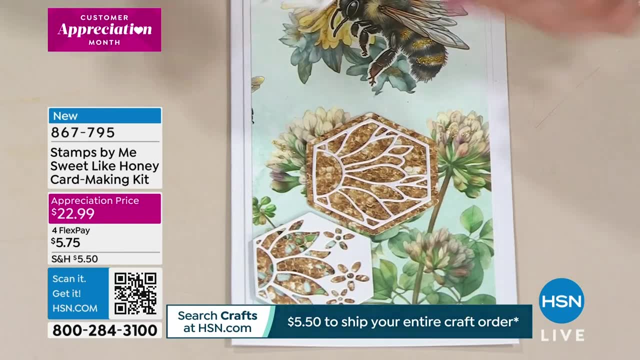 So, ahead of time, I've cut some of the lovely patchwork hexagons with all the detail behind with the coordinating papers, and I've just put some pattern paper on the back here. I'm not going to stick it in place because there's so much I want to show you, but you can see. 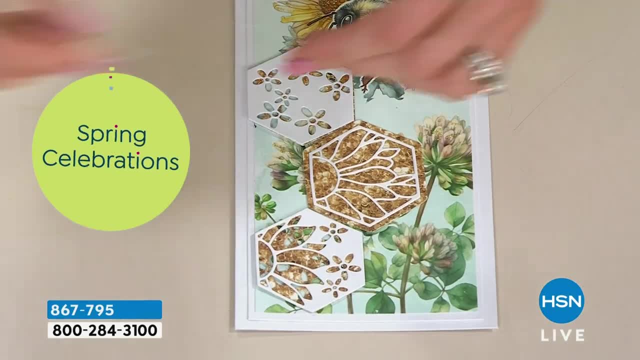 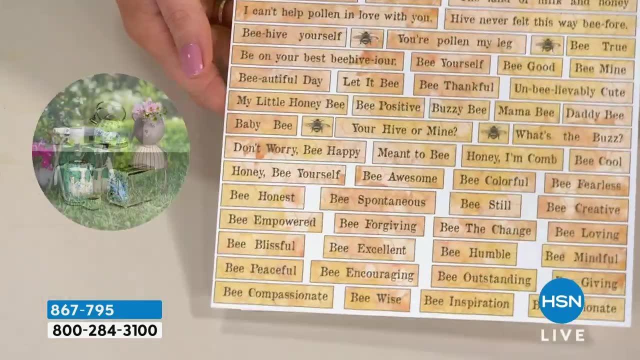 how you can build the design up and across the page if you want to. Then you just cut one of the sentiments away which come from this incredible sheet here. Look at all of these wonderful sentiments here. So you can just take away some of the sentiments. There's some bees in there too. 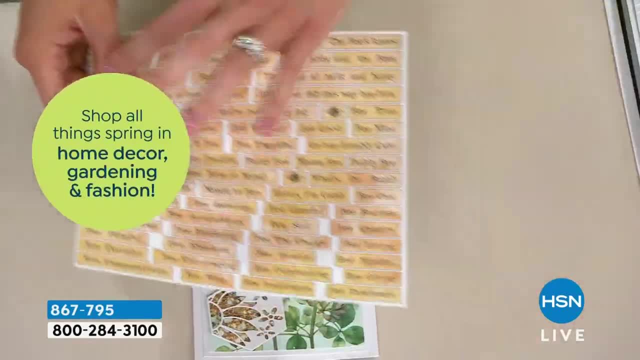 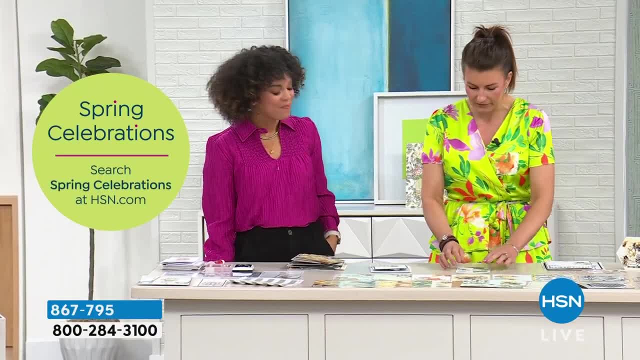 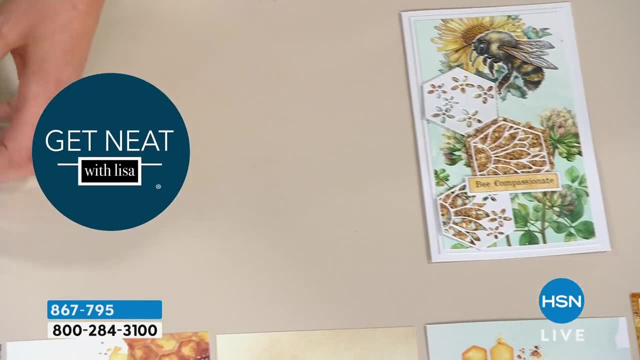 Yeah, Which is so Stamps by me. We just love positive in our creativity and our card making, So that's just one card we have there: Be compassionate. So that's one Let's move over. Let me just read this wonderful stamp set to you as well, because I think it's really important that. 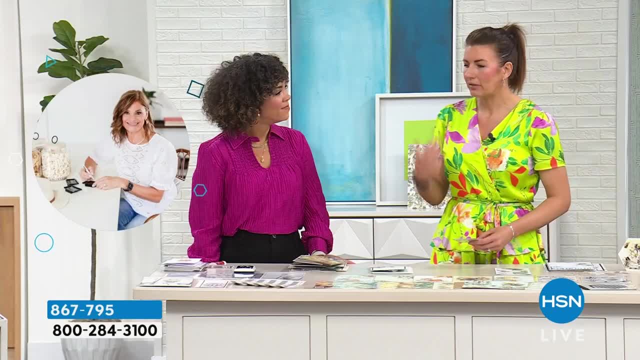 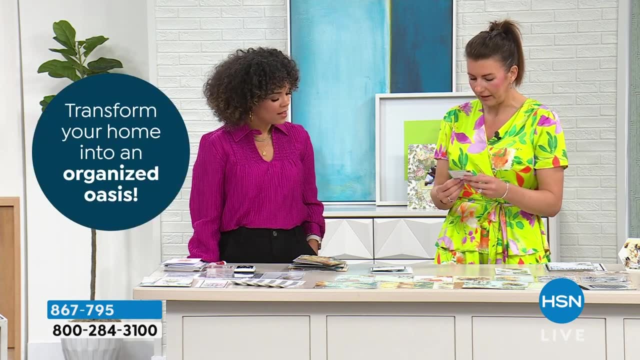 you understand the lovely collection and how it evokes, like crafting, community thankfulness, friendship. So sometimes there are not enough words to capture the essence of a truly thankful heart and put it on paper. So this is my way of saying: you are one in a million and you'll. 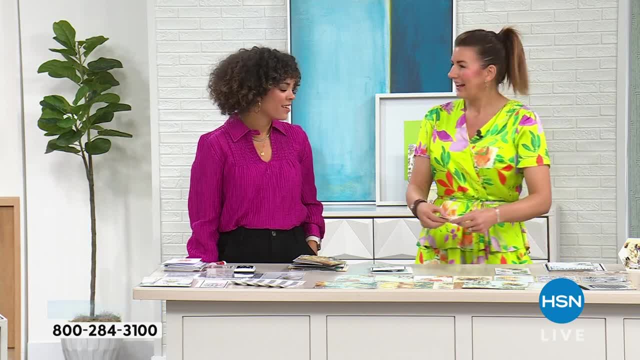 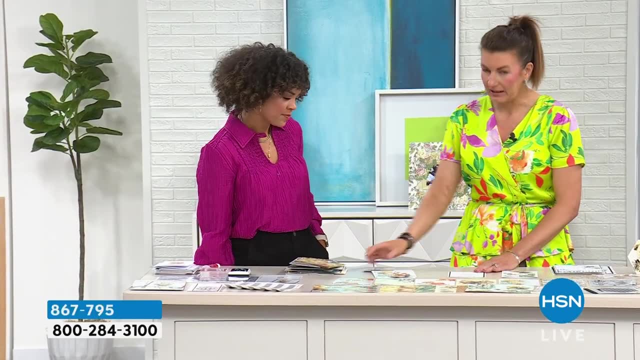 never truly know the difference you made. thank you for everything, oh my goodness. and that's inside, so you can pop that inside or exterior. so here we go. wow, here is one that was stamped at the bottom here and i just have some off cuts, so i'm just going to pop some off cut paper there and one. 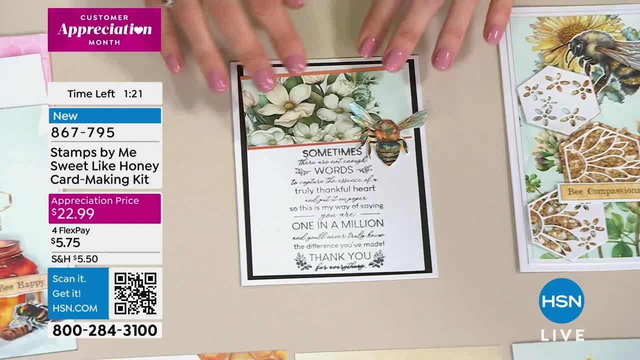 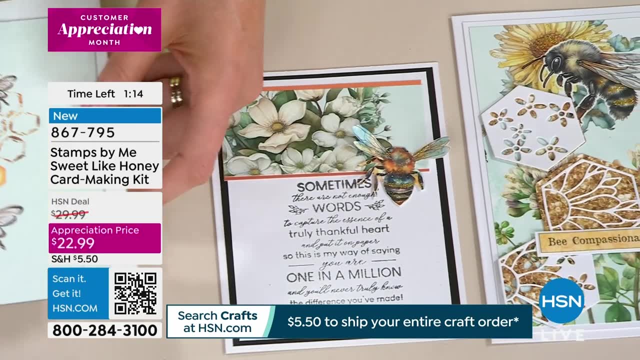 of the buzzy bees that i've just added some sparkle onto there. i'm just going to pop that up there. so we've got two cards already. you can see how the designs just simply work together without any force or any problems. so we have our painted mount again. i just added some sparkle. 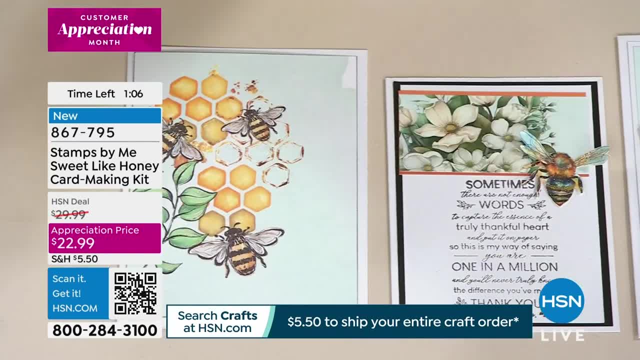 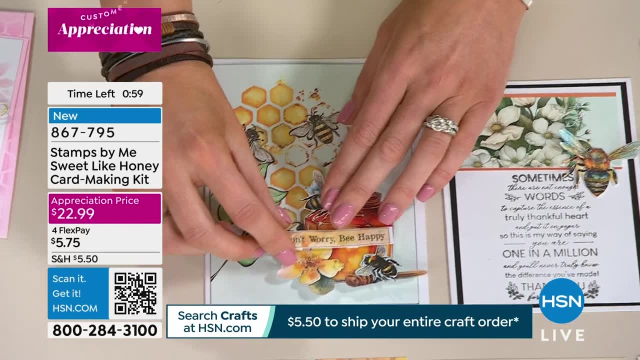 so we've just got- and these are the pre-printed mounts in here- and we have that fantastic qr code on all of our packaging. just scan that qr code. it takes you to all the information and all of the inspiration for all of the items that we use in the show. so you don't have to go hunting around. 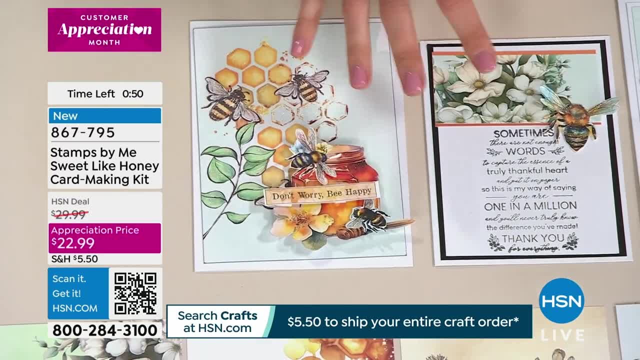 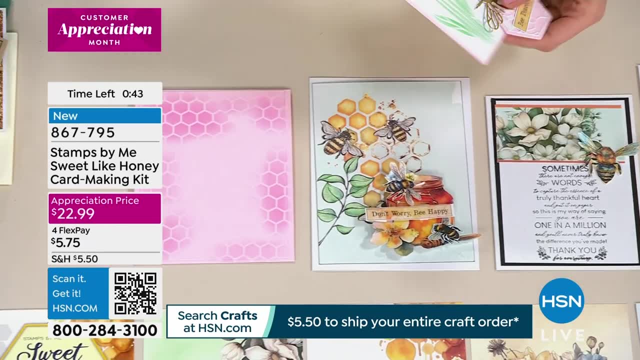 so we've done three cards there, all particularly teal and um sort of orange in design. let's show you, let's change it up now. so here we have a pink one, we have the lovely stencil honeycomb design. yeah, then we have that beautiful flower which is: 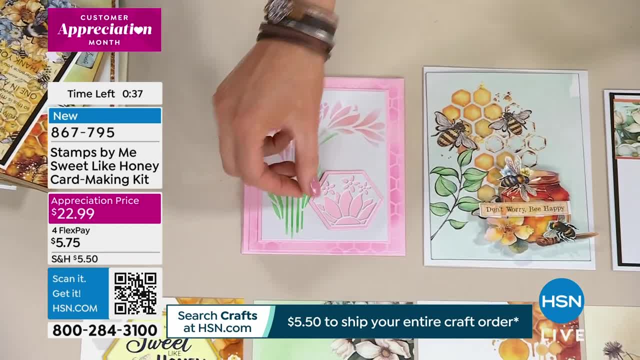 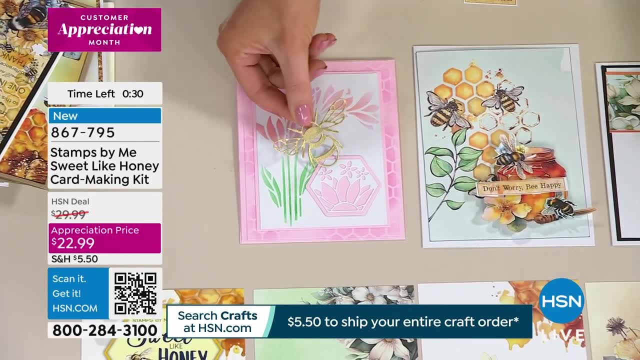 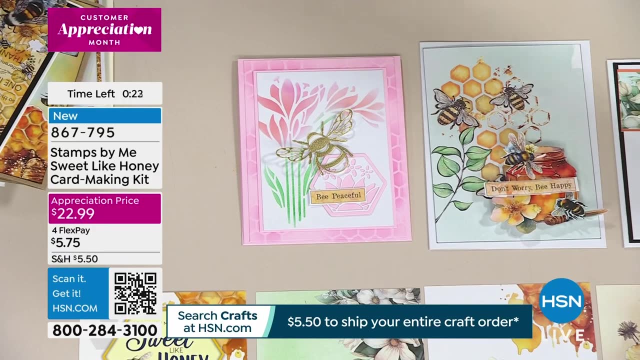 stenciled through with some ink there. then we have our pink sort of hexagon design here, a cute bee, because there is a huge bee in this lovely die set too. we'll pop him on there, like so, and we'll put be peaceful on here too, and i'll just show you that lovely dice. i'll just move this out of the. 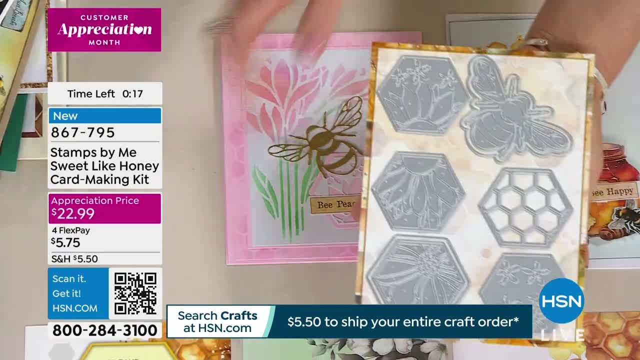 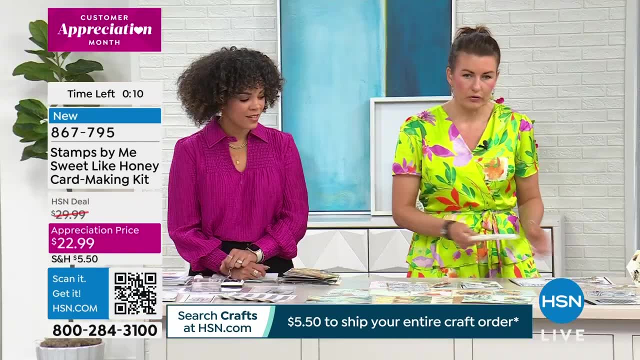 way very quickly just to show you how wonderful this dice is. it's a big die. so you can see by the hand there and you can see it's a big die. so you can see it's a big die. so you can see this is a big然后把他拢进去更多面颜的隙. 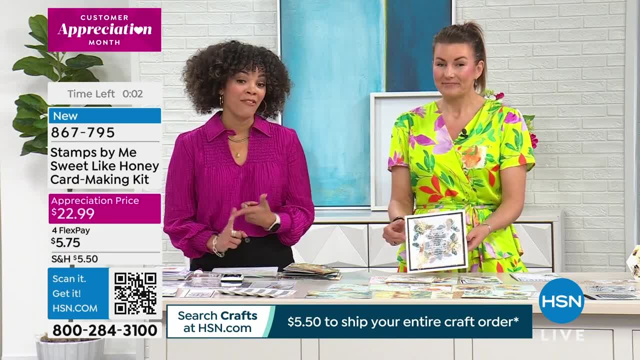 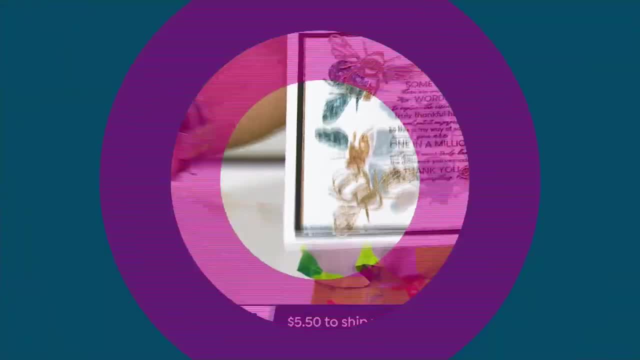 if you want to, gorgeous, here's the thing: vinyl 400 left and then that is it. so if you're kind to let it sit in your cart and you're like, well, i need to load up my cart and, for the 550 shipping, go ahead and check out. load up your cart, check out and you can add things throughout the day. 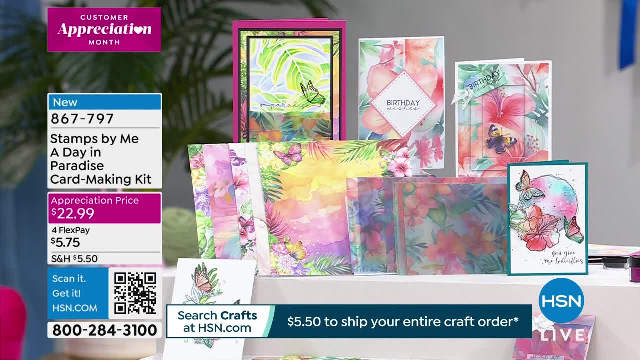 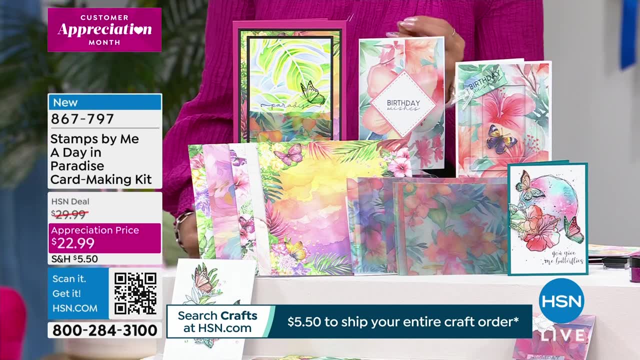 because all today your shipping is just 550, so you can check out several times, which is really great. okay, i'm exciting about this: now very limited, like we saw with the um, the bees, with the final 400, and that we only brought in about a thousand of this paradise card making kit. so this is brand new customer appreciation price at 22. 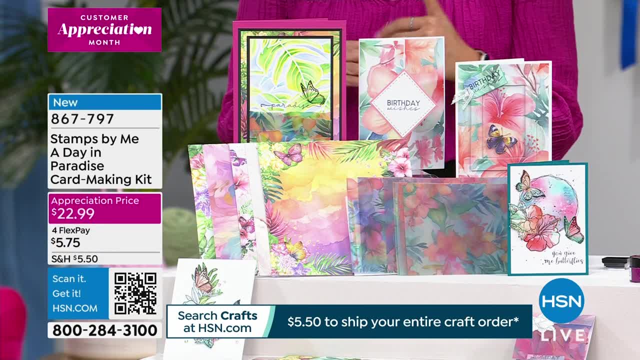 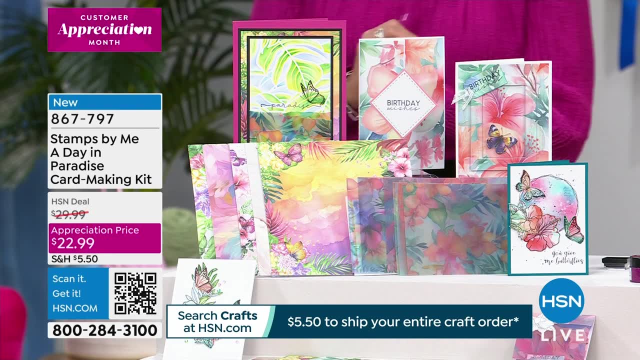 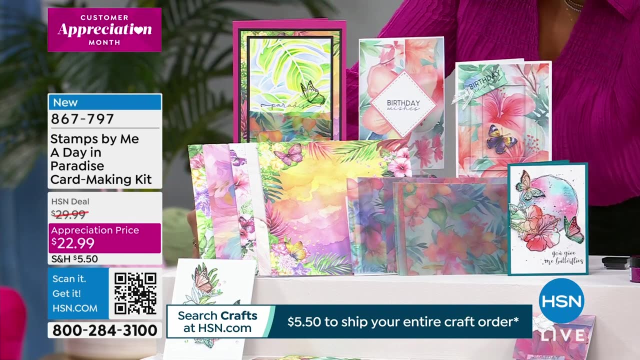 dollars and some change. i love that. you get the stencils that are in there, your vellum pack. you get a pot of paste. um, you get 11 pieces of stamp sets to give you that endless possibilities and really this is just transporting you to that floral paradise. i mean, wow, oh, my god, look at this. 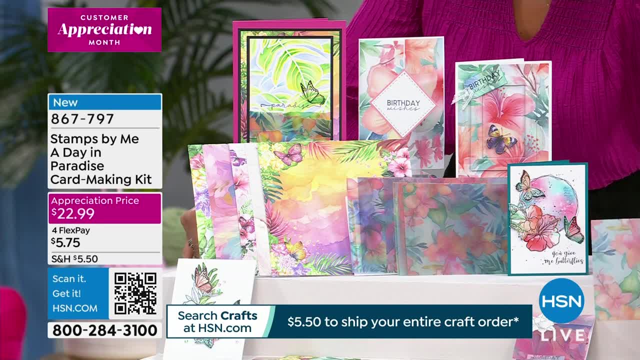 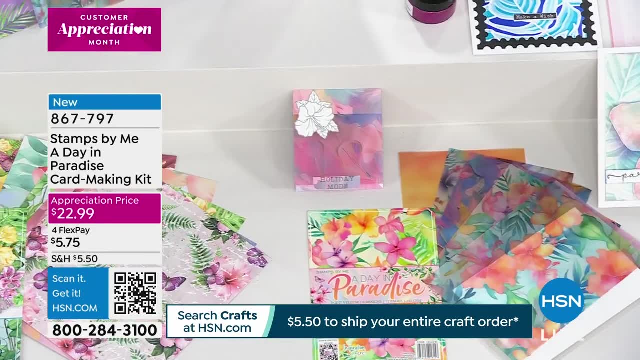 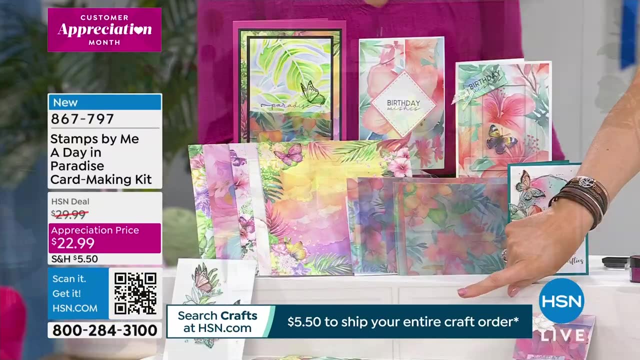 vellum by. oh my, how gorgeous is that. you're never going to see vellum like stamps by me. vellum, it's incredible. it's so luxurious, it scores beautifully, you can stamp onto it. it makes beautiful envelopes. so the kit contains 44 items. it has another paper pad for you here with the eight by eight designs. 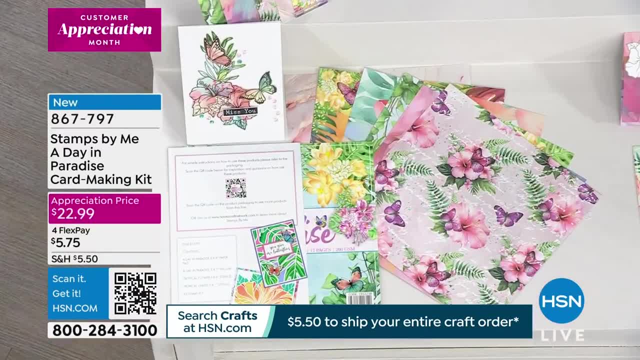 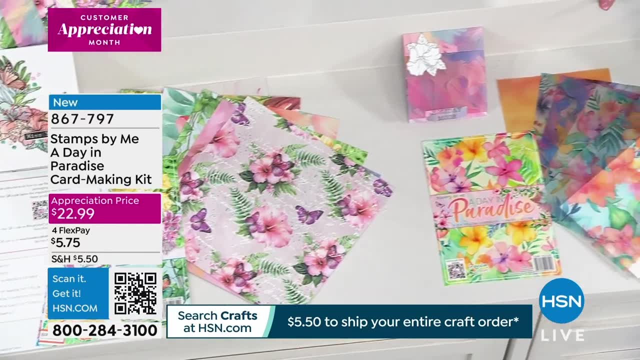 which you can cut down. you have two of each design. then we have the vellum again. you're probably not going to use this, you're just going to stroke it and look at it. it's too nice to cut into. i tell everybody to cut into it, but honestly, 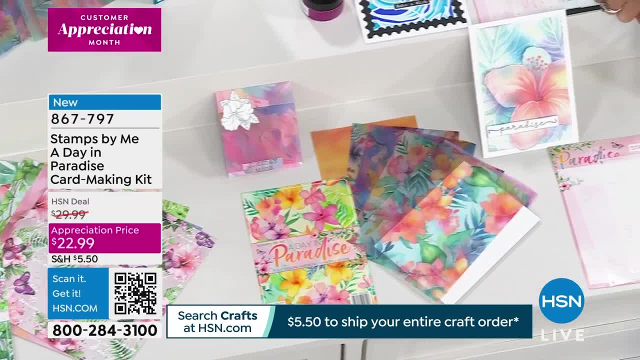 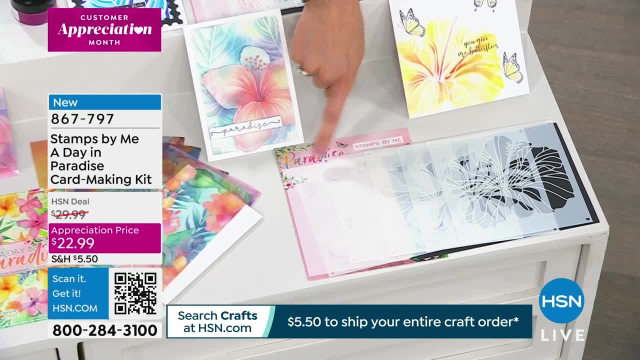 uh, you're the people save it. and then, moving across here, we have the five stencil layering system, which has the heart technology on all four corners, and you pop some ink through the hearts. they are numbered one to five and you just line up the system and you are able to create the most. 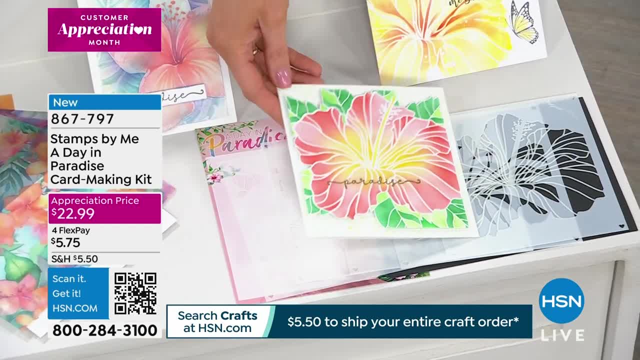 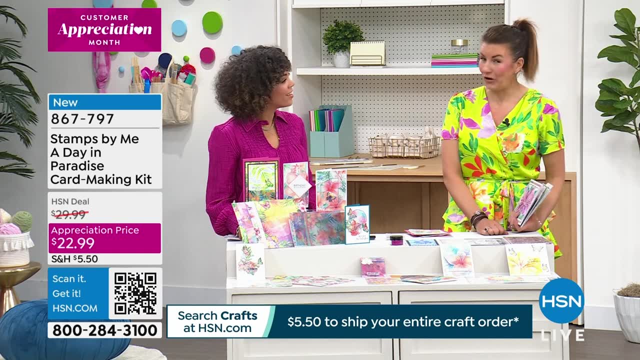 wonderful 3d dimensional florals in there as well. it doesn't end there. if we just move up slightly, we have a a5 stamp set which, when i say a5, half of an a4 sheet of paper. so they are huge and you get the florals, the butterflies, the leaves. 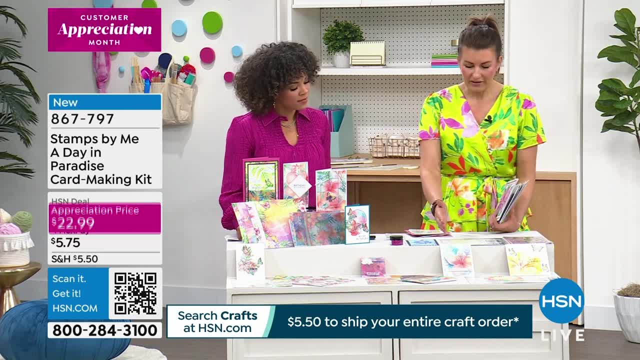 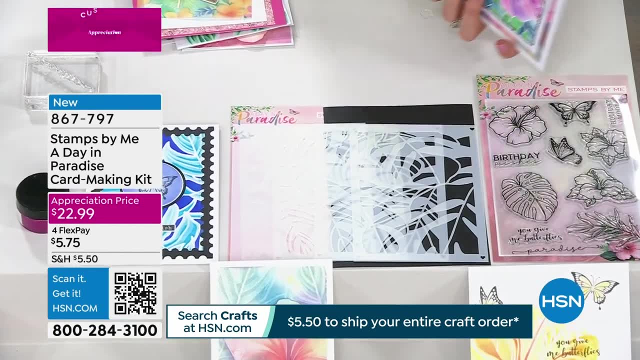 so you can see the size of that one there as well. then, moving over to the side, here we have a four layering stencil system which gives you the lovely greenery which gives you sort of this design here. check this out. so another three-dimensional card which creates beautiful backdrops. for the rest, 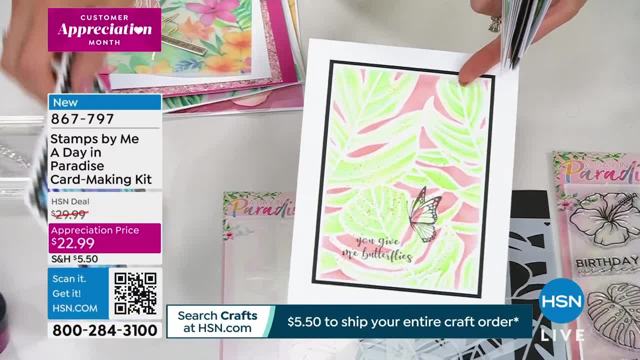 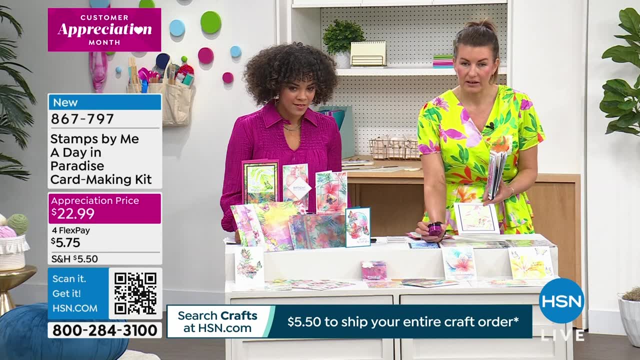 of the collection. so that's in the common theme of our wonderful paradise, but look at this one in the blues as well, so you can see that incredible dimension. then, moving across, you also get a pot of translucent gel paste. i love that, which is wonderful. i'm going to show you how to do that in just a moment. 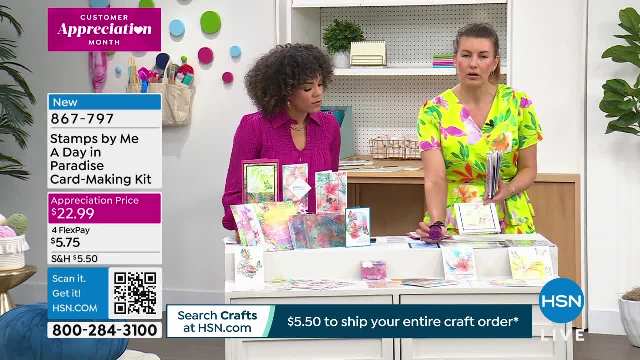 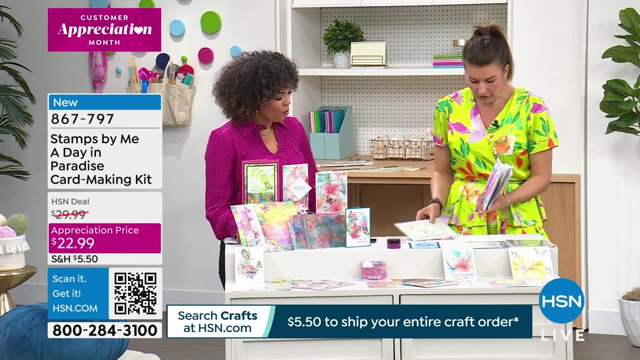 so you can see that it's a very beautiful color. it's not a full coverage paste, don't get confused. it covers over the ink and the ink that is underneath shines, so you get the sparkle on top of as well. so i'll just show you a handful of the samples here. 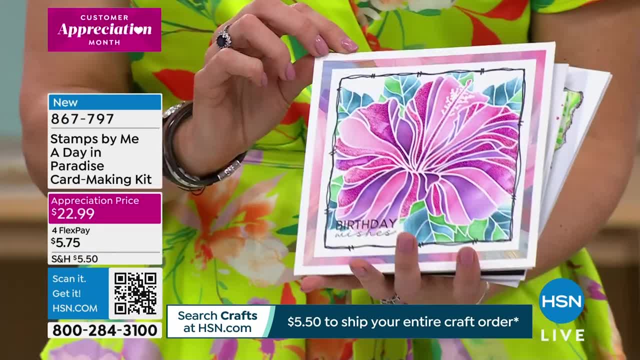 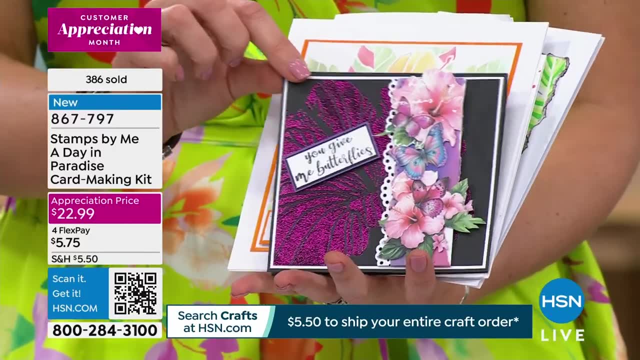 so we have these here with the sparkle on one of the stencils, layered sense, so you can see that shimmer come through on that pink there. all different color waves, so all you need to worry about is what color are you going to choose? that is, to make your own beautiful cards. the paper. 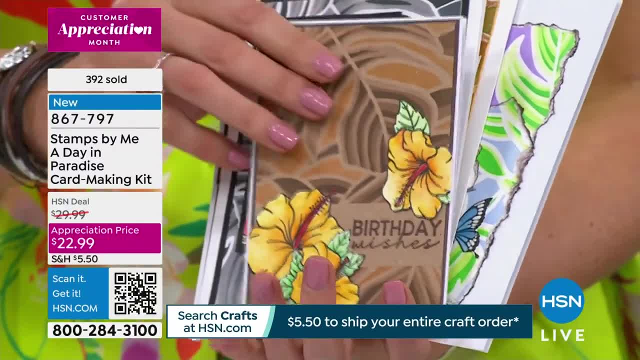 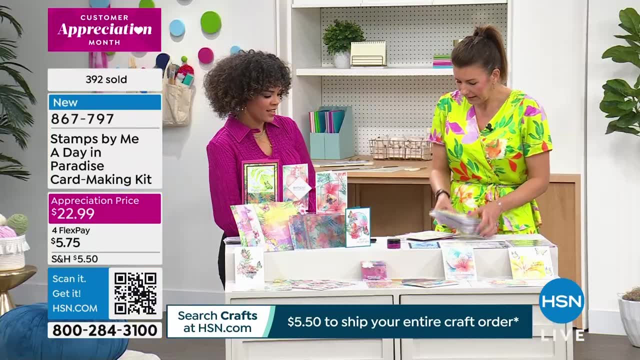 itself, but having the layering stencil system and the stamp kit to enable you to take longevity in your craft. look at that one with the black and white on there. so shall we do a little bit of card making, because i love card making. if you haven't absolutely come with a ton of demos, i've 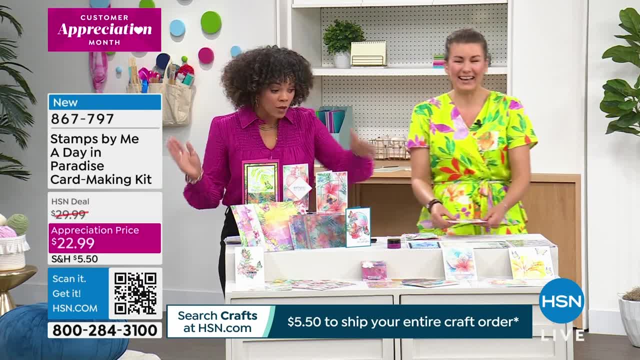 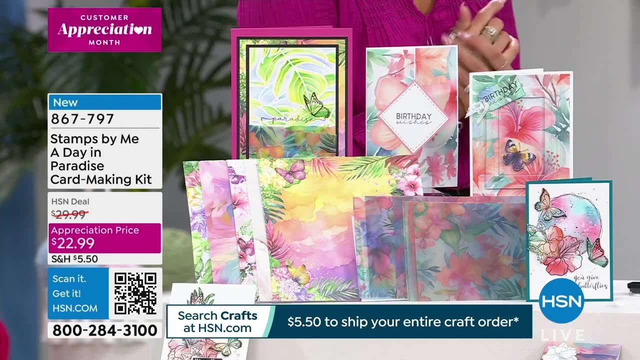 only got eight minutes so and a whole kit for 22. i mean, this is, this is a wow moment, jumping at any moment. i know a lot of you are picking this up. only a few hundred, that's it, less than a thousand. so here we have. let's have a look at this wonderful vellum. so we've got a card, we have some paper from. 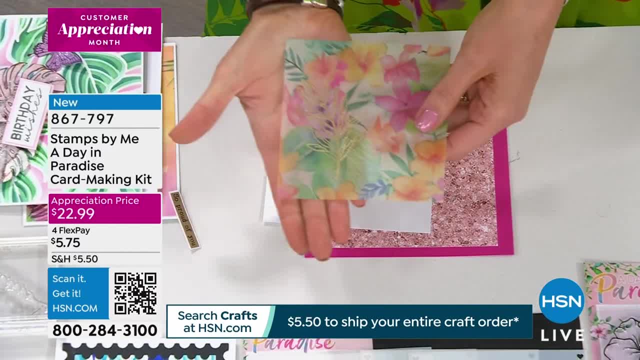 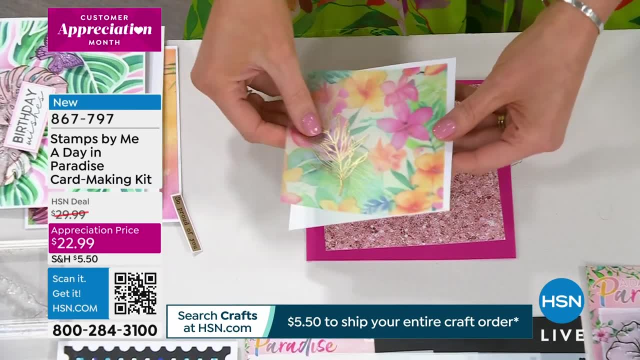 i've got a piece of white. now. this is what we were saying about the vellum i heat, embossed one of those beautiful gold leaf effects from the um stamp set, and then, when you pop it on the white, look what happens, how it just comes to life. boom, just like that, like my dress, right, yes, oh, crikey. 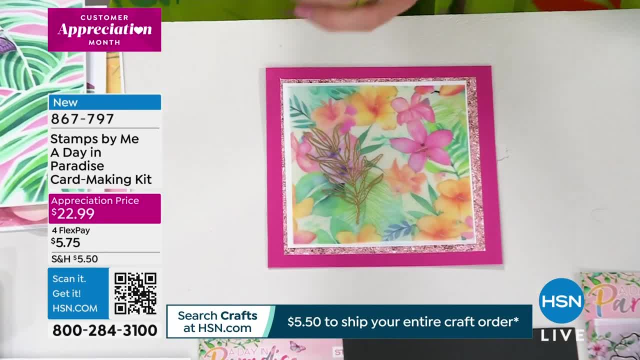 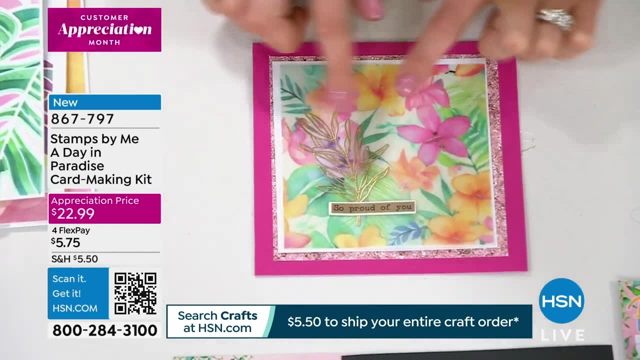 i'd they're all. i was coming down the corridor like my goodness me, we are never going to miss you so and then we've just got a cute sentiment, so proud of you. so that's just sort of like using the vellum and to hide your makings underneath the vellum. just add a tape, pen and you're. 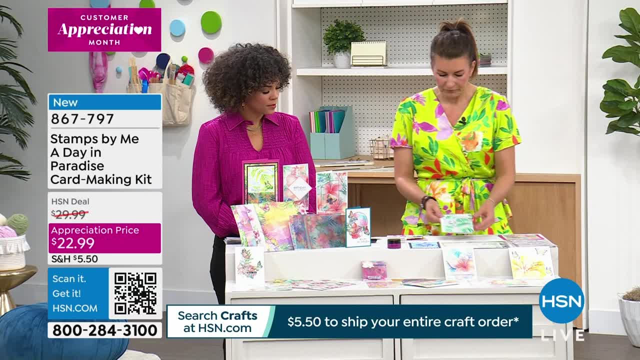 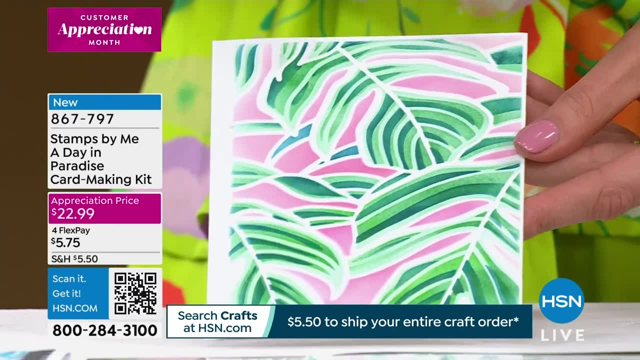 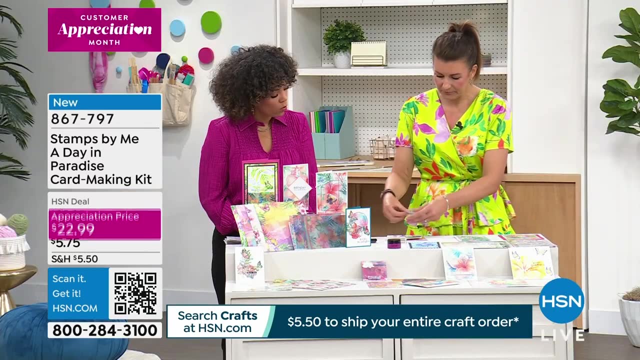 you can't see through the vellum. and then we have our wonderful um three-dimensional leaf stencil system. look at the dimension. there is no coloring, no pens, no pencils. just line the hearts up on the stencils in any color you desire and you can create the most beautiful three-dimensional backgrounds. 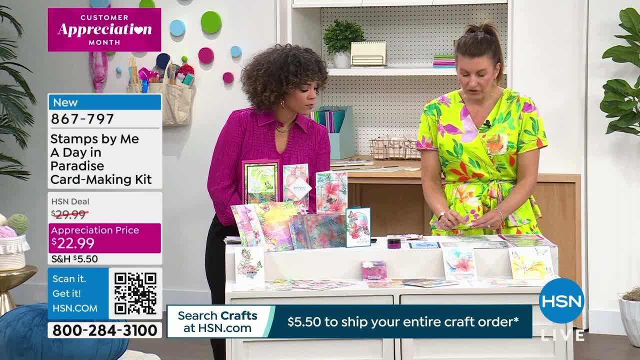 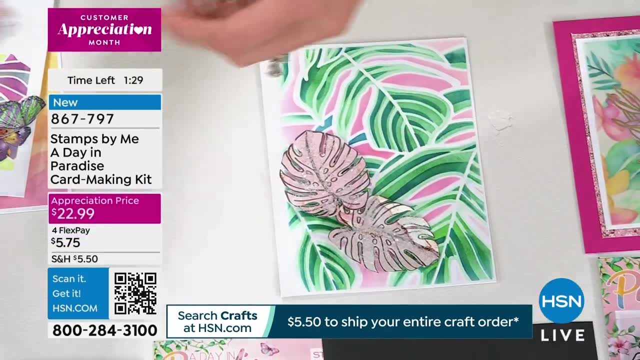 in the kit we also have these like large jungle leaves, but i've done them in pink, stamped them onto the paper, put some sparkle on there too, and let's just add a little bit of dimension in the on top. i'm not sticking anything down because i have tons, as you all know. so that's that one, and 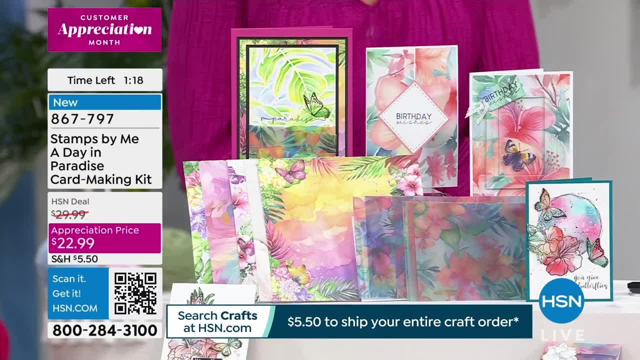 those sentiments are included too, which is great. in the stamps, absolutely everything is included, and i would say 50 of the items are consumable wise. so you'll use the papers, you'll use the vellum, but the rest of it will work alongside any other brand's products as well. so here we have. 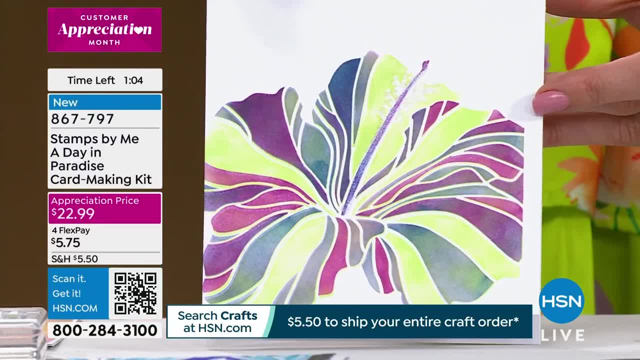 that lovely hibiscus and i just thought you know what. i'm just going to use random colors and see what it comes out like. it actually matches my dress, gorgeous, yes. so we have that one there, and then on the paper we have some cute vellum and then we're going to add a little bit of color to it. so 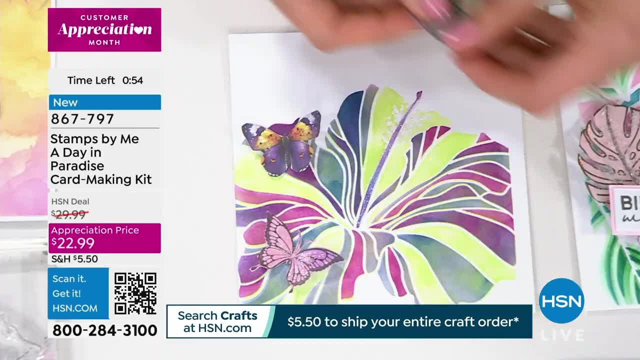 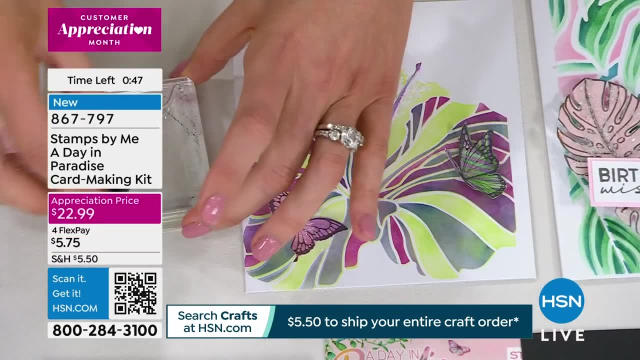 cute butterflies. so let's just pop a few of those on there. i mean, you could pop them wherever you wanted to with a little bit of sparkle. and then i have a stamp from the stamp set, and this is where you can stretch your craft. you can use the stamps in there to create your sentiments and things. 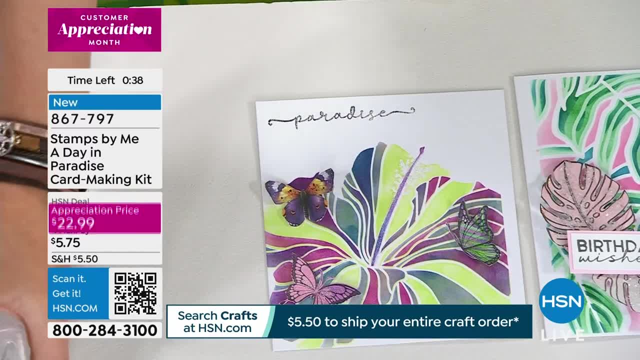 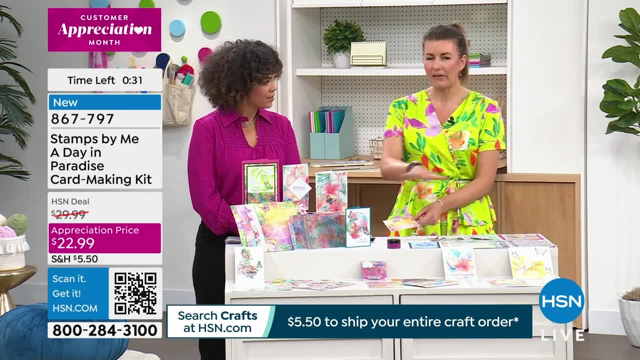 like that. so this one, i'm just stamping positivity at the top there, and then, lastly, the papers just absolutely hold their own. so don't be fearful if you're thinking to yourself. i'm not having a stenciling day today, i'm not having getting out all of my stash, i just want to write. 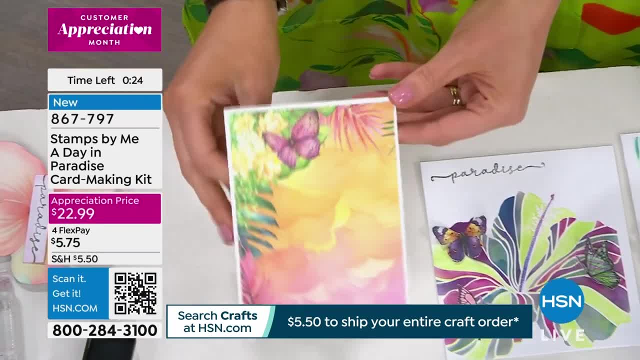 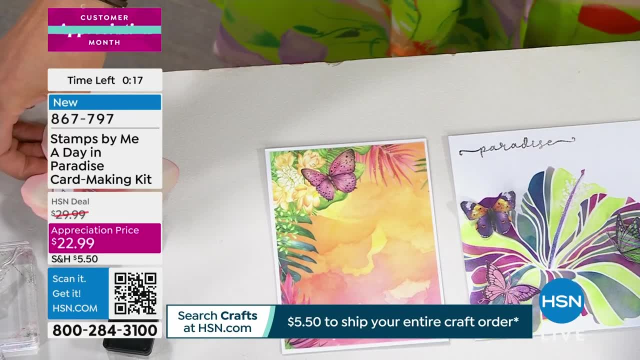 play around with the papers. the work's already done for you on the paper. i love it and, as you can see, it just evokes that tropical sense and very energized, very orange is a very creative color anyway, and it's packed with the color orange and then we have a beautiful flower from 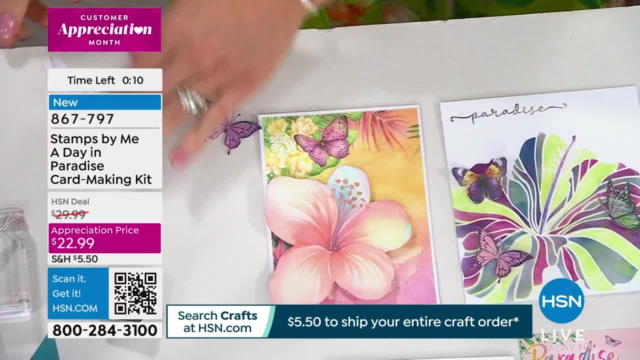 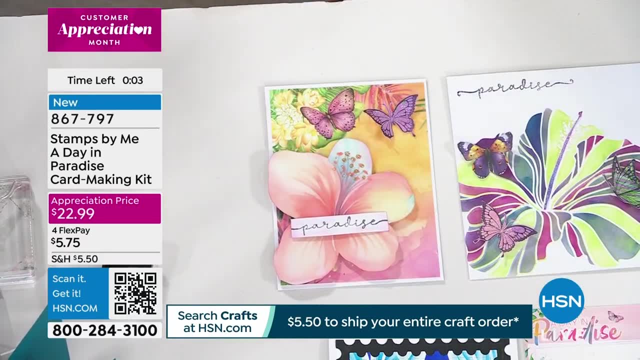 the paper collection. i just cut out there and just pop it on the side. here we have the wonderful um sentiment- positive, because i am a very positive person- and then we have the wonderful butterfly under there and i just very quickly show you some of the lovely samples, with the papers as well. we 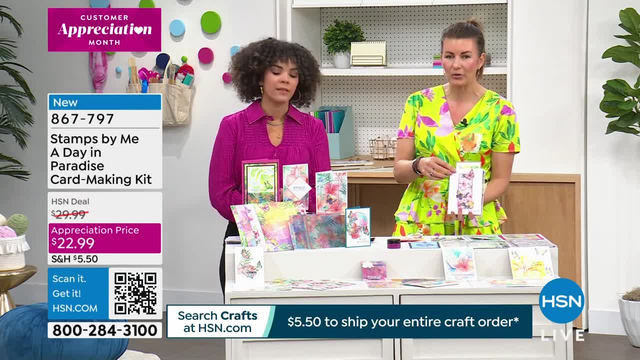 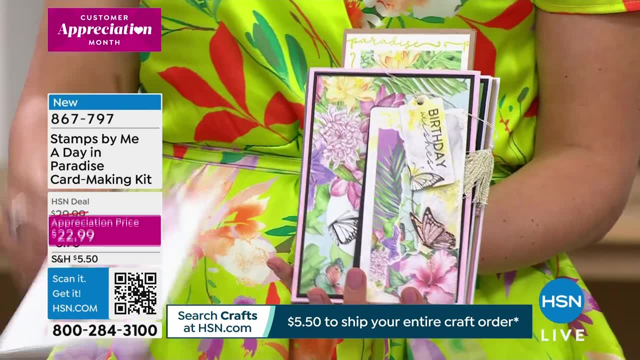 have a qr code for all of the inspiration. don't go hunting. scan the qr code. yeah, take you to all of the inspiration where you can be creative as soon as this item lands on your doorstep. absolutely so many beautiful things. as you take the final moment, remember a customer appreciation price of 22 and